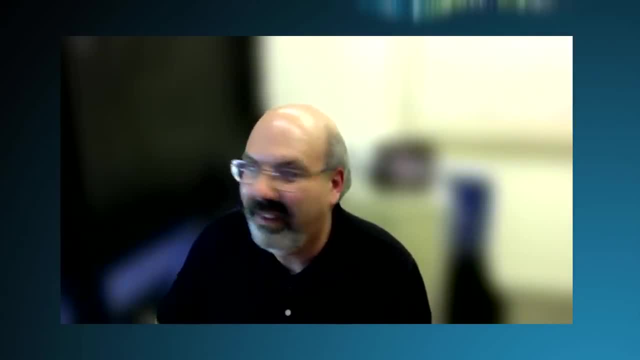 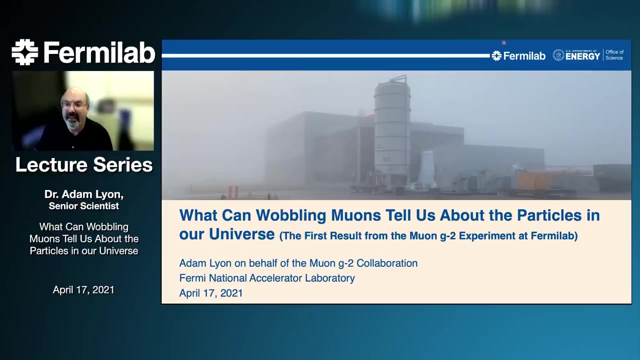 Thank you, Robert Alverson- An introduction, let me get things going here where you can see me and he hear me. okay, Robert Alverson- So, Robert Alverson- Okay, okay, you should be able to see my screen, so let me start that. okay, great, Okay. so thank you, welcome everyone. it is such a pleasure and honor to 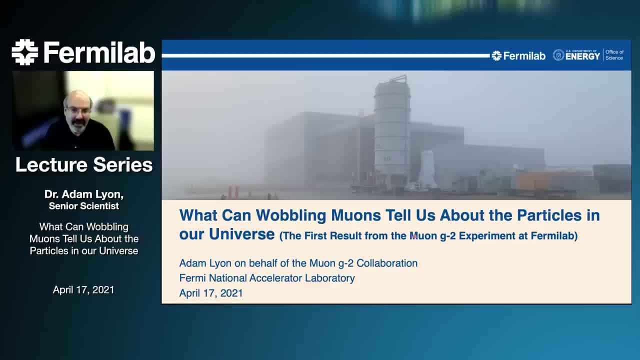 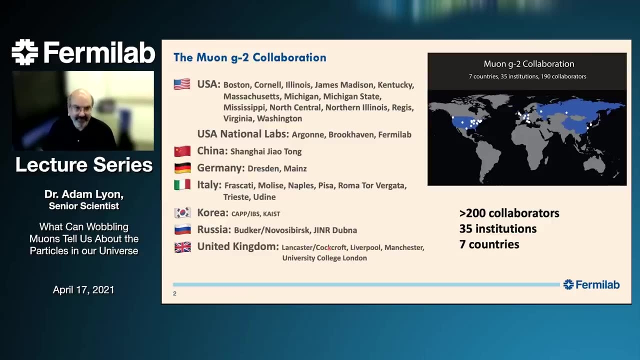 Robert Alverson- To be telling you about the first result from our new on G minus two experiment here, from your lab. or what can wobbly nuance tell us about the particles in our universe, Robert Alverson- So i'm speaking on behalf of the new on G minus two collaboration, let me say, is first for a second, what that means. so 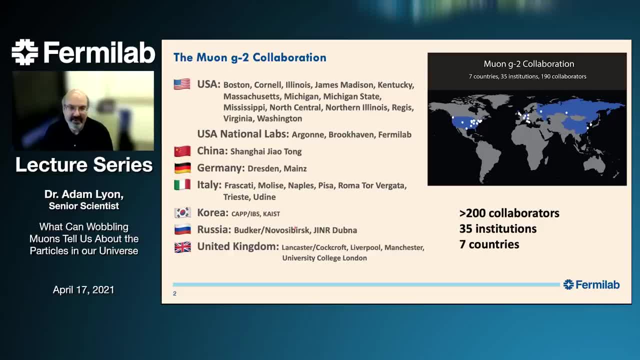 Robert Alverson- The work that i'll be showing is really a work of many, many people. so there are a little over 200 people working on this experiment- Robert Alverson- And Robert Alverson- From 35 institutions and seven countries, from all over the world. you can see on our map, you know, if we want to have a meeting where everyone shows up awake- and that's not an easy thing to do. 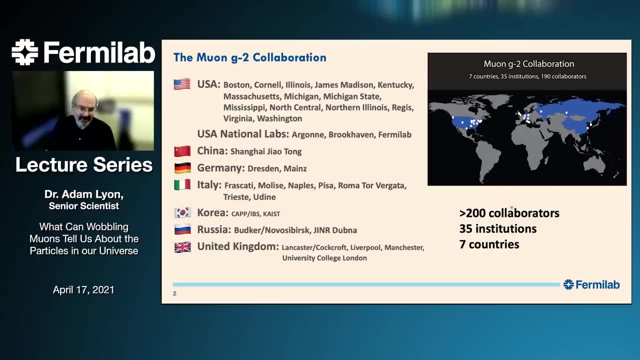 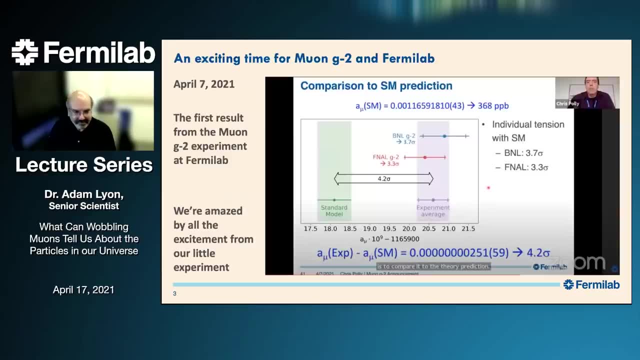 Robert Alverson- And actually I should point out, this is a small collaboration. there are collaborations and particle physics experiments that have thousands of people, so we're we're actually a very small collaboration, Robert Alverson- And as, as as Nigel said, this is a really exciting time for me- one two minus two, and for me, loud, about two weeks ago. 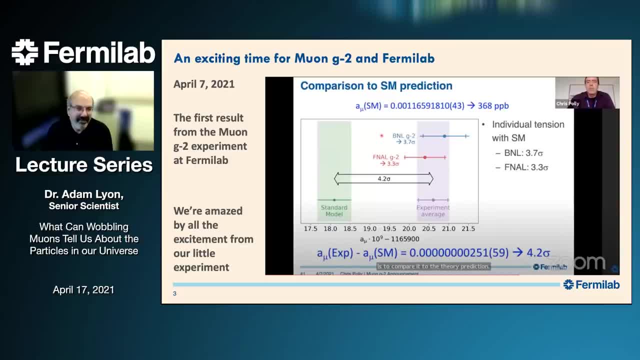 Robert Alverson- One of our spokespersons, Chris polly, presented the first result from our new on G minus two experiment and that's what i'll be talking about tonight, Robert Alverson- And hopefully some of you got to see that- that science seminar. so i'll give you some of the background behind this and, as Nigel said, we're just amazed by all the excitement from our, our little experiment. 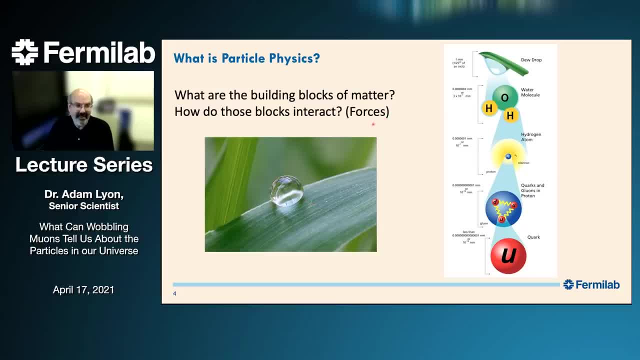 Robert Alverson- So I have to start at the beginning and and tell you a little bit about what particle physics is and how it works. so the question, Robert Alverson- Questions are really trying to answer- are: what are the building blocks of matter? what, what's the universe made out of, at the smallest scale scale, and out of those building blocks interact, what are the forces that that go between them? 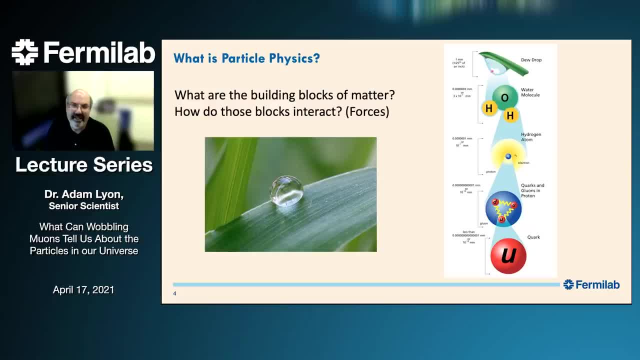 Robert Alverson-. So you know, we start with kind of a standard picture of something you know, like a dewdrop of water that contains water molecules. the water molecules have atoms, right, and the atoms have electrons and protons and also neutrons, Robert Alverson- And? and for a long time that we thought that was the story. 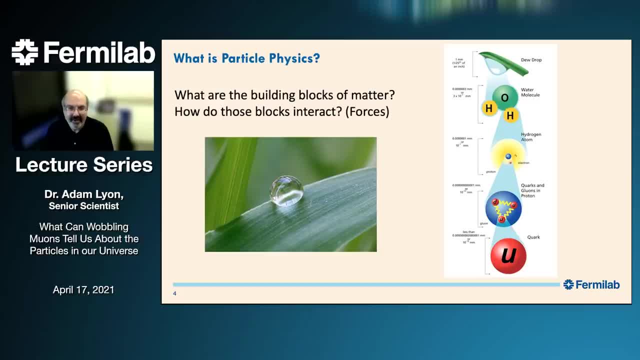 Robert Alverson- Until in the late 60s it was discovered that protons and neutrons have internal structure and they actually have quarks inside of them. they have three quarks. the proton has two ups and down quark- Robert Alverson- And we kind of imagine that there's gluons, these particles that carry the strong force that bind these particles together inside the proton, and also buying the protons and the neutrons into the nucleus. 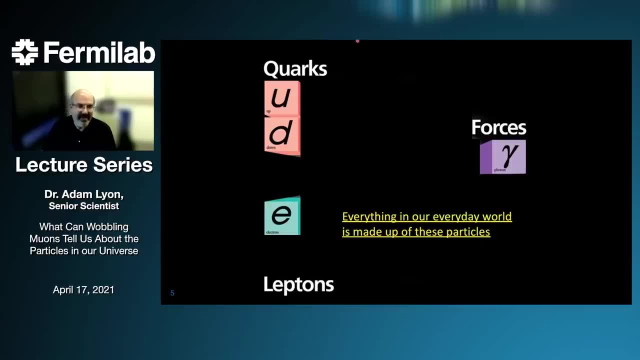 Robert Alverson- So so this soon now sort of build up the standard model- which is sort of our periodic table, Robert Alverson- Of of subatomic physics and now very told, told you about three particles, up up quark, the down quark, and the protons and neutrons and the electron. 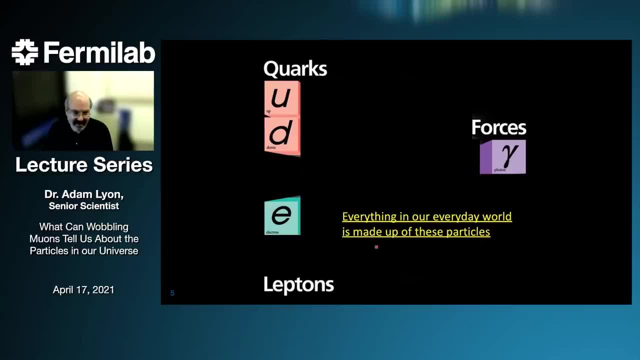 Robert Alverson- And what's really amazing is that with these three particles, that pretty much describes matter in our everyday world. everything- you, me, the planet, Robert Alverson- Cars, dogs, everything that you know- it's made up of up, down and and electrons. 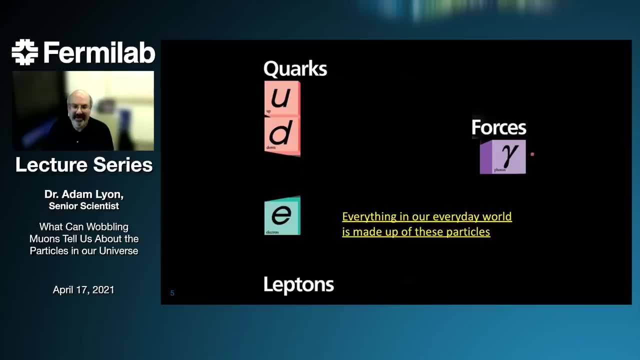 Robert Alverson- there's also- I mentioned the gluons- that's a force particle for the strong force. there's, Robert Alverson- photons. you probably have heard of those. they carry the electromagnetic force. in fact there's photons hitting from sets sent out by your screen, hitting your eyes. so photons are very important. 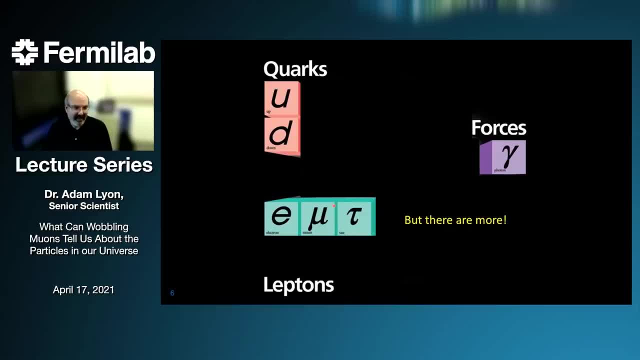 Robert Alverson- So it's really interesting in particle physics is that as we've done experiments and look for more particles, we found more. Robert Alverson- So the electron has some heavier cousins, has particle called the muon- we'll talk about this one a lot- and even heavier cousin, call, call the towel. 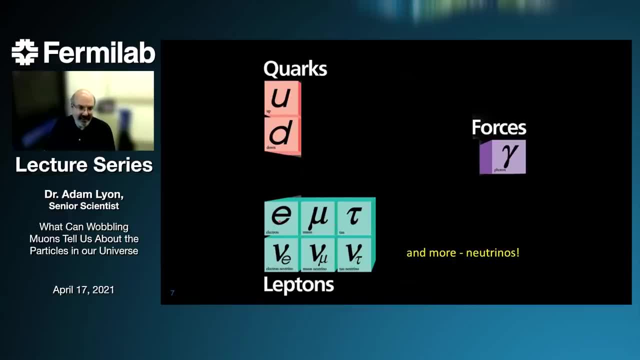 Robert Alverson-. And then there are other particles that are associated with each of the electron muon and towel. collectively these are called leptons, Robert Alverson-, And these other particles are the neutrinos. and these are really fascinating, interesting particles. for me, lab has become the world's premier. 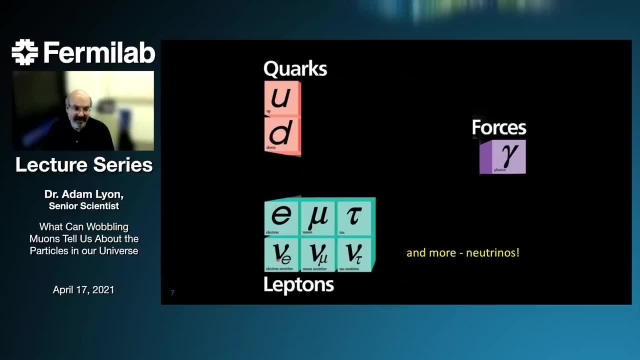 Robert Alverson- particle physics, laboratory and studying neutrinos. we have many neutrino neutrino experiments and we're building new ones. Robert Alverson- we're building a big experiment in a mine in South Dakota called dune. you've probably heard talks about that if you pay attention to. 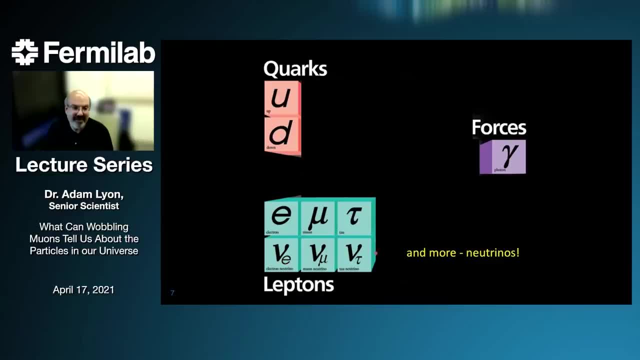 Robert Alverson- The Fermi lab on YouTube and things like that. I won't talk about neutrinos very much for will concentrate instead on the muons, but neutrinos are very interesting, Robert Alverson- And along with the, with the additional leptons, we've discovered additional quarks. 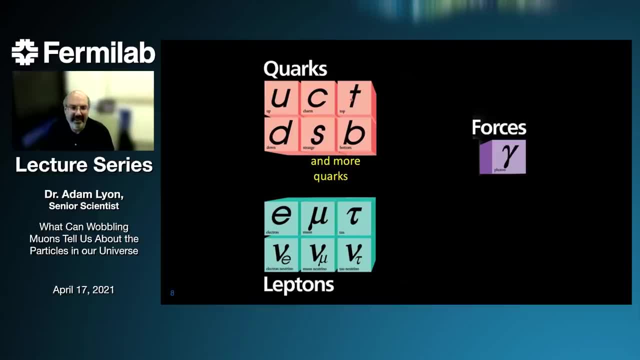 Robert Alverson- So, like I was at the zero experiment when the top quark was discovered in 1995, that was another very exciting time. and so you see this sort of these three families, three columns of of of fundamental particles, Robert Alverson-. And then, to round out the force carrying particles, we have a photon, the glue on I talked about, and then there's the weak force. 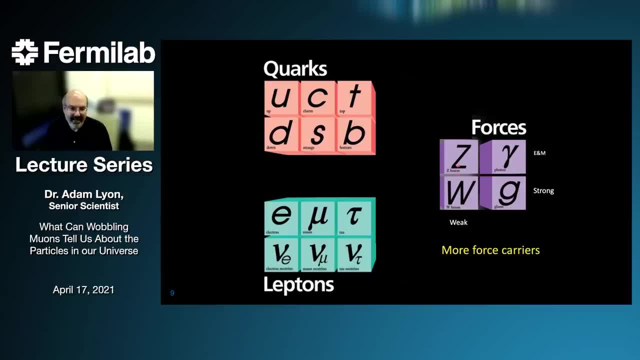 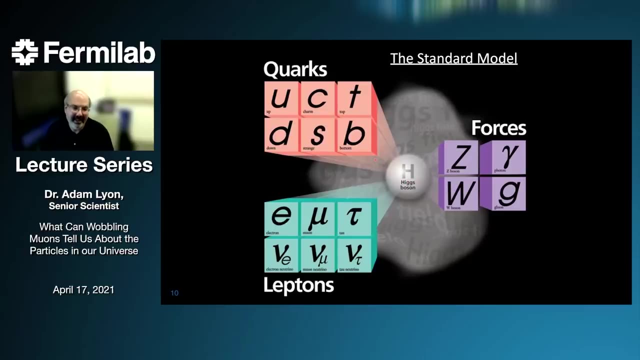 Robert Alverson- Which is involved in radioactive decay and that has to force carrying particles. heavy w article and a heavy z particle. the w and Z goes on, Robert Alverson-. And then there's one more particle that was predicted for quite a while. I was finally discovered at the large and experiments on the large hadron collider at CERN. 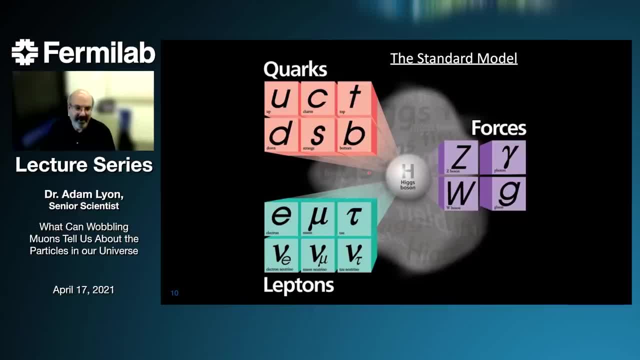 Robert Alverson-, And this particle is the Higgs- Robert Alverson- goes on. so this made you know all the news and 2012, and this completes the picture of the standard model, Robert Alverson- And we think that well, Higgs goes on- is involved in giving mass to to to particles in the standard model and this is the the picture of what we have of of the Sarah model, and this has been tested with literally thousands of analyses and and all the particles exist and we study them. 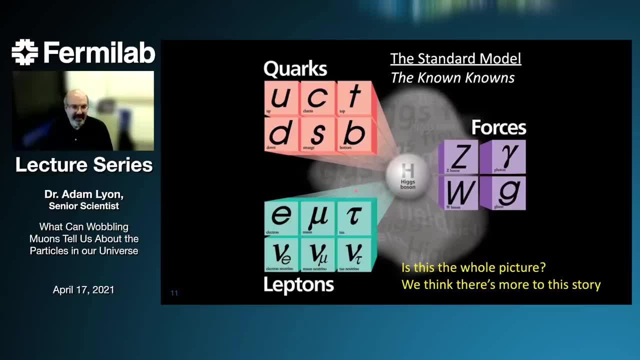 Robert Alverson- But, Robert Alverson- We have this notion that you know. we want to ask: is this the whole picture? is there more to the story? and we think that this is not the whole picture, that that there must be more to the story. 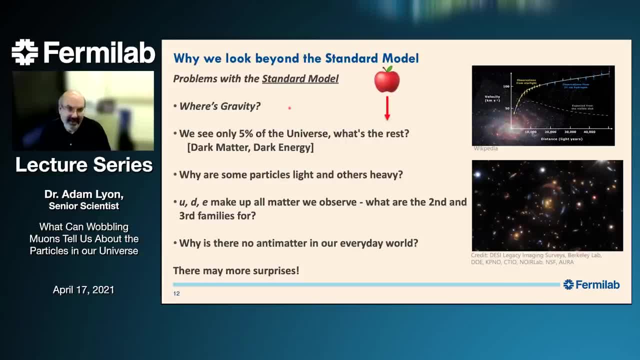 Robert Alverson-. And so we look beyond the stair model to try to look for, look for things that that the stair model doesn't explain and find other theories that can encompass the stair model and explain these things. so, for example, when I went through the forces, you might have noticed that one force was missing. 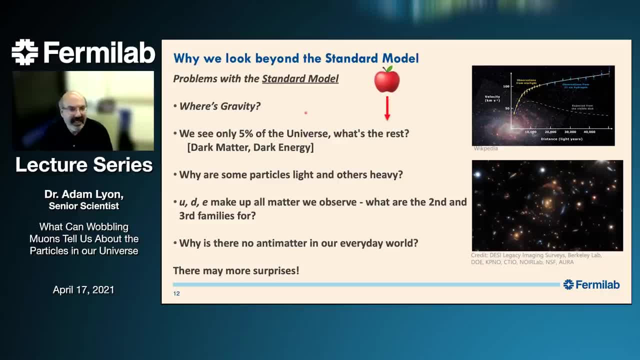 Robert Alverson- That was gravity. of course, gravity is very important for us, so the standard model does not describe gravity at all, and that's a that's a feature we would like to have. Robert Alverson- You probably, if you follow a lot of, 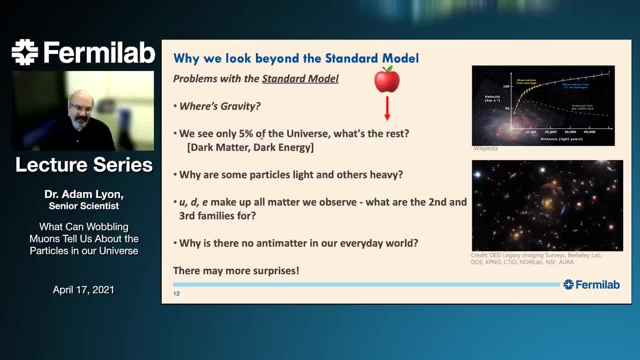 Robert Alverson- Business and science recently. you probably know that our everyday world is really only 5% of the universe. the matter in our, in our everyday world. we know that there are, there's matter, that, that, that be that interacts gravitationally but not with 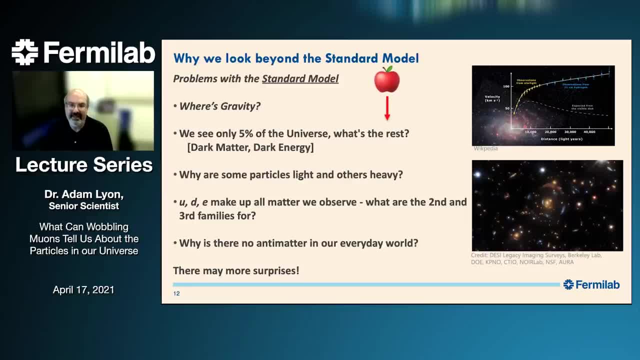 Robert Alverson- The electromagnetic force. so, for example, we look at galaxies and we look at stars at the edges of galaxies. we can calculate- Robert Alverson- By how much mass there is in the galaxy, how fast those stars should be going. and we find them to be going much faster than the audit be going. 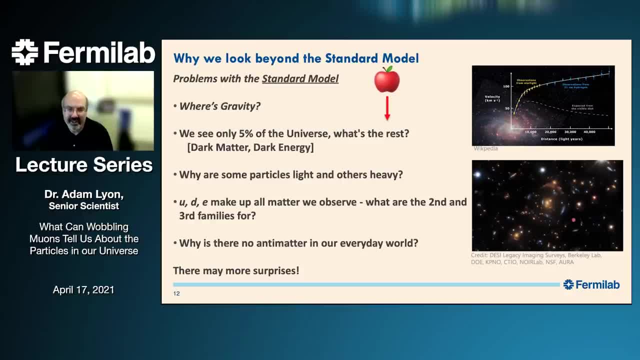 Robert Alverson- And we also, actually astronomers, find these structures called gravitational lenses. where there's a background galaxy, that's picture is distorted- Robert Alverson- By a foreground galaxy, and there's not enough mass and the foreground galaxy to do that. so we think there's extra matter. 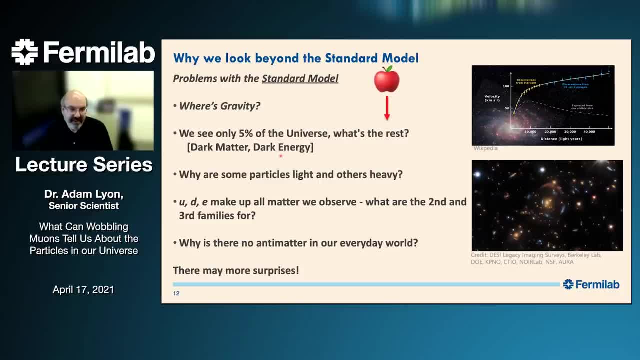 Robert Alverson- That we can- Robert Alverson- see called dark matter. we know the universe has been expanding for quite a while. as we know, for quite a while the universe has been expanding, Robert Alverson- And recently, and near 2000 or so, we just discovered that the expansion is accelerating. so there's some energy that's feeling that and we don't know what that is. that's called dark energy. we have 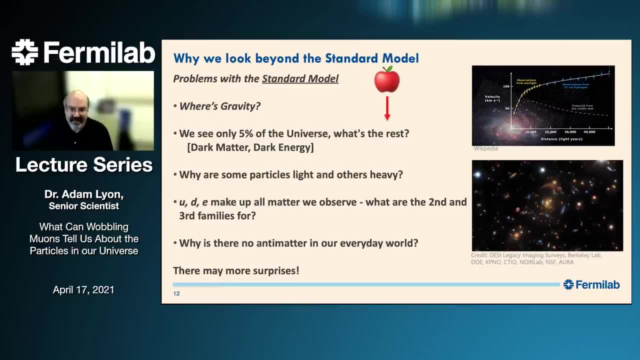 Robert Alverson- Several experiments are from. you know. i'm looking for dark matter and then a galaxy survey and understand dark energy. so formula is involved in that too. Robert Alverson- We also want to ask questions, like you know. why is the electron so light and the top part so heavy? 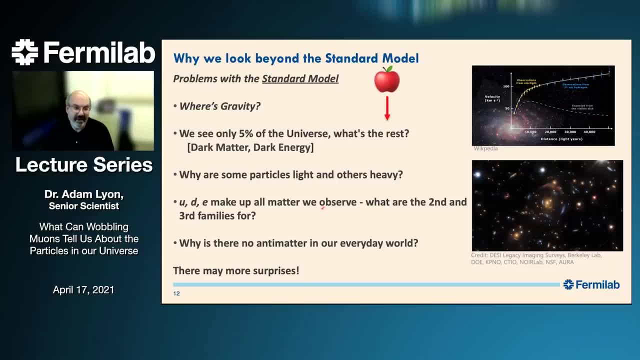 Robert Alverson- I mentioned the three particles that basically make up our everyday world. what are the other particles for the second and third families, those other columns in that table? Robert Alverson- we're all made of matter. anti matter is not really found in our everyday, everyday world. why is that? where did the any matter go? and maybe there are more surprises that will that there are out there, so theorists. 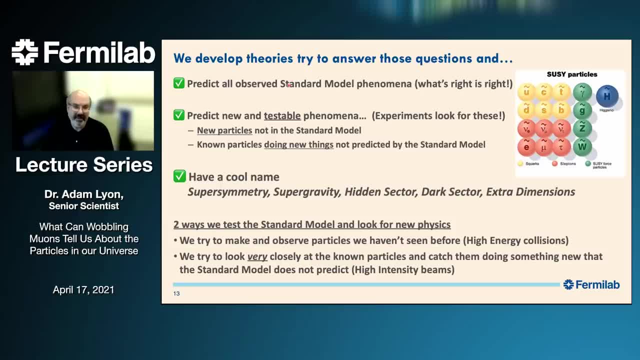 Robert Alverson- try to develop extensions to the standard model to try to answer these questions. Robert Alverson- So to pretend you're a theorist and you're coming up with with your model to try to explain some of these things, Robert Alverson- So your model has to have us have certain things. so, for example, you have to. you know, whatever the standard model predicts, that we've, that we've tested. 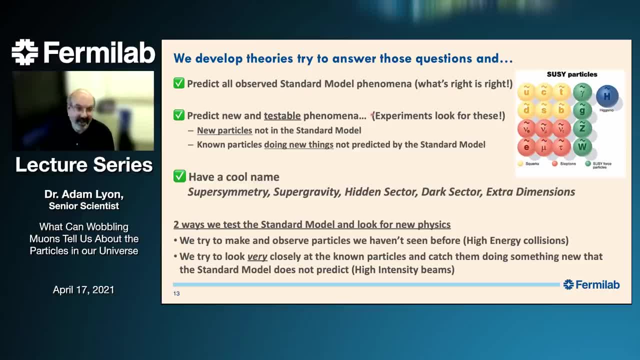 Robert Alverson- Your model had better do that to you know what's right is right and your model has to predict the same things. hopefully your model predicts new and testable phenomena, like maybe new particles- Robert Alverson- that are not in the standard models. we can build experiments, look for those. here's an example of this. is an extension to called super symmetry. that predicts many, many new particles and we've searched for these at the temperature on a Fermi lab and now at the LHC. 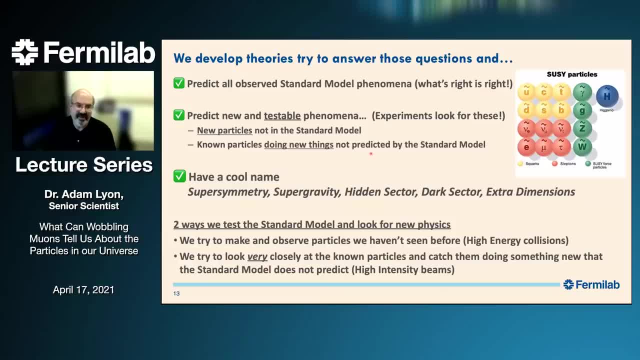 Robert Alverson- You can also predict the particles that we know about but maybe behaving somewhat differently than than what the standard model predicts. Robert Alverson- So those are things we can test. many of these models have kind of cool sounding names, like super symmetry. 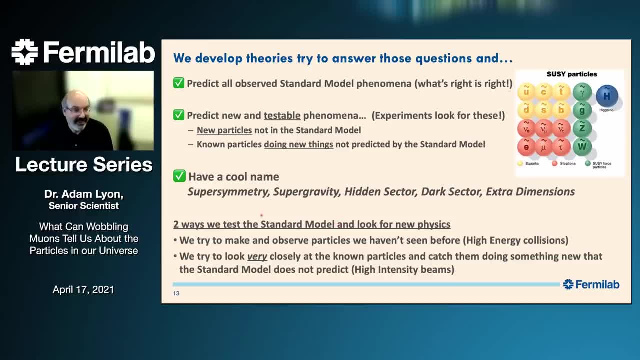 Robert Alverson- super gravity, extra dimensions, things like that, to get people interested, Robert Alverson-. And so really there's, there's two ways that expert experimentalists go about: testing the theorem model itself and also looking for for this new, for these extensions to this theorem model. 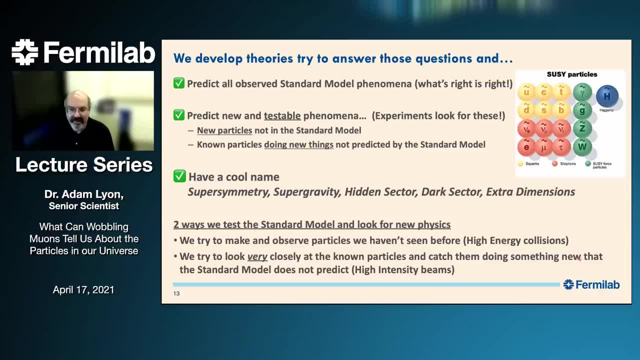 Robert Alverson- And what we do is we try to make. one way to do that is to try to make these particles in high energy collisions. so the LHC now trying to do that, Robert Alverson- And so so look for. 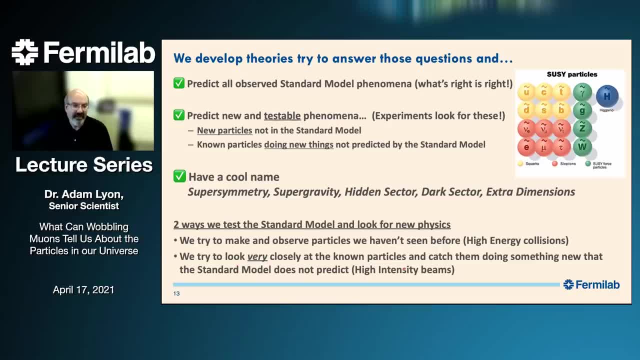 Robert Alverson- These particles we haven't seen before, and also trying to look very closely at the at the particles we do know about studying them very precisely to try to catch them doing something, Robert Alverson- That maybe the standard model does not predict, and so for that you need lots and lots of particles, and so we typically call that high intensity. 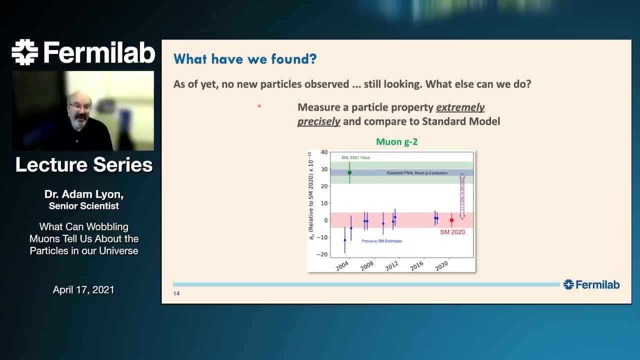 Robert Alverson- There we go. Robert Alverson- Okay, so you haven't heard about any new particles being discovered, Robert Alverson- Beyond the standard model, even though the LHC has looked really, really, really hard. Robert Alverson- Experiments have many, many analyses looking for particles from supersymmetry and other models. they are still looking. 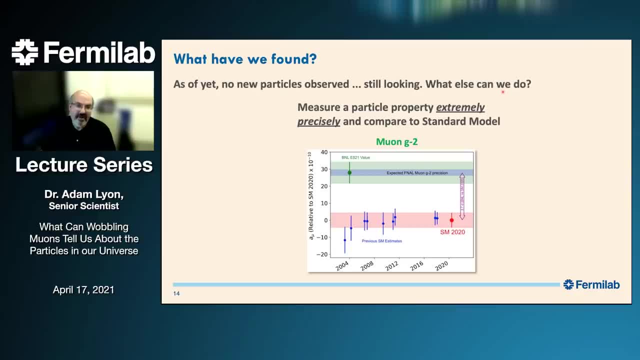 Robert Alverson- In fact, at the end we'll sort of talk a little bit about where that's going. so what else can we do while they're doing that? so, Robert Alverson- As I mentioned, we can study some proper particle properties very precisely compared to the standard model. 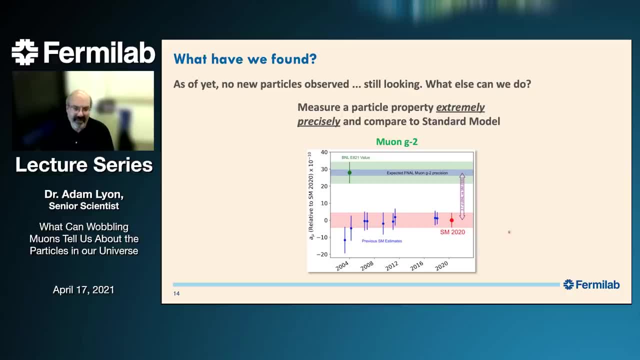 Robert Alverson- And this experiment, muon g minus two, is one of those types of experiments that does that. and actually this experiment is very special- the latest, Robert Alverson- The one before ours- that the the result that came from brookhaven about 20 years ago, brookhaven national laboratory. they did this experiment. 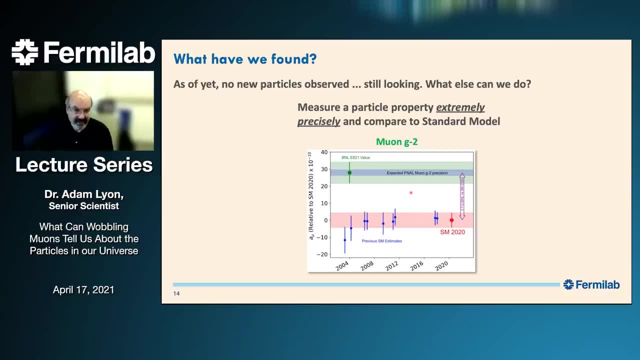 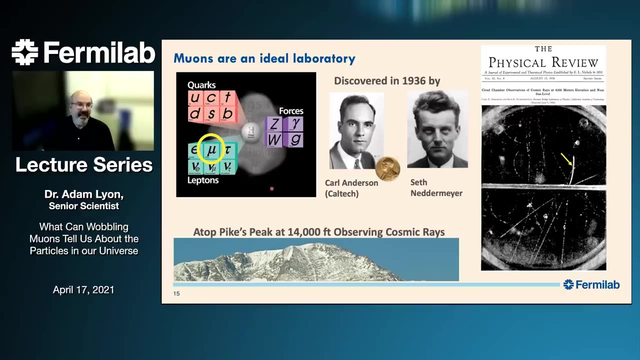 Robert Alverson- And they measured a slight discrepancy with the standard model. not enough to claim a discovery, but enough to be really, really interesting. so we're going to talk about this tonight and what Fermilab has done in our experiments- Robert Alverson- And our result. Okay. so I said I would talk about muons a lot, so muons are, in fact, a really nice laboratory. 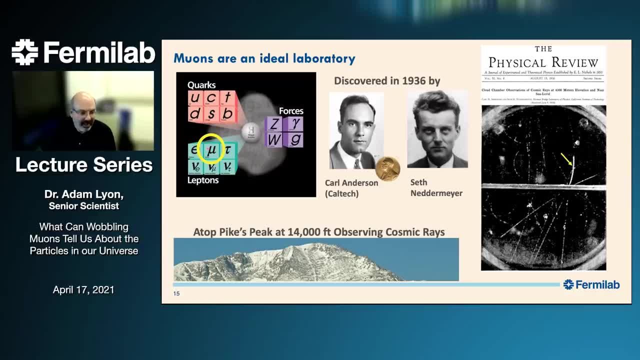 Robert Alverson- For for studying fundamental physics. so here's where the muon is and our our table of standard model particles was discovered 1936 by these two gentlemen from caltech- Robert Alverson- The first one, Carl Anderson, actually got the Nobel Prize for- for discovering anti electrons, or positrons, or anti matter. 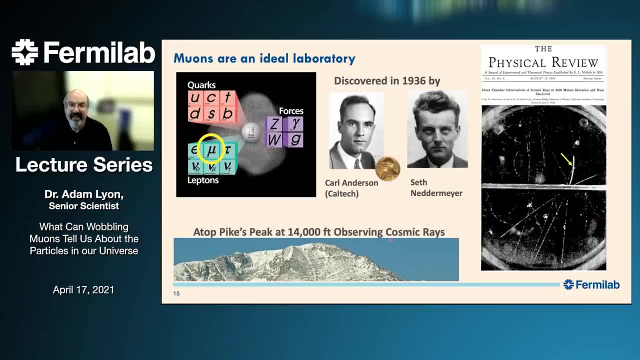 Robert Alverson- Basically, they took this device called a cloud Chamber up to a really high peak so they could see particles coming down from the sky- they're called cosmic ray particles- and they saw Robert Alverson- tracks in this cloud Chamber and there was a magnetic field to bend the tracks and they saw a particle here that didn't bend like the particles that that they knew about, not like how electrons and protons bend, and so eventually this, this became known as the muon. 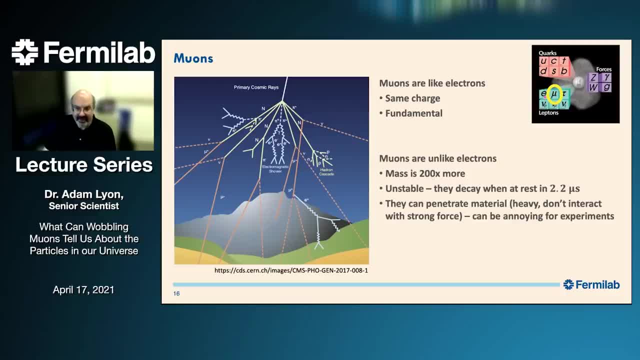 Robert Alverson- And muons are, are are like electrons. they're in sort of the same row here in the standard, standard model picture. they have the same charge as an electron. and the lights just turned off. people still see me, okay, Robert Alverson-? Or do I need to go turn on the lights again? lights on a timer here on this floor, so 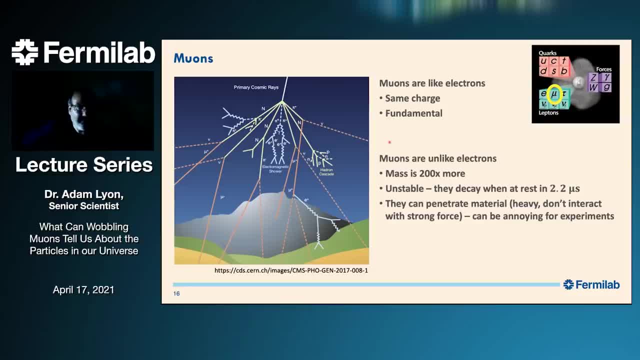 Robert Alverson- i'm just going to keep going and hopefully, hopefully, that's okay. Janet Callahan- um, it might be a good idea to turn the lights on, if you can. Robert Alverson- Okay, give me one second. Janet Callahan- Great, Thank you. 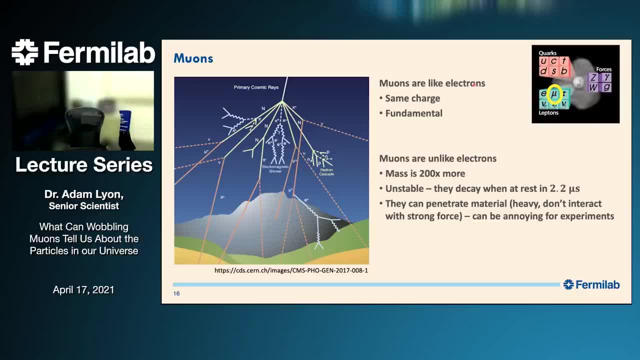 Robert Alverson- Okay, sorry about that. I was actually filling with the lights hoping they wouldn't do that, but uh, but they didn't anyway. okay, so let's see. so muons are like electrons, Robert Alverson- they're also fundamental. so we think they have- they don't have- any internal structure. but muons are unlike electrons in that they're- they're quite a bit heavier than electrons. 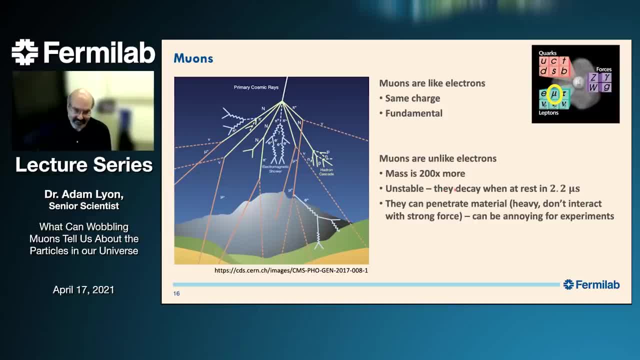 Robert Alverson- they're unstable. they don't live very long. they live for about two- Robert Alverson- microseconds at rest. then they decay to electrons and neutrinos. Robert Alverson- And one thing that's that's interesting about muons is that they can penetrate a lot of material. so here's picture of a cosmic Ray hitting the atmosphere and makes lots of, lots of particles. 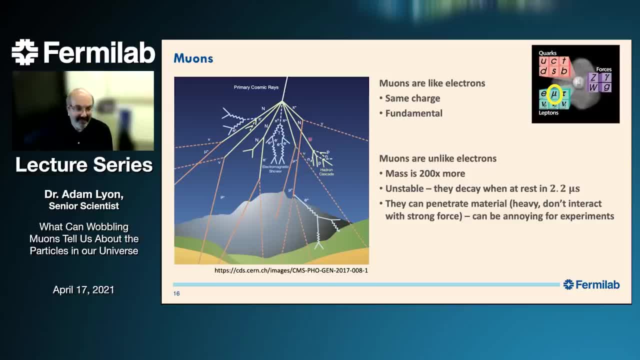 Robert Alverson- Some of those particles eventually, or muons, and muons can- can penetrate buildings and things like that and there's nuance going through us. right now they don't really do very much to us, but if you're running a very sensitive experiment, 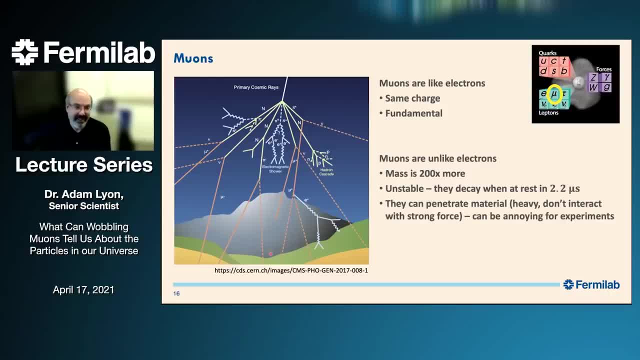 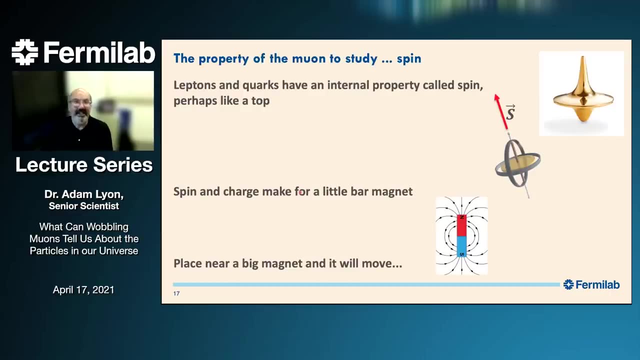 Robert Alverson- And a muon goes through your experiment. that might confuse what you see. so, Robert Alverson- A lot of neutrino experiments that are incredibly sensitive have to go underground to avoid being affected by cosmic Ray muon. so this was part of all that we study very intently is an annoyance for other other experiments. we just kind of funny, I think. 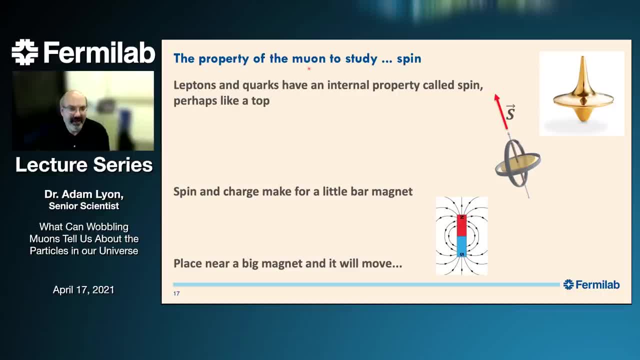 Robert Alverson- Okay, so we're going to study a property of the muon very, very closely and that property is spin. so leptons and quarks have this internal property called spin, Robert Alverson- And it's- we could say it's an intrinsic angular momentum and we sort of 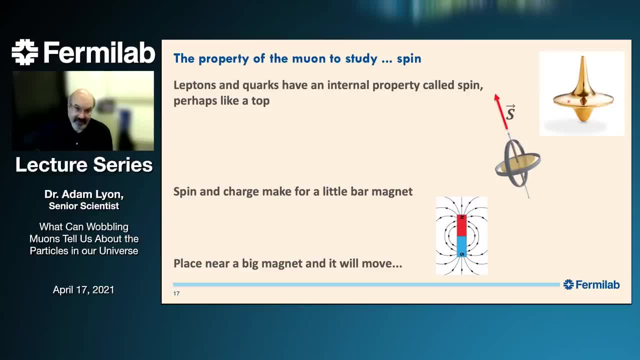 Robert Alverson- imagine that it's spinning like a top. we don't, we don't know if that's what, is that what? that's what it's really doing. but this, this analogy, seems to work from in many ways, Robert Alverson-. And so if you've all played with gyroscopes, I hope you have. you spin up this, this gyroscope, this disk starts spinning really fast and this thing can kind of stand up all by itself because of its angular momentum. 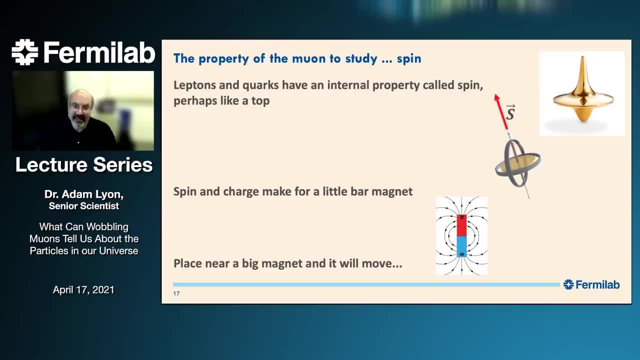 Robert Alverson-. And so we're going to use this analogy a lot and we're going to say: the spin direction is the axis of the gyroscope, Robert Alverson- So the disk is spinning in a certain direction and Robert Alverson- That. 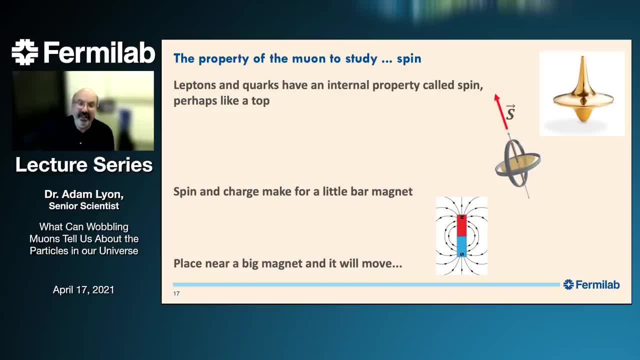 Robert Alverson- That, Robert Alverson- It's going to spin along its axis. so when I say the spin direction, you know, picture this little gyroscope and where this arrow is pointing, we'll see this again. Robert Alverson- spin and charge, make for a little bar magnet. and when we place a bar magnet into another magnet, 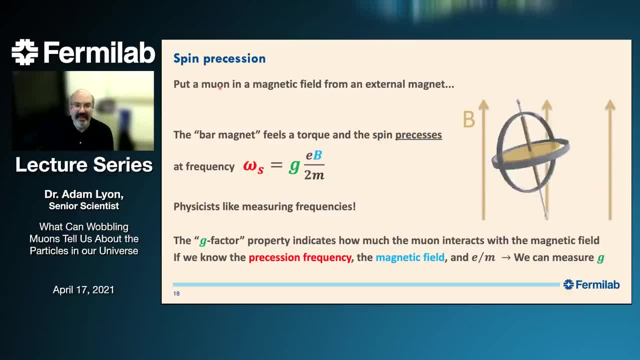 Robert Alverson-, Then that bar magnet will move a little bit. so if you put, say, a muon magnetic field from an external magnet- so here's our muon spinning, Robert Alverson- And here's our magnetic field with strength, be then this little magnet fields of torque and the. 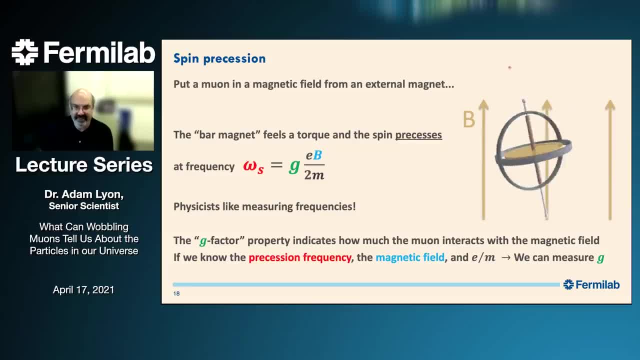 Robert Alverson- spin will process, so the spin vector and the other axis of this thing will move around- sort of like it's shown here, Robert Alverson- And it moves with a frequency that we can measure and that frequency is related to the strength of the magnetic field, some constants like the charge and the mass of the muon, and this really interesting number here called, called, or this, this quantity called G. 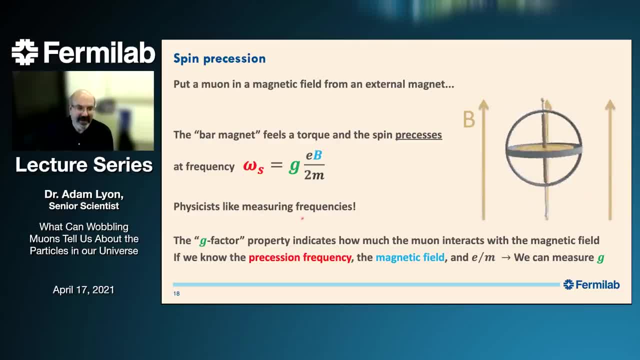 Robert Alverson- Which is called the G factor. Robert Alverson- And the G factor is actually a property of the particle and, Robert Alverson-, That basically says how much that particle interacts with it, with them, and that it feels. Robert Alverson-, So if G is really small, then the procession will be really slow and you can say, well, the particle is not really feeling the magnetic field. 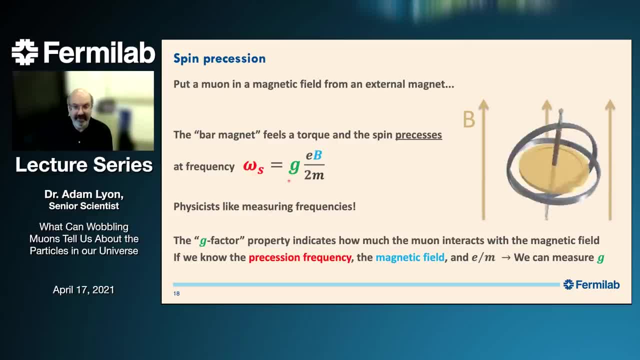 Robert Alverson- If G is really big and so then the spin free procession frequency will be really fast, then then the particles really feeling that magnetic field, right. so this sort of measures, the strength of how well particle feels magnetic field? Robert Alverson- So so if 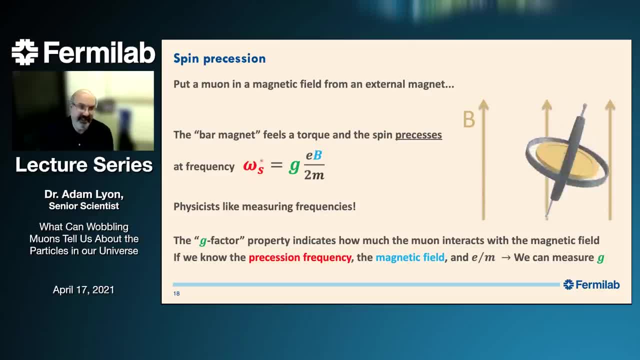 Robert Alverson- We can measure some of these things. we can measure the procession frequency- and this is this- can measure frequencies really well, Robert Alverson-. And if we know the strength of the magnetic field, whether it's a refrigerator magnet or an MRI magnet, we can measure that or determine that. then we can measure what this G factor is, and that's in fact what, what we've done. 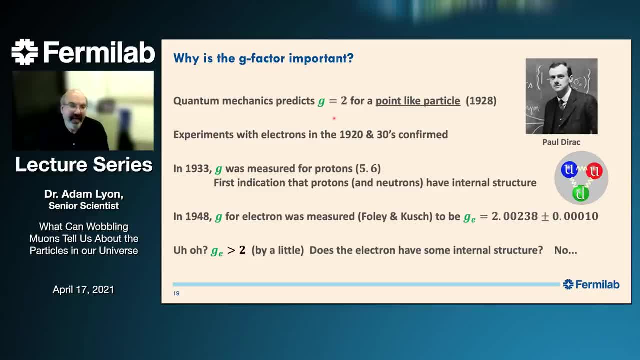 Robert Alverson- So the G factor is really important. it's a, it's a, it's a quantum mechanical effect and quantum mechanics actually predicts that G is equal to two. Robert Alverson- For a point, like Robert Alverson- particle and this was actually derived by Paul the rack, a very famous physicist, in 1928, and this was confirmed with with electrons in the 20s and 30s that the G was about equal to. interestingly. 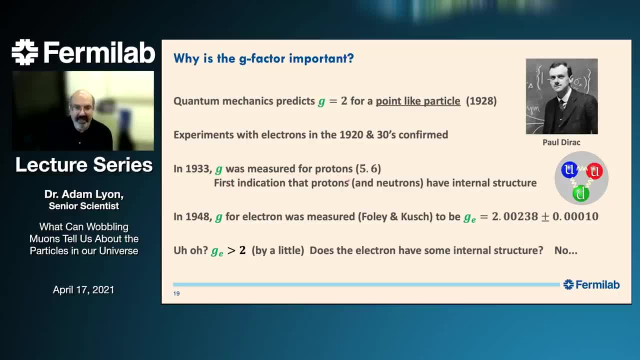 Robert Alverson- A little bit later, when some, when people measure G for the proton, it wasn't, they didn't get to, they got a kind of a strange number, Robert Alverson- And that was one of the first indications that protons and neutrons to have an internal structure, that they're made of quarks, they're not, they're not point like particles. this is, of course, has figured out much. 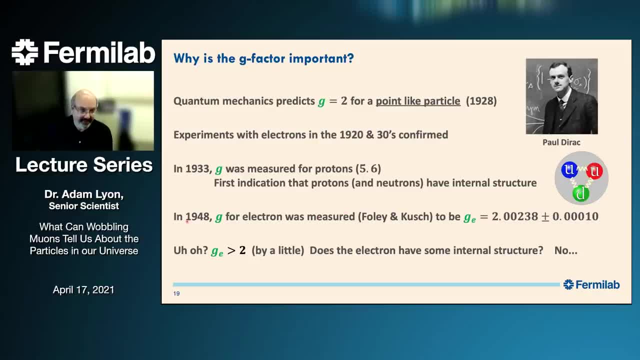 Robert Alverson- Much later, but this was kind of a hint of that. and then in the late 40s, as there was a surprise, this G factor for the electron, which had been close to two for quite a while- Robert Alverson- fully encouraged it- an experiment where they found G to be a little bit greater than two. 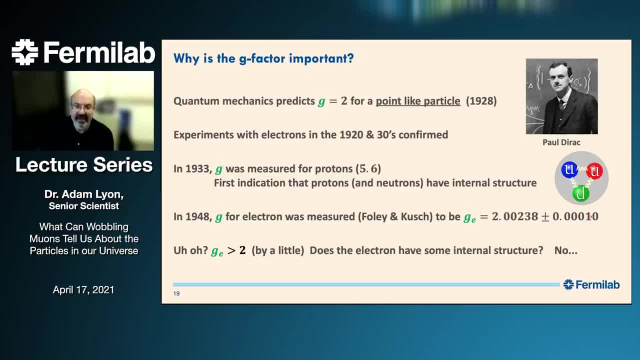 Robert Alverson- Not much greater, but a little bit greater, and their uncertainties, you know, cannot account for, for this discrepancy. their uncertainties are quite good. so this plus or minus point 0010, that's, Robert Alverson- How they're, they're, they're degree of 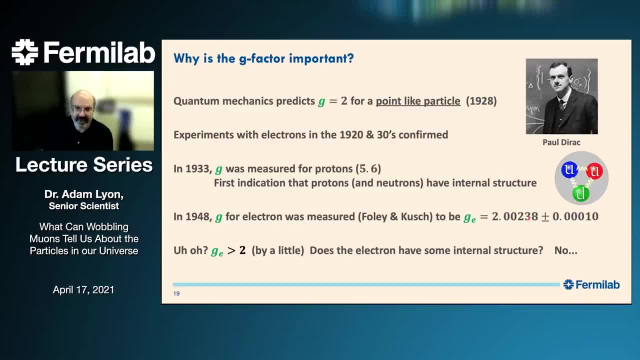 Robert Alverson- What, how much? they believe this number is right, so it's. so the three could be a two or four, Robert Alverson- And actually this, the way this is written, this kind of pain, all the zeros. what we actually like to do is. 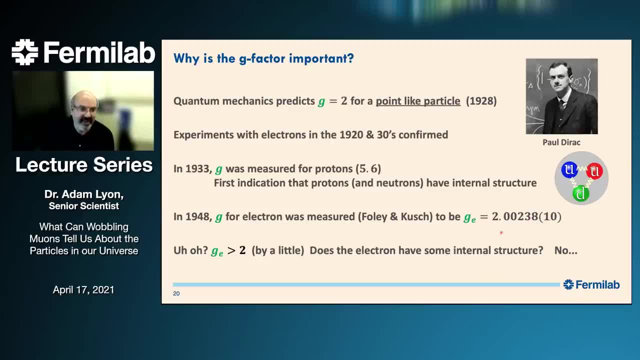 Robert Alverson- Say the last two digits. here's the error in the last two digits. that's the same as what you saw before, Robert Alverson- So what's going on here? so G for the electron is now measured to be a little bit greater than two. why is that? does the electron have some internal structure? 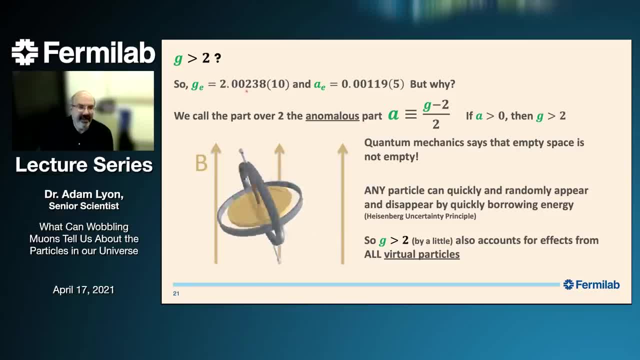 Robert Alverson- And the answer is in fact no. so here again is their result. Robert Alverson- G is a little bit greater than two, and actually the two is kind of a pain. so physicists like to get rid of things that are pain, and so we actually have a new quantity called the anomalous. 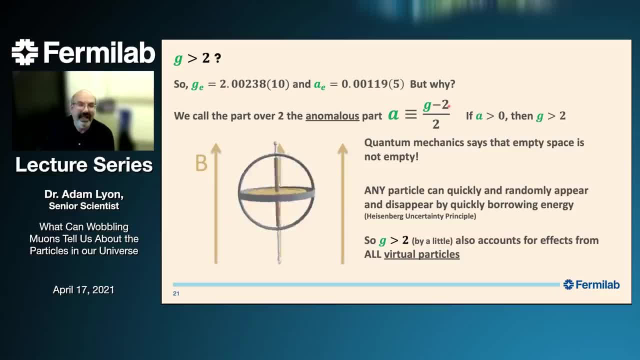 Robert Alverson- Factor, and for that we actually subtract off the two and divided by two, so it's the fractional part over two, and this is what we call the anomalous part- Robert Alverson- Of the magnetic moment. and so basically, all you have to remember is if a is greater than zero, than G is greater than two, and we'll kind of go back and forth. I have these in green, sort of 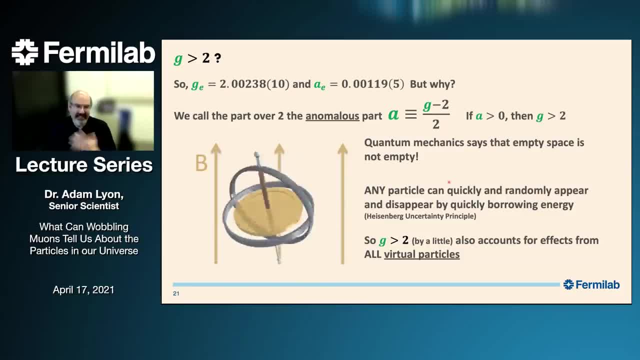 Robert Alverson- In a way that you know, these are all related. so what's going on here is that if you study quantum mechanics, quantum mechanics actually says- Robert Alverson- That, and this is the theory that describes how subatomic particles work and their world. quantum mechanics says that empty space is not actually empty. 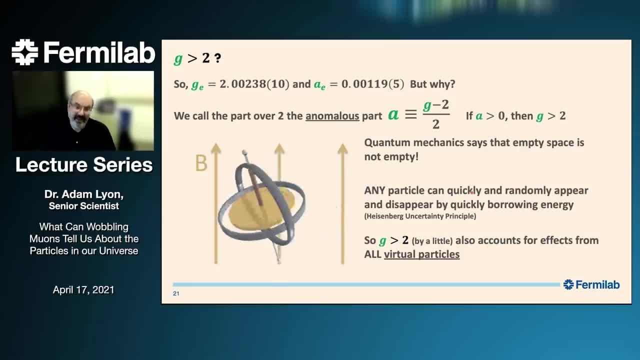 Robert Alverson- And that any particle, any particle can quickly and randomly appear and disappear by quickly borrowing its energy. this is related to the heisenberg uncertainty principle. Robert Alverson- Just have a little. I will animation here. so say you have a new on spinning around and a photon appears, it's gonna be me one or an electronic, doesn't matter, they do the same. 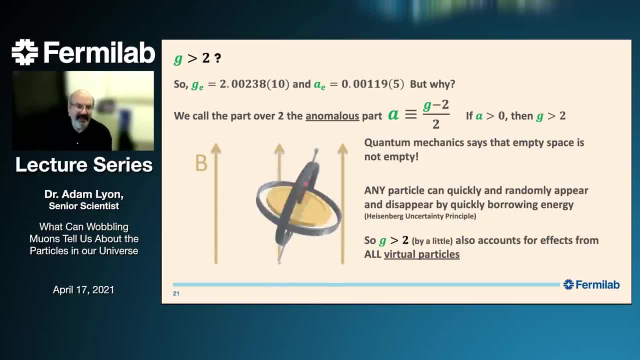 Robert Alverson- Or you have, you know, a photon appear and that then goes into electron positron pair and then you get a photon again. or maybe, Robert Alverson- Two particles with quarks appear, or Z boson appears, or, interestingly, maybe something we don't know is appearing and disappearing. 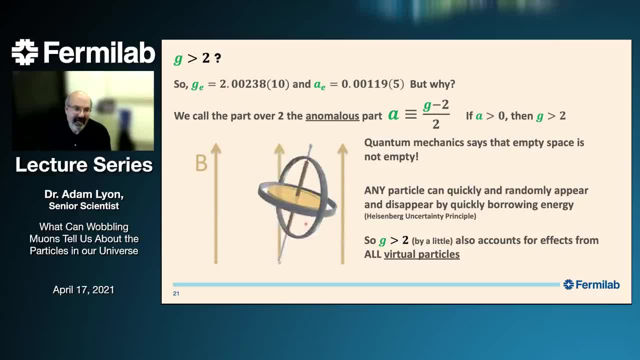 Robert Alverson- And so these are called virtual particles, Robert Alverson- And actually we can see, we can see them inside, see their effects inside protons and neutrons and things like that. so we know this, this, this picture actually works and so if G, being a little bit more than two, accounts for these effects from all these virtual particles, 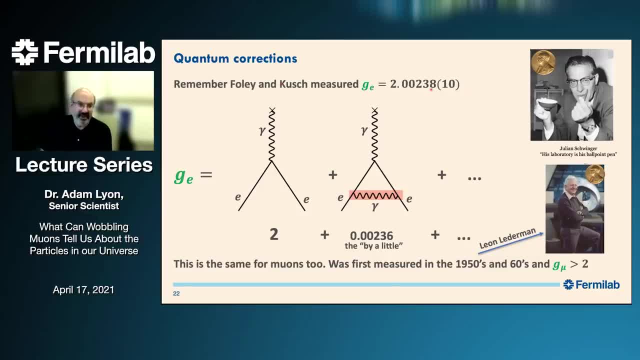 Robert Alverson- And you can actually, and so so remember, here we have this result: a little bit more than two. and this little bit more than two was first predicted- Robert Alverson- By this gentleman, Julian swinger, who got the Nobel Prize for this. this was in, I guess, the late 40s, early 50s. 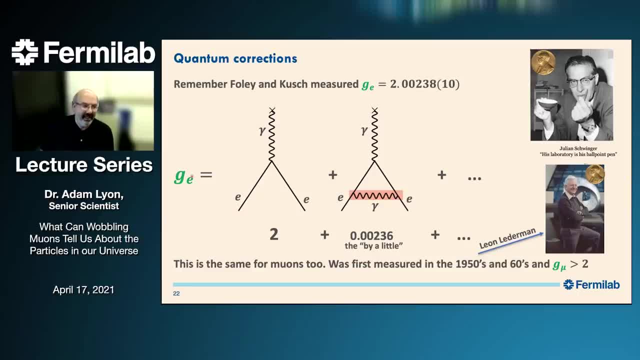 Robert Alverson-. And so the way this works is that we imagine sort of the, the, the G factor, being built up by the basic thing that's happening, the two part, which is the- the electron, Robert Alverson- interacting with the magnetic field. that's this photon and the X, that's the magnetic field. the electron sort of says hi to the magnetic field and then goes up, goes on again, so in and out, and then this little extra. 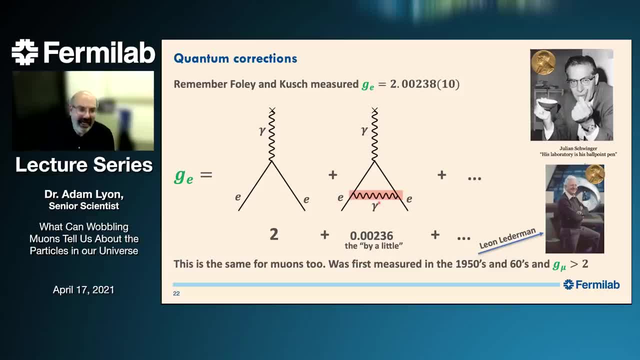 Robert Alverson- part here is where the photon sort of appears, and so the electron gives, gives a little energy to this photon and gets it back later on. Robert Alverson- And swinger actually calculated how much this interaction adds to G, and so he got this, which almost things that are very closely map, matches what, what fully and could cut. so this is the start of what we call quantum corrections to the diagrams. 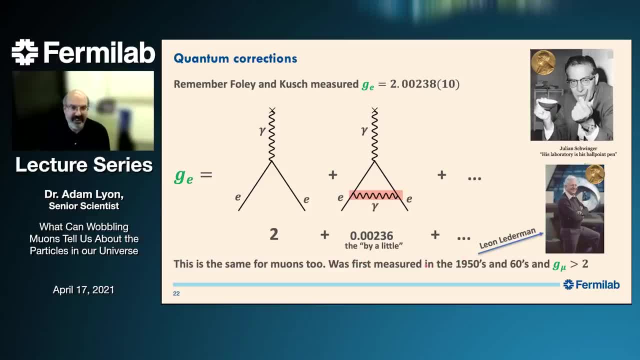 Robert Alverson- Actually the same thing happens for them. you on. this was confirmed in the in the Robert Alverson- 50s and 60s. and actually Leon letterman, who became the who was the second director of friendly lab he was, was led one of these experiments in the 50s for G, minus two of the new one. 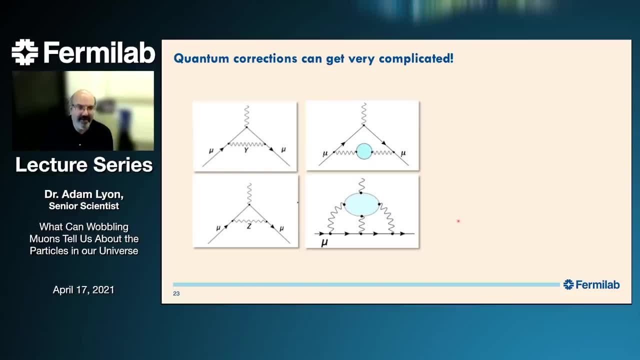 Robert Alverson- Okay, so I showed you that. that one picture of the quantum correction here here that is involving involving the photon. you can have other pictures as well. you can have the zebras on that one I mentioned you can have. 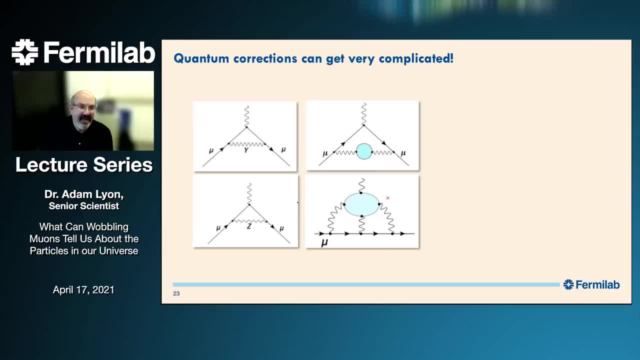 Robert Alverson- photons that go to quarks. I go back to photons again and then you can have a very, very complicated- Robert Alverson- funny looking diagrams like this one, again involving quarks, that sort of the blue, the blue ball there. 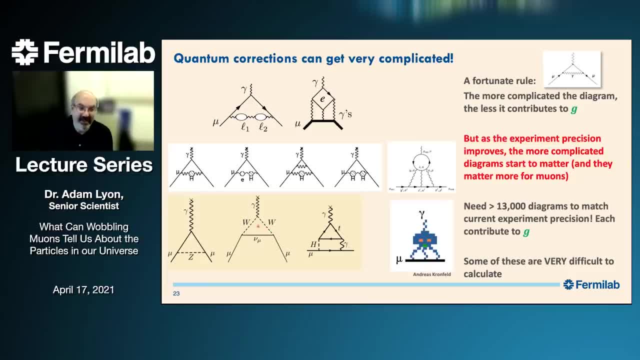 Robert Alverson- And you can sort of go wild. there's really an infinite number of diagrams involving you know lots of, lots of lots of these little loops you can imagine. you know two loops, three loops, 100 loops- Robert Alverson- And really interesting looking things. you can make them look like space invaders if you want. it's kind of neat. 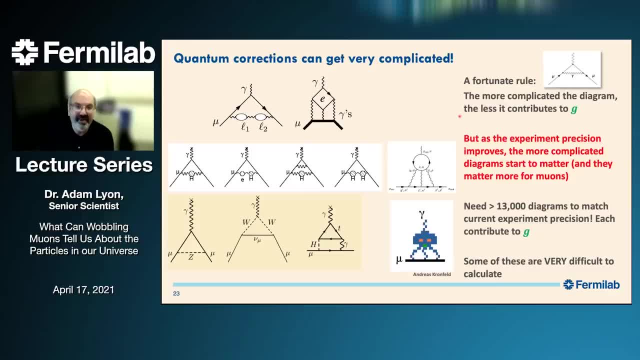 Robert Alverson- But there is a fortunate role. there's a good thing that happens, even though there's there's an infinite number of diagrams, Robert Alverson- The more complicated the diagram, Robert Alverson- The less it contributes to the G factor. so the more stuff going on, the less it contributes. and so this one, the most basic one, that's the one that contributes the most. 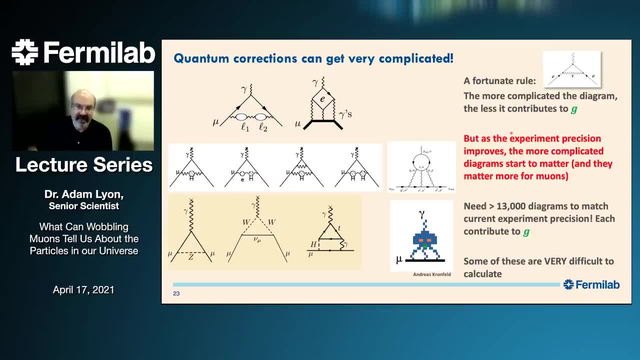 Robert Alverson- And the more complicated ones can, should be less so. at some point you don't have to calculate anymore because it just doesn't. you know they don't add very much, Robert Alverson- However, as our experiment precision improves, then you have to start worrying about these more, some of these more complicated diagrams, because these sensitive experiments you can see there's effects and see their effects. 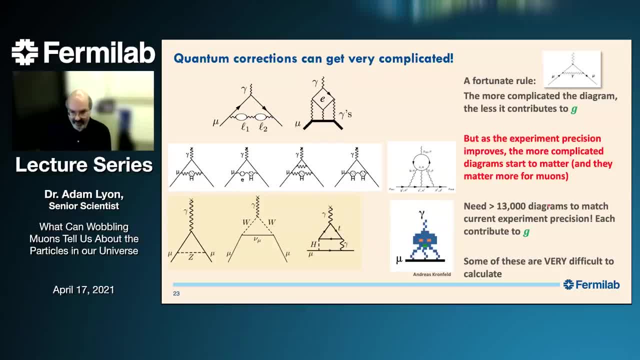 Robert Alverson- And so to to account for the the precision that our experiments are, and now the theories have to calculate over 13,000 of these diagrams, Robert Alverson- To to calculate what the, what the standard model prediction is for the G factor, and some of these are very difficult to calculate. 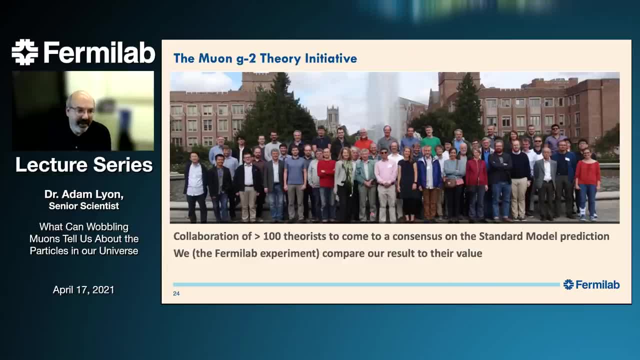 Robert Alverson- In a sort of an industry behind doing this, in fact, the fear of the theorists themselves have their own collaboration. now, this is only a couple years old, Robert Alverson-. There have been a lot of groups, theory groups. 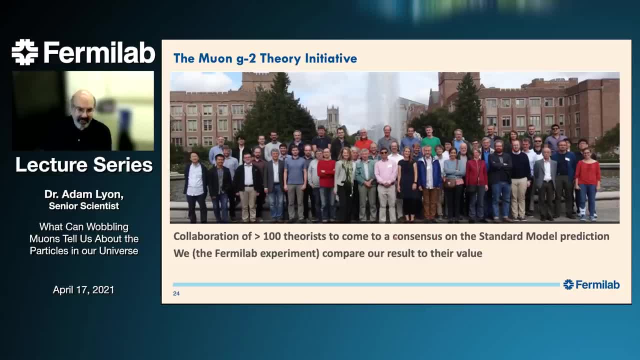 Robert Alverson- Calculating parts of G minus two, and so they form their own collaboration to come to a consensus- Robert Alverson- To put together all their different ways of doing things and come with one, one number for the standard model prediction that they can all agree on. 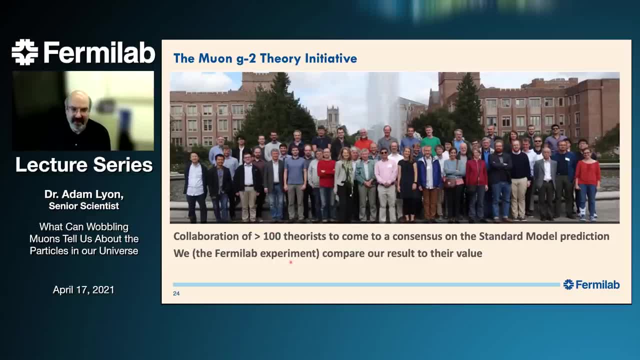 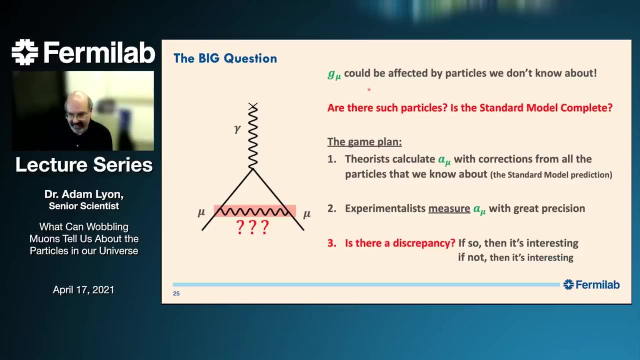 Robert Alverson- And this is what now? the formula experiment, our experiment. we will compare to their value, so we no longer choose which theorists to follow. the theorists themselves get together and give us the best value that they think is right. Robert Alverson- Okay, so I showed you also in that that animation, that there could be question marks, that could be particles. 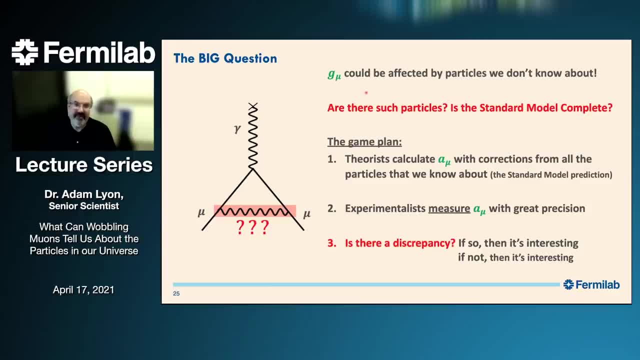 Robert Alverson- That we don't know about, that are in the mix of virtual particles and could be affecting the G factor. and that's what's really exciting- right, Robert Alverson- That we could be sensitive to particles that are not in the standard model. and then we can ask the question: is the standard model complete? so here here's the game plan. so the theorists will calculate on G, the G factor, or a, the anomaly. 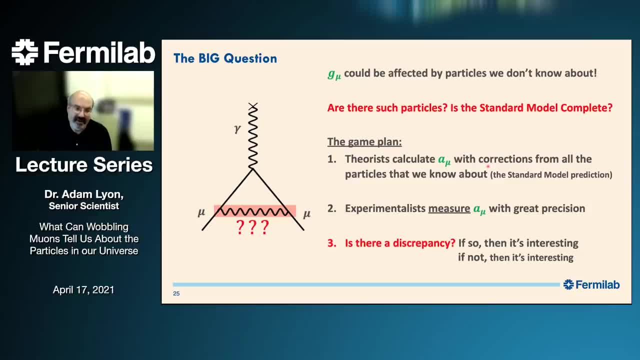 Robert Alverson- The anomalous part, with all these diagrams, from all these corrections, from the particles that we know about, that the standard model has and that's the standard model prediction. Robert Alverson- Experimentalists like myself make an experiment and measure the anomalous part of the G factor with great precision, right precision that matches their, their calculation. 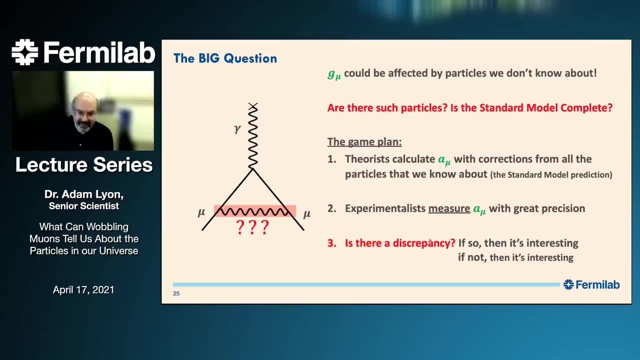 Robert Alverson- And then we look to see: do we agree? is there a discrepancy? and if there is a discrepancy, well then that's really interesting. Robert Alverson- Maybe there's a hint that there's something else going on, Robert Alverson- outside. 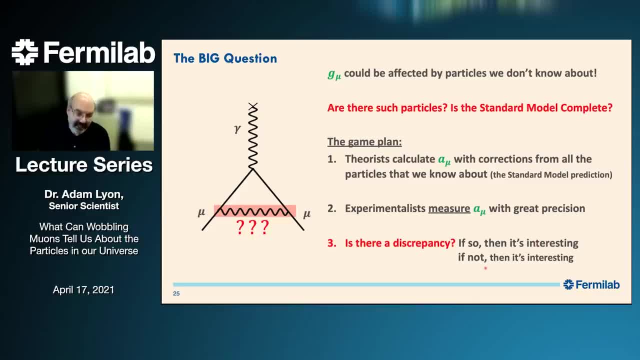 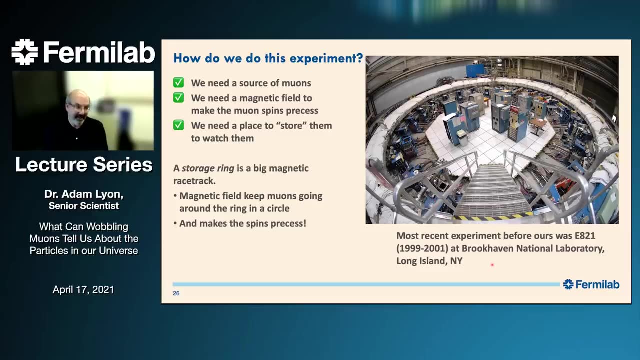 Robert Alverson- Inside this terror model that's affecting our muons and if we agree, well, that's also. you know, that's interesting to. maybe you would agree not quite as interesting as finding something new, but that's okay, it's all interesting. Robert Alverson- Alright, so how do we actually do this experiment? 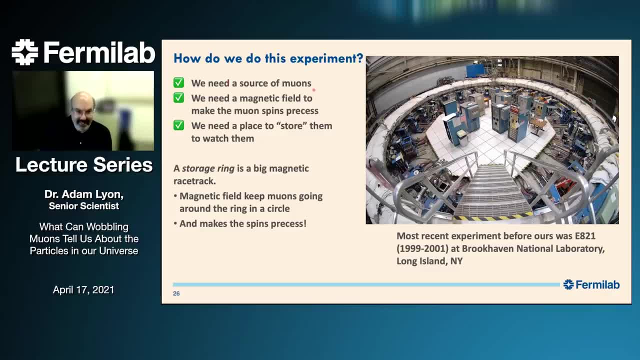 Robert Alverson- So we need a couple things. first of all, we need muons, need something that that gives us nuance, a source of nuance. using nuance from the sky, from cosmic rays, are not enough of them, Robert Alverson- In any in any one place to really use. 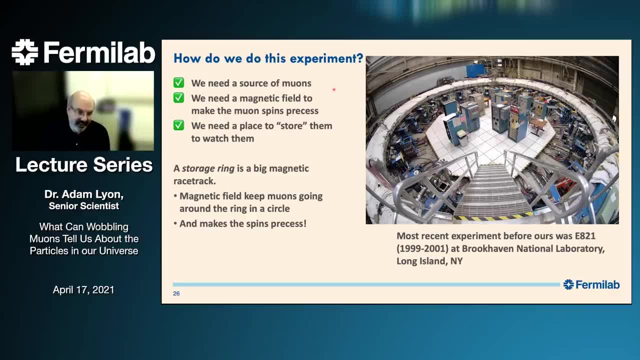 Robert Alverson- them for for this sort of experiment, although there are other experiments that study those cosmic rays. but we need a lot more nuance than that, Robert Alverson- We need a magnetic field to make the muons been processed. right, I showed you that. that gyroscope that's processing 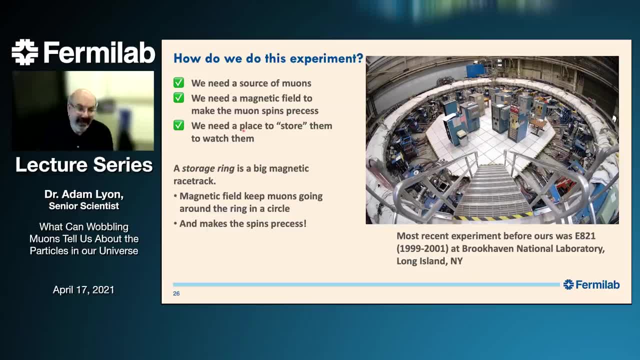 Robert Alverson- And we need to put them somewhere where we can watch them for a while. right, we have to give time for that procession to happen and time for the muon to decay, and so we have to actually watch them, Robert Alverson-. So there's a device called a storage ring, and that's what this picture is here. this is the storage ring of Brookhaven. 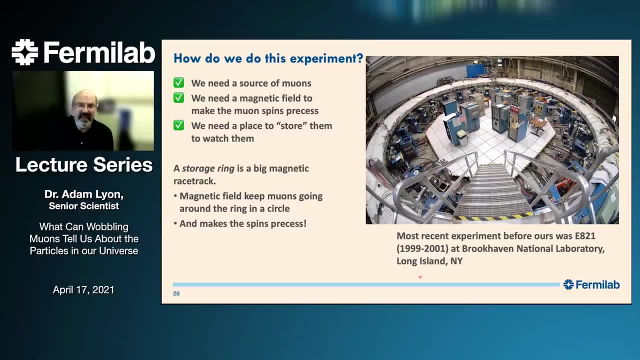 Robert Alverson- This was the experiment- Robert Alverson- done 20 years ago and storage rings are really nice for for this sort of thing, because it checks off two of these boxes. Robert Alverson- Storage ring keeps the muons going in a circle. that's what the magnet- this is a magnetic storage ring- so the magnet does keeps the nuance going in a circle so we can keep them there for a while and it provides them and then it feels to make the spins process. 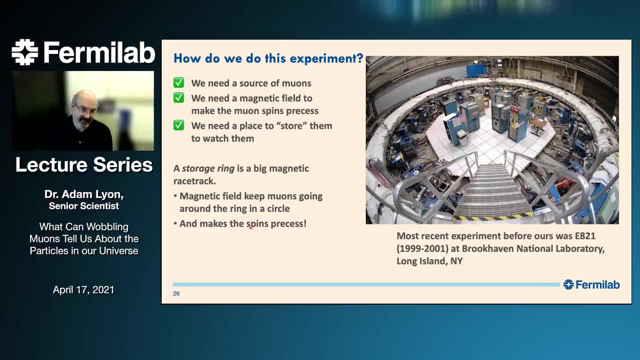 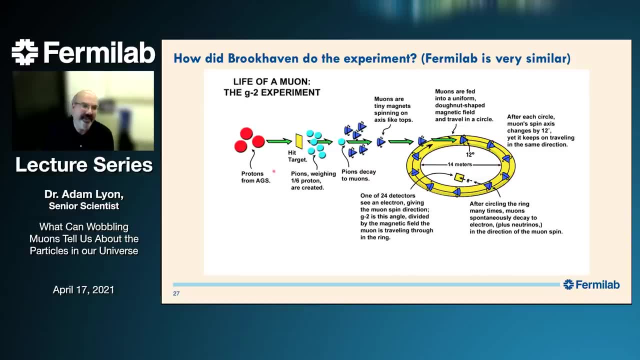 Robert Alverson- And so this was the ring of Brookhaven and that's that's what we're going to use. actually, Brookhaven has this really really nice diagram here to show how the experiments work, Robert Alverson- So i'll use it too. and the Fermilab experiment is almost the same. so you have a source of protons. Brookhaven has their accelerator. we have our accelerator complex that takes protons. 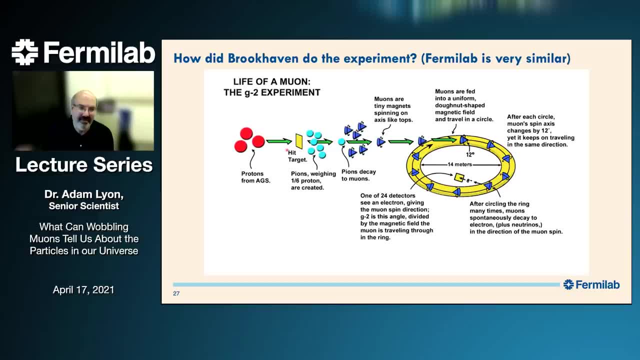 Robert Alverson- We always start with protons, because that comes from from a hydrogen model, and then those go through our accelerators and we accelerate them to high energy and then we smash those protons into a target, Robert Alverson- And because energy and mass are interchangeable. that's E equals mc squared. 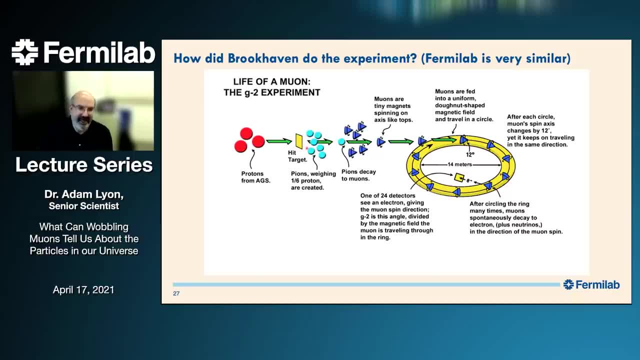 Robert Alverson-. A lot of the energy that those protons- Robert Alverson- are going to get- Robert Alverson- are carrying by because they're going very fast, can be converted to new matter and we can make a lot of different types of particles. a lot of stuff comes out, but particles called pions are the ones we're interested in. 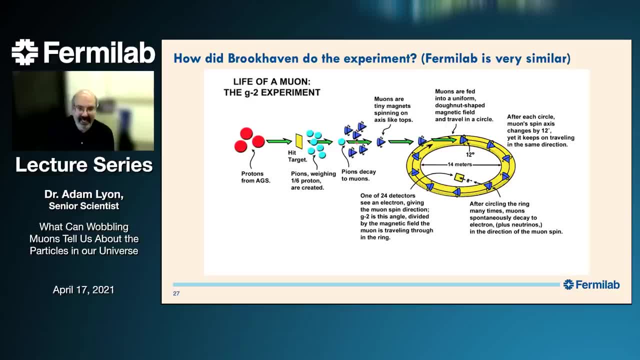 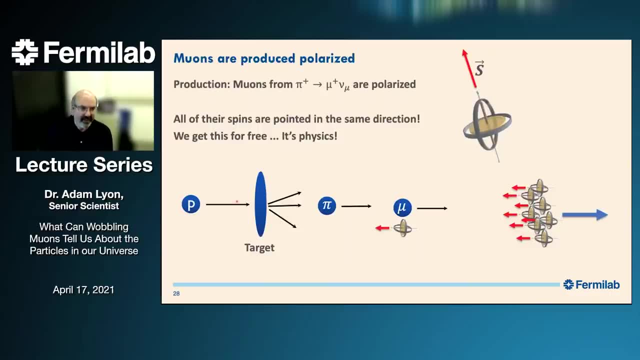 Robert Alverson- they're made of two quarks and those pions will decay to muons and neutrinos and these muons will have a very special properties. let's look at that, Robert Alverson- For a second. so here's our, here's protons hitting a target. we got lots of stuff, a lot. some of the what comes out, or pions. 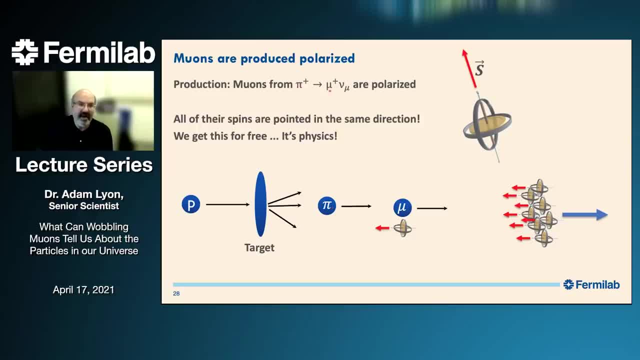 Robert Alverson- And a pion- Robert Alverson- will decay after a short period of time to a muon and a neutrino. we actually have used pi pluses because protons are positively charged and they like to make Robert Alverson- pi pluses, and so we're actually going to use mu pluses or anti muon. so actually our experiment uses anti matter, which is kind of cool. 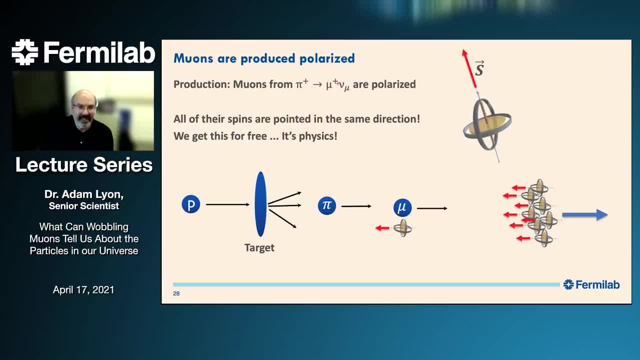 Robert Alverson- So the pi pluses decay to muons and a neutrino and actually we use this to also make neutrinos. we don't care about the neutrinos. you need a very different beam to if you're going to study Robert Alverson- neutrinos. so we make the muons and the neutrinos just just just go on their merry way and we never see them. they can go through everything, so it doesn't matter. 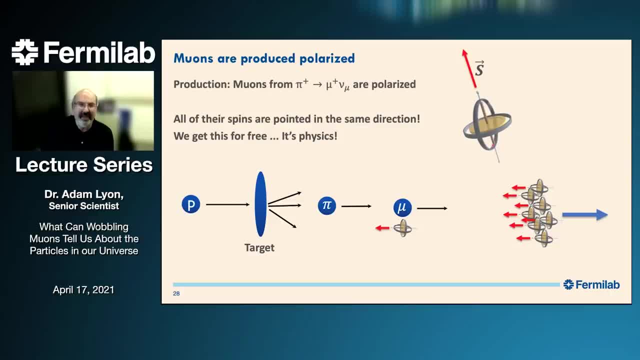 Robert Alverson- And what's a neat thing is remember how the spin works, that we have the spin axis. when the muons are produced, their spin- Robert Alverson- Is is always in the opposite direction that the muon is traveling. that is a property of the weak force, which is how this thing decays. and we get this for free. this is physics. so the muon spin is always in the opposite direction. 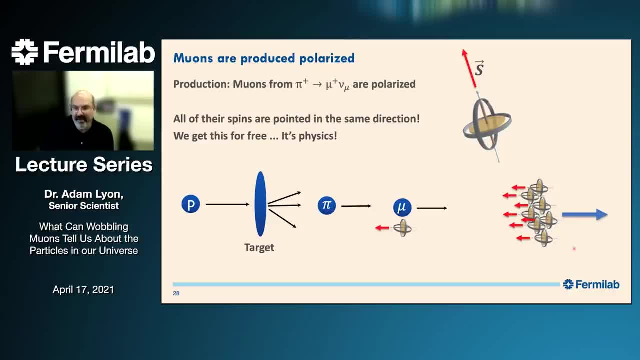 Robert Alverson- of a Robert Alverson- direction the muon is going, and so we can make a beam where all the muon spins are all pointing the same way, Robert Alverson- And this is called a polarized beam. and this is a really key if, if we had randomized. 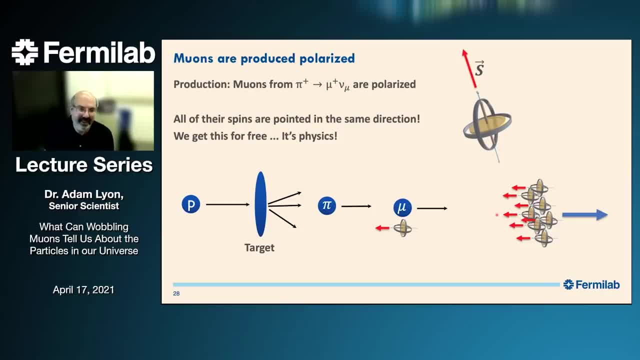 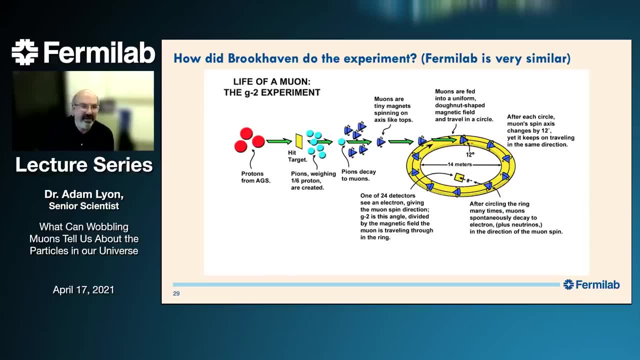 Robert Alverson- spins directions. that wouldn't work. we need all the spins pointing in the same direction and we get that. but it's hard not to get that with pions, Robert Alverson-. Okay, so the muons going to go into the storage ring, so here. 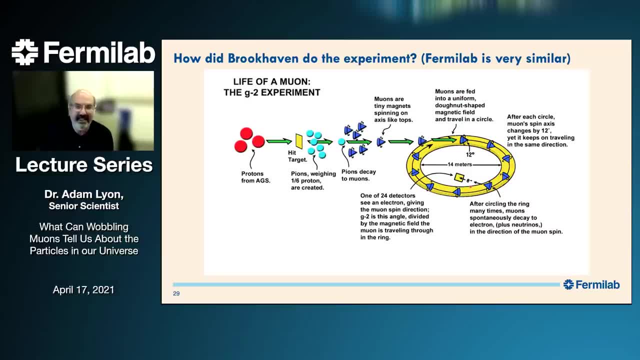 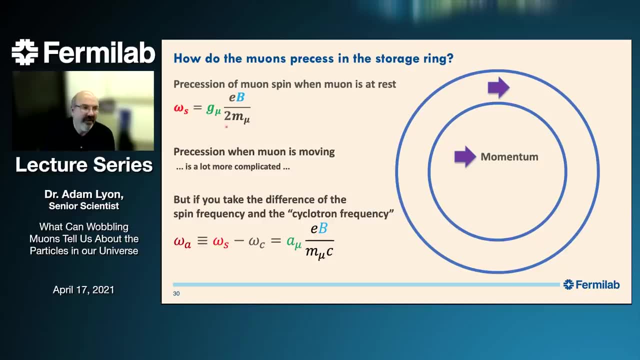 Robert Alverson- And they go around and and their spins process as they go around, Robert Alverson- The storage, Robert Alverson- ring. so let's look at that, Robert Alverson-. So remember, here's our, our, our little formula for relating the spin procession frequency: how fast the spin is processing around, how many times around a second. 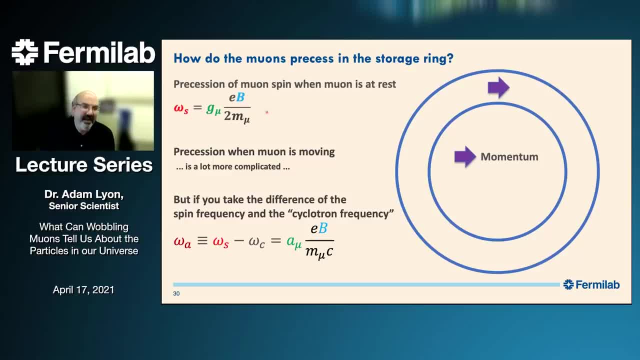 Robert Alverson- it's related to the G factor and the magnetic field. this is when a muon is at rest, Robert Alverson- But these are muons are moving, they're going around the storage ring. here sort of a top down view of the storage ring or a little racetrack. 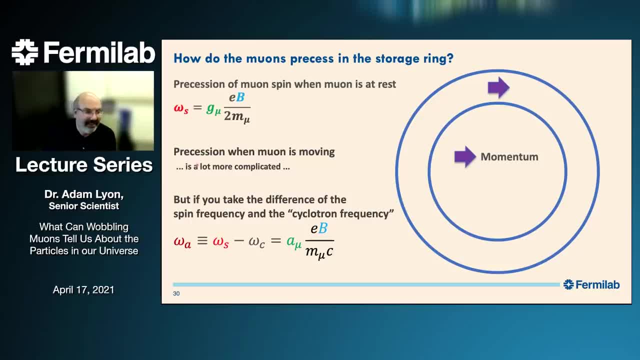 Robert Alverson- And this. this formula is a lot more complicated, I will- I won't scare you with it, Robert Alverson- But there's a really neat thing that does happen: that if you take this formula for the spin frequency and subtract off what we call the cyclotron frequency, 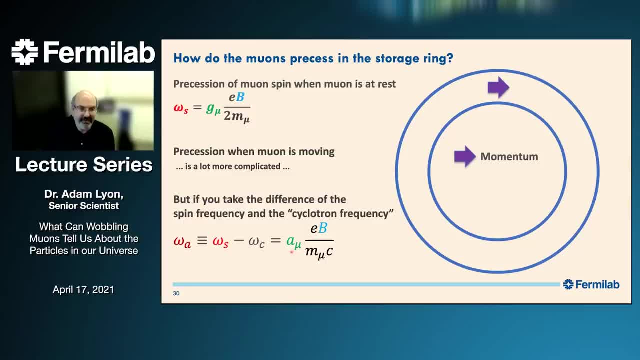 Robert Alverson-. Then we get this frequency called a mega a, which is directly related to the anomalous part of the G factor. so all we need is the measures up to know the magnetic field really well, some constants and this frequency, and then we can measure what this anomalous part of the G factor is, or how much of it is bigger than two. 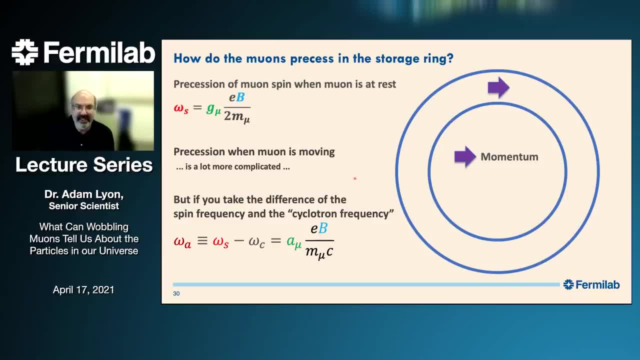 Robert Alverson- And so what we do? Robert Alverson- And so what this cyclotron frequency is? it's just how just the rate at which the muons go around the ring. and so we imagine this has a vector called the momentum, and this momentum vector spins. 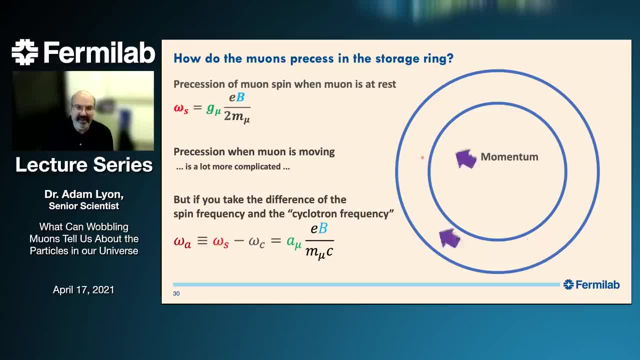 Robert Alverson- Just in the direction that the muons going around. so just goes around in a circle, and so if you just look at the vector itself, this is what it's doing, Robert Alverson- So this goes around. it's just pointing in the in the direction of the new one. that's all that it does. so nothing, nothing, nothing interesting there. 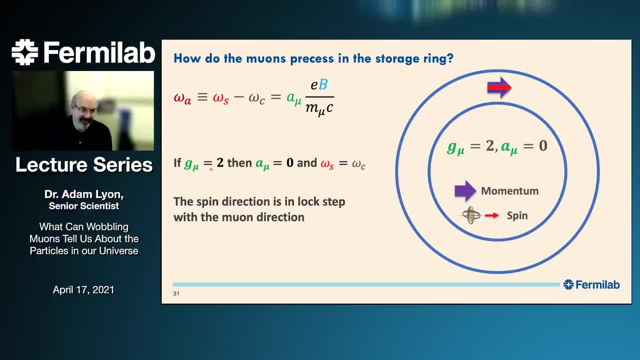 Robert Alverson- So let's let's play some games. so, Robert Alverson- If G is exactly equal to that, means that a zero right and the spin processor frequency is a cyclotron frequency, Robert Alverson-, And if that were the case, then i'll show you here. then the spin vector, which is in red, is in lockstep with the momentum vector, so as 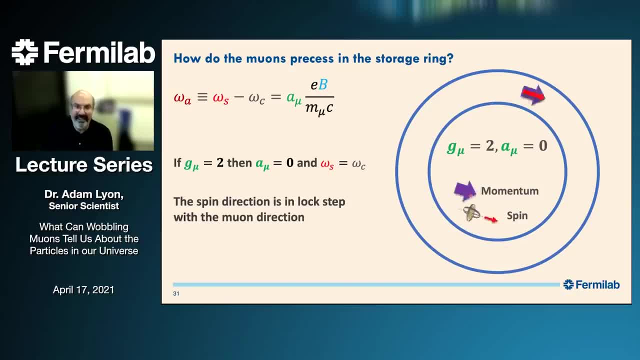 Robert Alverson- The new one goes around the ring and the direction points in a different direction. is it goes around, the spin direction follows that in lockstep, Robert Alverson- Okay. so now let's say G is a little Robert Alverson- greater than two, which of course we know that it is. so that means that a mu is a little bit more than zero. 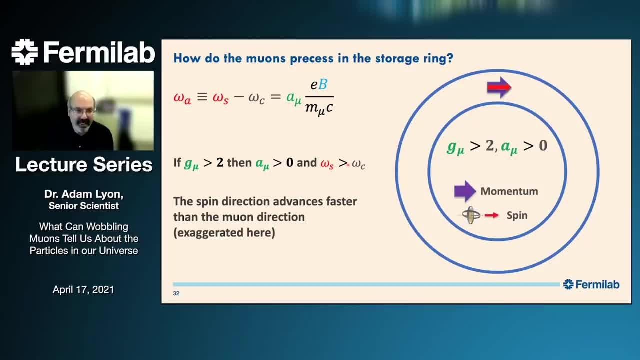 Robert Alverson- And so that means that the spin processor frequency is a little bit greater than the cyclotron frequency, and so that means the spin vector will advance a little faster. Robert Alverson- And that's what's shown here. notice that the spin is not getting out of sync with the direction. I don't. I don't work in the middle ones, because that that that will make you nauseous. 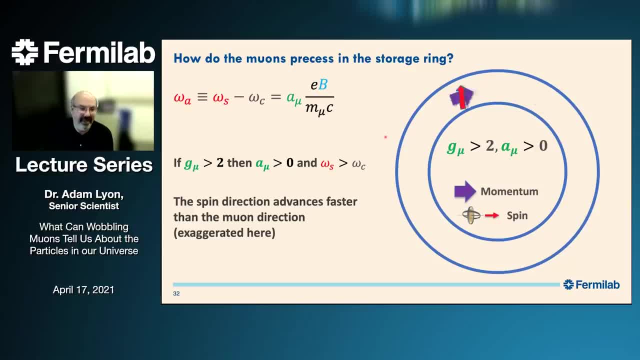 Robert Alverson- And you can see, sometimes it's forward, sometimes it's backwards and in between it's actually- I exaggerated here for Robert Alverson- The value of G minus two for the muon. it takes 29 times around the ring for the spin vector to go all the way around once. 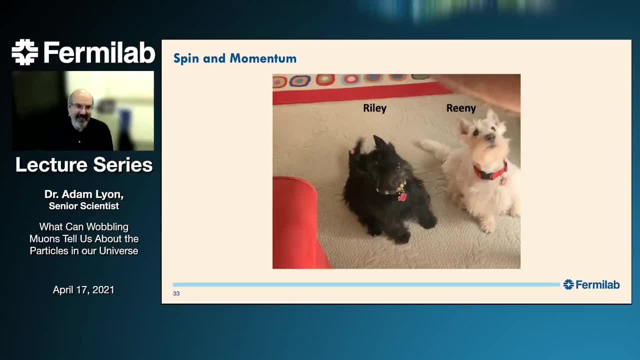 Robert Alverson- let's let's try to hit this home a little bit more. i'm going to get two friends to help us. these are our two doggies, Riley and Rini. we adopted them about seven months ago. and so, Robert Alverson- So G is equal to zero. actually going to do this, we're going to rename them spin and momentum just for this talk. and so if G is equal to zero, spin and momentum should rotate around the same rate. 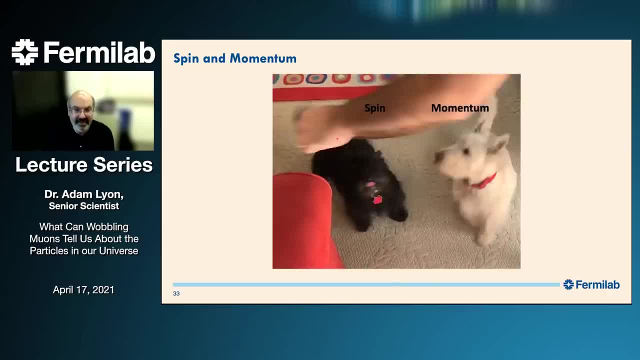 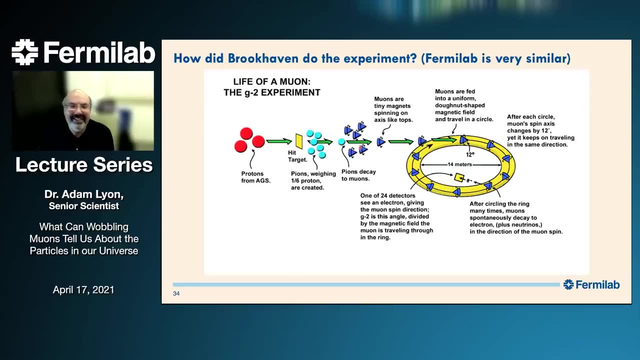 Robert Alverson- And hey, they did. and if G is a little greater than two spins a little faster. okay, we're still working on it. hopefully, maybe by the next result from G minus two we'll have all that figured out. so anyway, Robert Alverson- So these muons are, the spin is processing if G is greater than two is processing at a faster rate than the muons are going around the ring and then the muons decay. 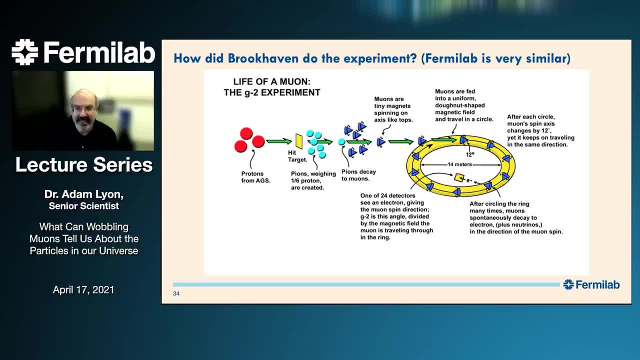 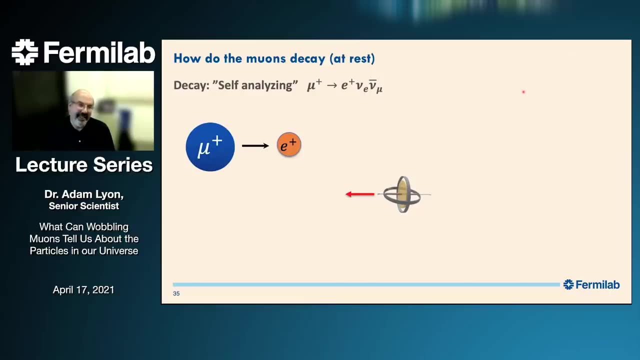 Robert Alverson- The muons. we have positive muons, so they decay to positrons or positively charged electrons, Robert Alverson- And then Robert Alverson- We can catch those electrons in a detector called a colorimeter, or those positrons in a colorimeter and measure their energy. so let's see how that works. and there's another really neat thing that happens. 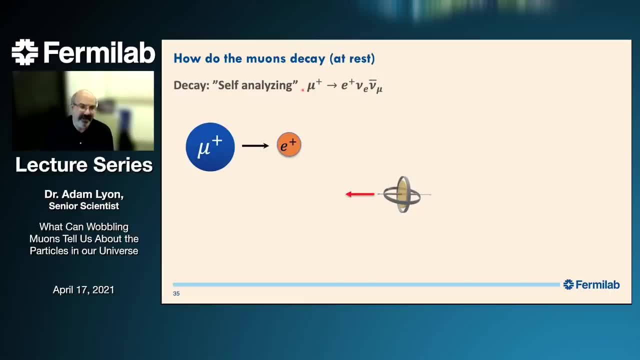 Robert Alverson- Because of the weak force. so imagine so i'll use. i'll start first. start out with muons at rest, and so muons will decay to a positron and more neutrinos. Robert Alverson- Lots of neutrinos are being produced here that we don't care about. they just go on their merry way and we never seen them. we care about the positron. 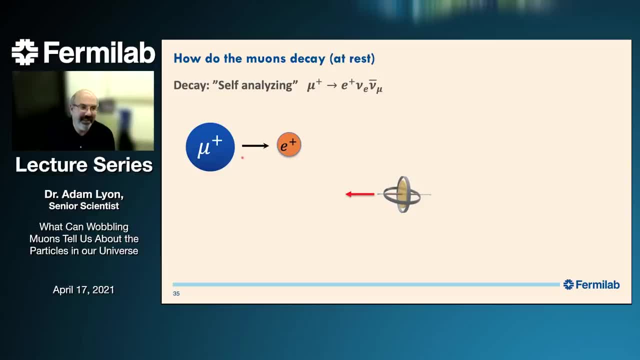 Robert Alverson- And the really neat thing is that, Robert Alverson- The way the weak force works is that the positron, when it is admitted from the muon, the highest energy positrons are emitted along the direction of the muon spin. 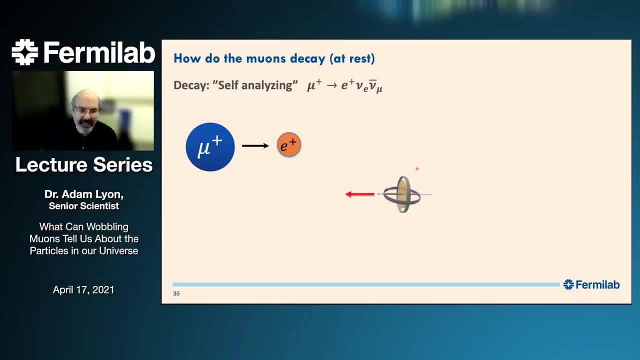 Robert Alverson-. So here is our little gyroscope. here's the direction that the spin is pointing. if this muon were to decay to a positron, the positron will come out in the direction of that spin, Robert Alverson- So here's another. one comes out in the direction that's been. one more comes out in the direction of that spin. 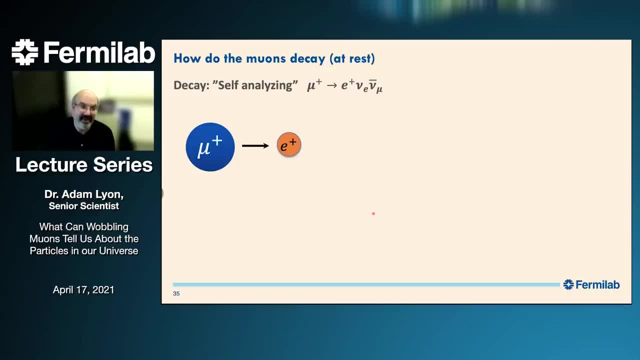 Robert Alverson- Right, so that's really neat. that means that, Robert Alverson- This Robert Alverson- positron is carrying information about the spin of the original muon, right? so by looking at these positrons, we can get information about the spin of the muon that it came from. 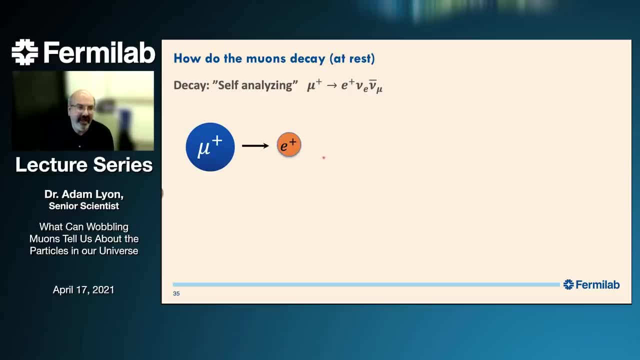 Robert Alverson- Right, so we can actually see this. then procession of the muon spin through these positrons. I hope that made sense. Robert Alverson- we're actually go a little bit further, because that was for a muon at rest and our muons on the storage ring are moving and they're moving fast, they're going, you know almost. 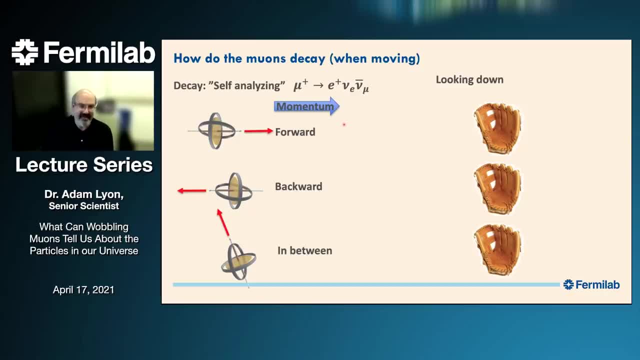 Robert Alverson- Almost the speed of light. and so what happens then? is that basically the direction that the muon- that the positron Robert Alverson- is emitted is always along the same direction as the muon? muon is going so fast that it basically it's like throwing a ball from a fast moving train- right if you're on top of the training and throw a ball. 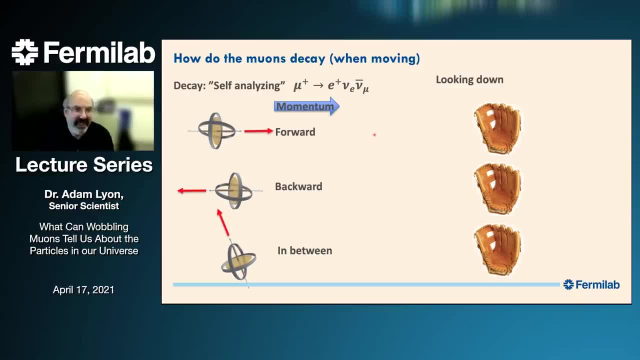 Robert Alverson- That ball is going to speed of the train, because the speed of the train is overwhelmed. Robert Alverson- However fast you throw the ball, but that the ball, or in this case the positron, will get a little boost of energy, either a boost or kind of an anti boost. 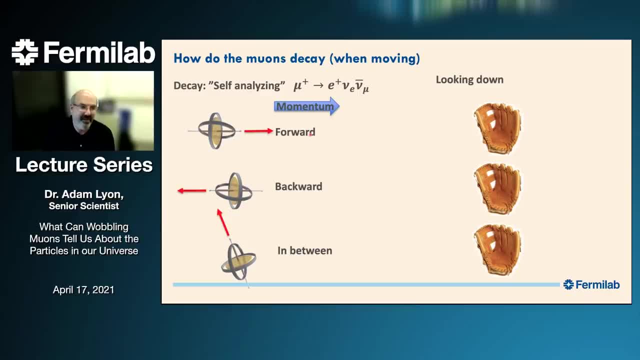 Robert Alverson- Depending on if it's thrown off along the direction of the muon or in a different direction. so, Robert Alverson- So we have these. these detectors are called calorimeters, which I represent as a catcher's mitt. Robert Alverson- So the catcher's mitt will catch the positron and it'll measure how much energy that positron has and sort of how hard it hits that catcher's mitt. so 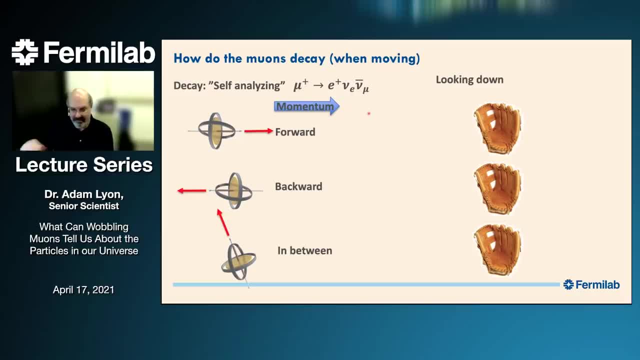 Robert Alverson- If the spin is pointing in the same direction as the muon momentum, so the spin is pointing along the direction the muon is traveling in. Robert Alverson- That positron will hit the calorimeter and the calorimeter will. 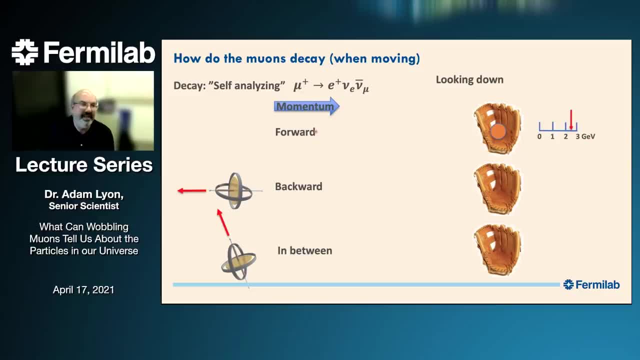 Robert Alverson- register really high energy, that that that positron is getting a boost from the muons motion and muons direction. Robert Alverson- If the positron is emitted in the backwards direction, so backwards from from the direction that you want to traveling in, it'll get a boost to. 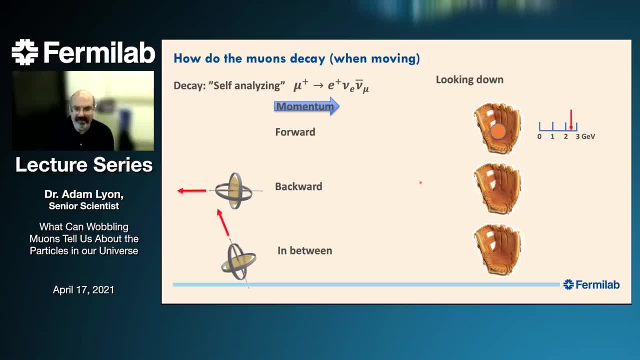 Robert Alverson-, Because the muon is still moving from left to right, but it'll get a little bit less of a boost, and so the energy that is registered by the calorimeter will be a little bit less- Robert Alverson- than what it was in the forward direction. 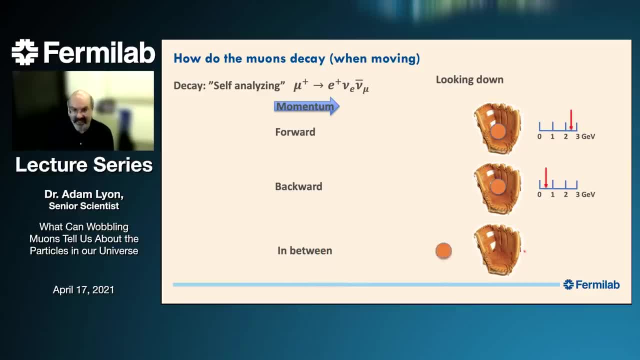 Robert Alverson- And if it's Robert Alverson- In between. still, the positron always comes out, you know, in the direction of the muon, because it's overwhelmed by that. but now, but the energy that the calorimeter 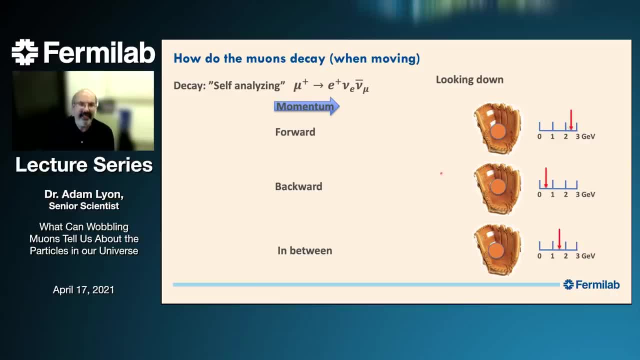 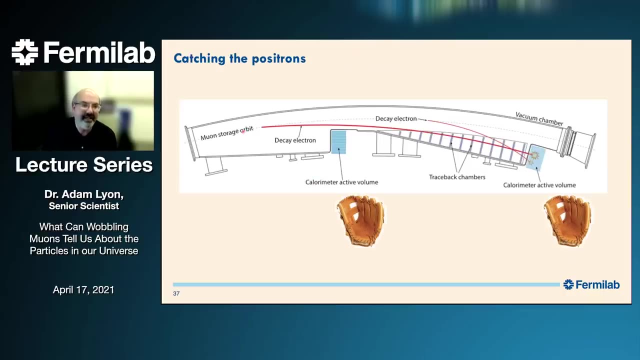 Robert Alverson- registers will be in between the lowest and the highest, so from this you can sort of see this picture of you. know how we can maybe measure? use this calorimeters to measure the positron energy- Robert Alverson- To get information about where that muon spin vector was when it decayed, and so the way this actually works. here here's a piece of our storage ring. 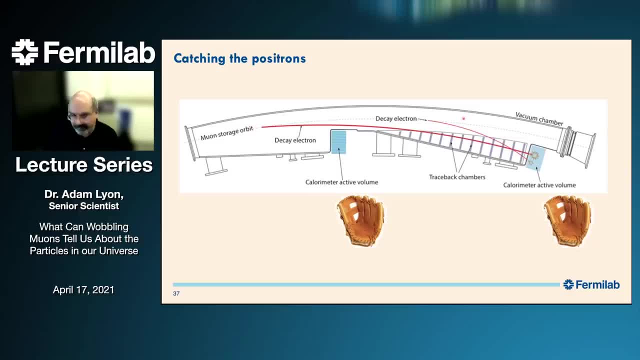 Robert Alverson- This dashed line here is where the muons actually go, so they're going around the ring. the muons will decay to a positron. Robert Alverson- The positrons actually are lighter and a little slower than the muon, so they curl inward. 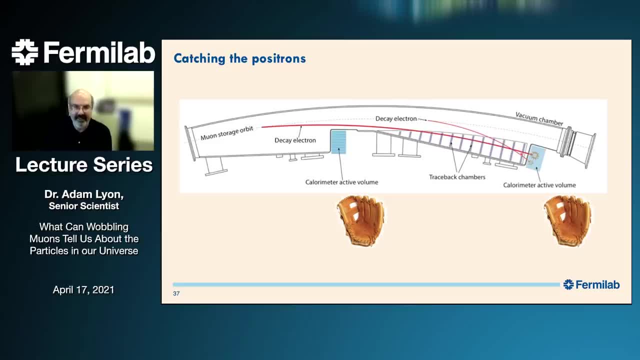 Robert Alverson- Out of the sort of the point, out of where they should be in the in the next storage ring. the storage ring is not set up for positrons and set up for muons, so it'll curl inward and it'll eventually hit our catcher's mitts or our, our calorimeters and sometimes 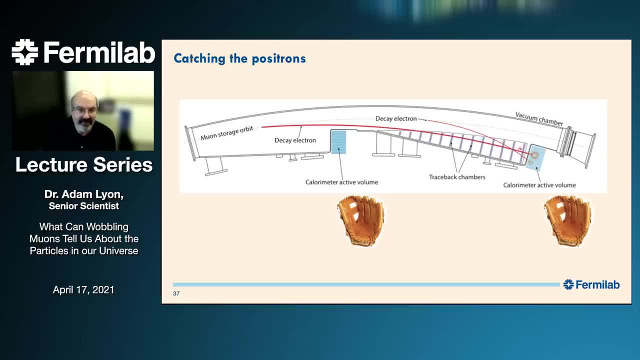 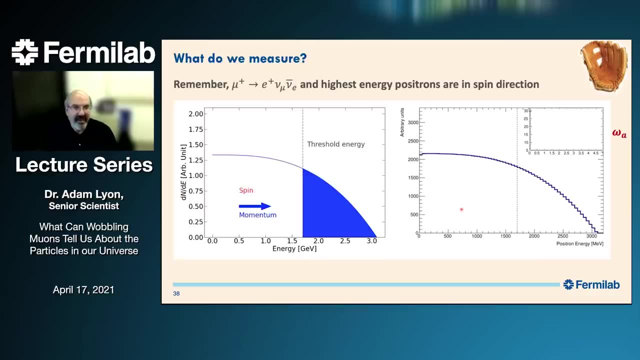 Robert Alverson- They can go really far into the catcher's mitts and sometimes they don't go very far at all and that depends on kind of where the spin vector was when the muon decayed. Robert Alverson- So more complicated and more complicated picture. I showed you sort of one positron at a time. it's actually not what we get. we get lots of positrons and they all have an energy distribution. 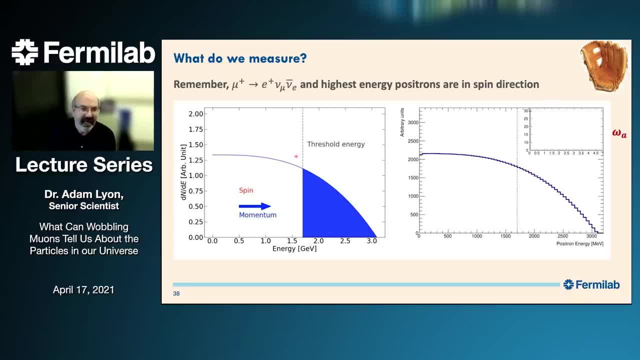 Robert Alverson- So this sort of shows what the energy, energy distribution is. Robert Alverson- Here I should kind of show a threshold energy where we're going to look at how many, how many positrons come in. Robert Alverson- Above. 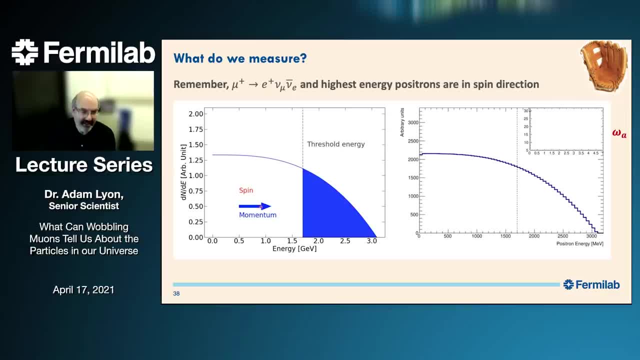 Robert Alverson- This energy. and so when the spin and the spin vector and momentum are aligned, then this spectrum is pushed really high because, right, because the, the positrons, get a nice boost- and i'm going to see if I can, Robert Alverson- control this here a little bit- and so as the spin vector turns around, so here i'm going to stop it and go, oops. 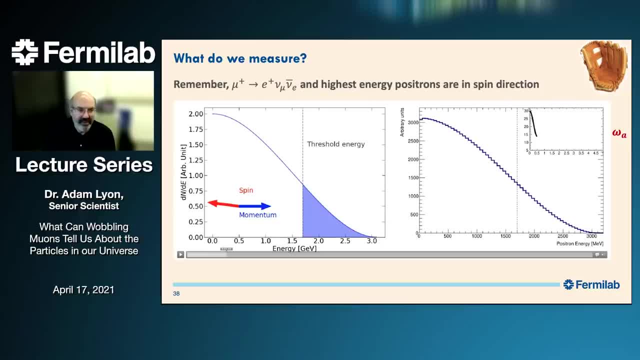 Robert Alverson- I knew that. there we go, there we go. so it's backwards- notice that the energy spectrum is lower above the threshold. and it's pushed to the left, Robert Alverson- And it gets higher and higher and higher. and when it's aligned, it's the highest, looking at the left picture here, and then when it's anti aligned, is the lowest. 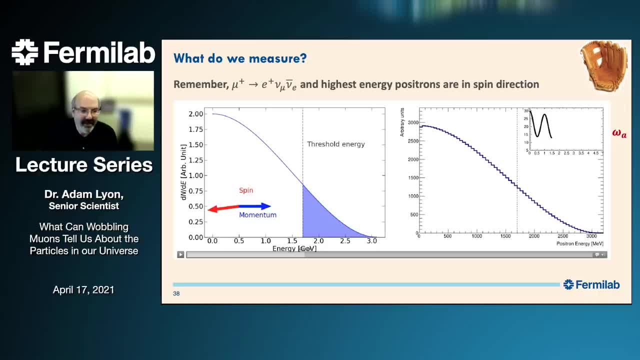 Robert Alverson- And and so this oscillates right. so now on the right hand picture, i'm going to go back to the beginning and stop it, Robert Alverson- On the right hand picture, we're now counting these positrons over this threshold energy, and i'm going to plot how many of these we see. and so, when the spin and momentum are aligned, 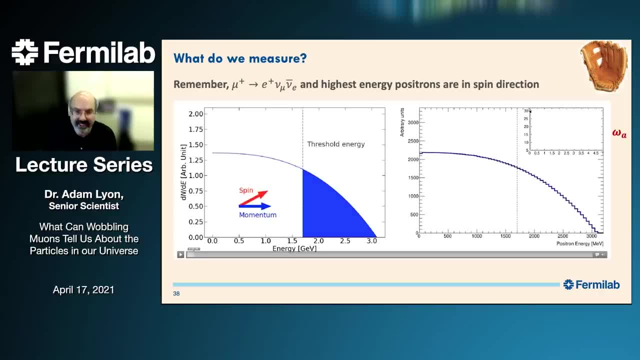 Robert Alverson- We see a lot. it's, that's a 30, it's really high. Robert Alverson- In the upper right inset plot. and then as it gets anti aligned, it gets low and then it gets higher again, Robert Alverson- As it comes alive and then lower and it gets anti line and then higher again when it's aligned. so hopefully that makes sense. let's let the drone, and so we build up what's called the wiggle plot. 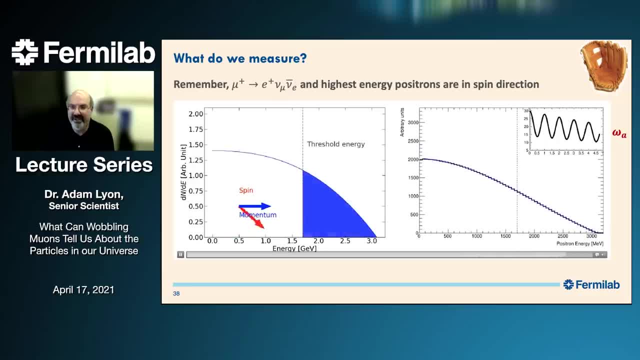 Robert Alverson- As these new ones are going around the ring, their spins are processing, they're shooting out positrons, and that positron energy depends on where the spin vector is. Robert Alverson- And we can tell where that is by basically measuring. 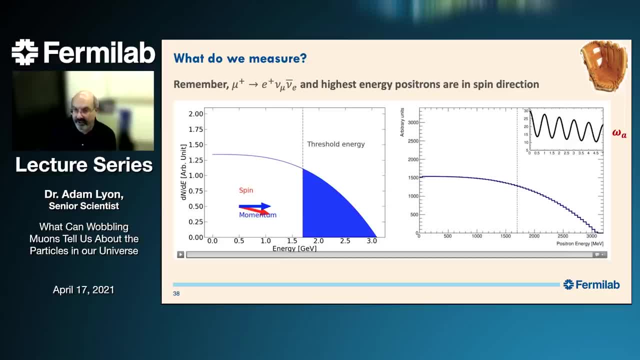 Robert Alverson- How many new, how many positrons we see over this, this threshold, and we see this oscillation. Robert Alverson- Remember this oscillation? the frequency of this oscillation is a mega a and that's directly related to the anomalous part of the G factor. so we can measure G minus two. 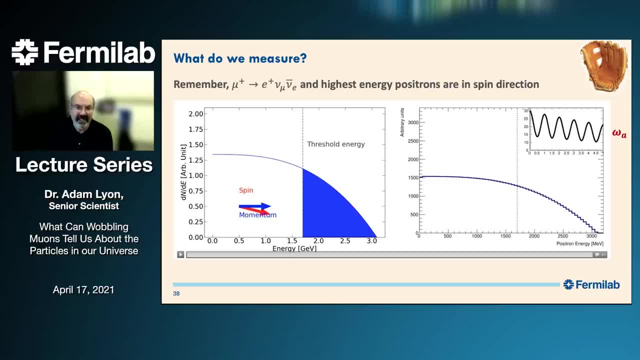 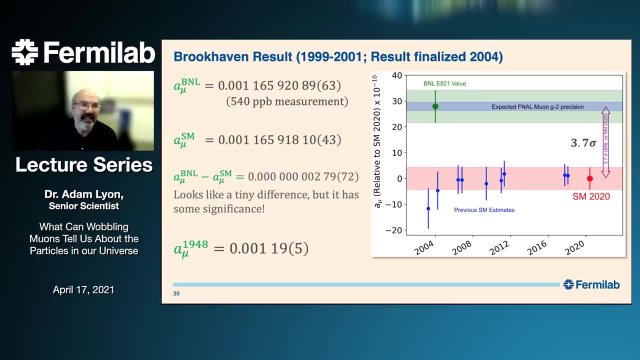 Robert Alverson- By looking at this, this frequency of these oscillations, and that's basically how this experiment works. Robert Alverson- Okay, so if that wasn't clear, I can talk about it more, more at the end. Robert Alverson- And you can ask me questions. 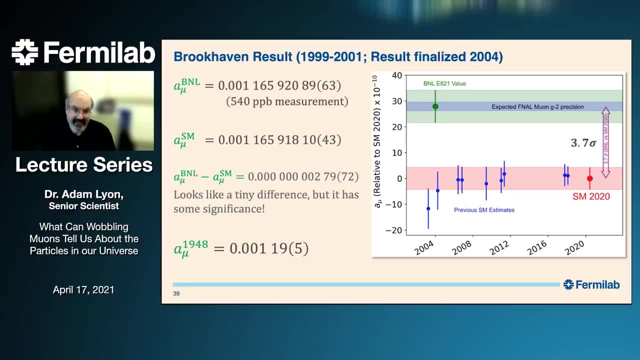 Robert Alverson- about it. so so brookhaven did this experiment and and collected billions of of positrons and made their wiggle plot. i'll show the one from friendly lab a little bit later. and so they came up with a result for the anomalous part of the G factor and it's 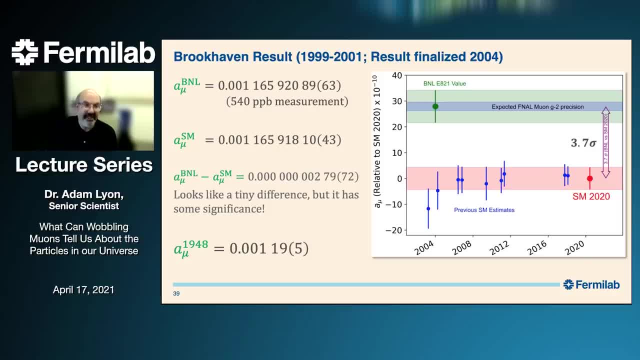 Robert Alverson- Lots of digits here, with a of the error and the last two digits which is really really far out. compare that to the kitchen foley number from 1948.. Robert Alverson- You know, and to see how much, how much more precision we have. 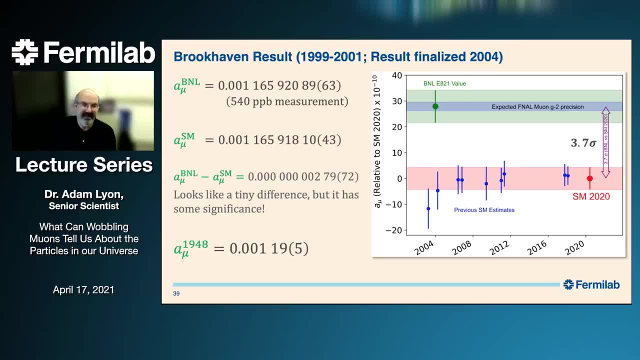 Robert Alverson- Compared to what they had. we have the standard model value and then we can compare. take the difference, Robert Alverson- And that makes this this gap here. here's where the brookhaven result is, but their error bar, that's the error here. and we call this a 540 parts per billion. 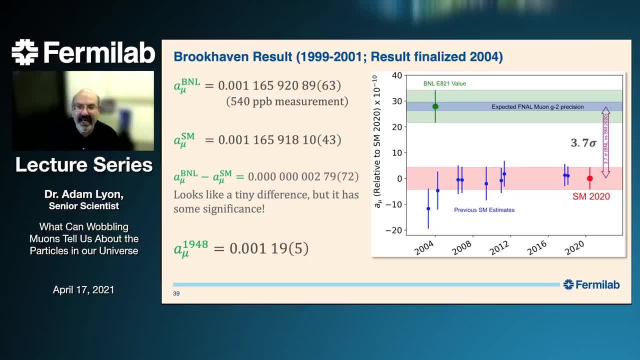 Robert Alverson- measurement, that's the precision and i'll talk about that in a second and that makes for this gap and we can characterize the sort of the significance of this gap in standard deviations or Sigma, and it's 3.7 Sigma. 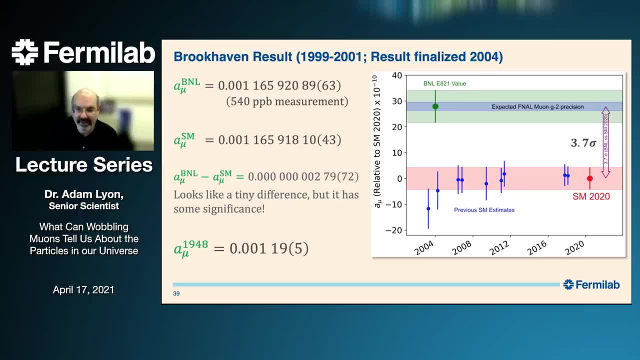 Robert Alverson- If the error bars were smaller, if this error were improved and this would get better, this would get larger, Robert Alverson- And so that's why actually framing I was going to try to do, but this is 3.7, the gold standard for discovery is five Sigma, and so they don't. so doesn't quite meet the level of discovery, but certainly very, very interesting. 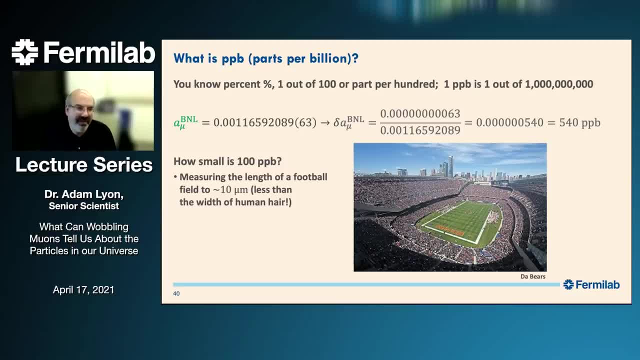 Robert Alverson- Actually, just to give you a sort of hint of what a part per billion is, you know what a percent is. that's a part out of 100, and a part per billion is a part out of the billion, Robert Alverson- So basically, the way we calculate it. 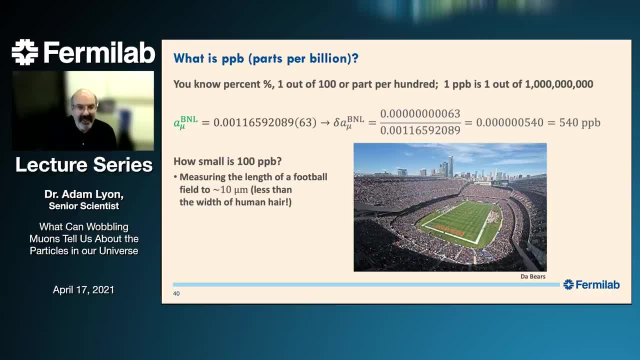 Robert Alverson- is very simple. you take the uncertainty which is in this, these last two digits. you divide that by the measured value, and that's the and that's the result, and you multiply it by a billion and you get the parts per million. 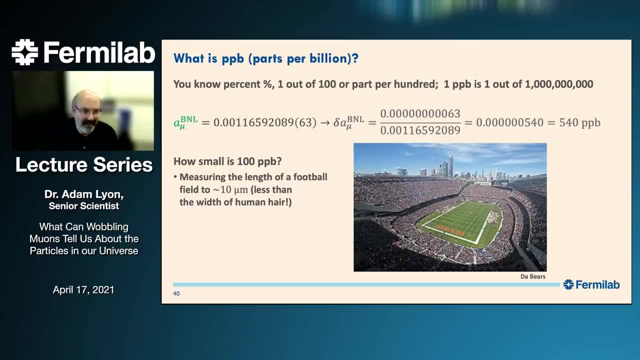 Robert Alverson- So how, how precise is this? so if you pick a nice round number like 100 parts per billion, Robert Alverson- that's equivalent to measuring the length of a football field to about 10 microns or less than the width of a human hair. so so that's really really, really. 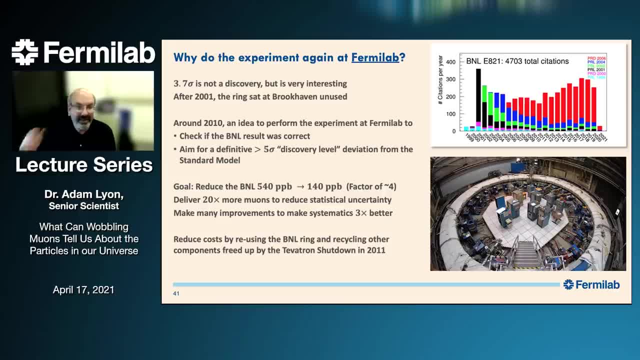 Robert Alverson- Very precise. so that gives you some picture of Robert Alverson- The precision- Robert Alverson- Of these experiments. Robert Alverson- Okay, so, so. so brookhaven got their result. they got a 3.7 Sigma discrepancy. so not a discovery, but also very interesting. 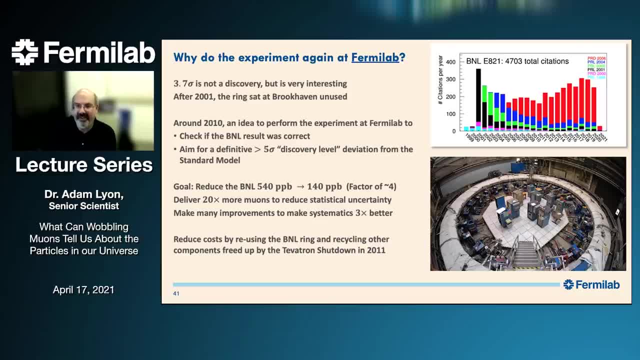 Robert Alverson- And actually this is generating an enormous amount of interest. this plot shows the number of citations to the papers from brookhaven and over the years- and I really has been sustaining for a long time, Robert Alverson- But for brookhaven to make big improvements to this would have been very difficult, and so brookhaven does a lot of other things, and so they stopped working on G minus two. 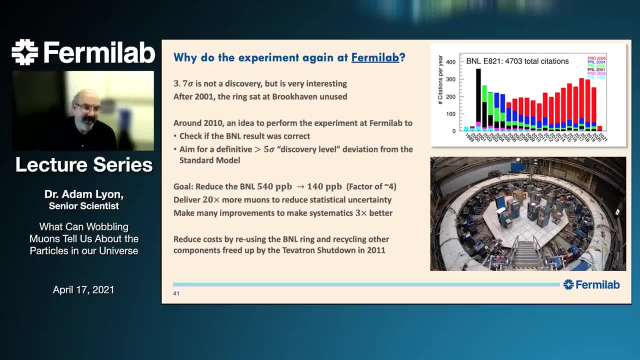 Robert Alverson- And the ring sat for quite a long time at brookhaven and then around 10 years ago or so a little more at Fermilab. some people started to get the idea that Robert Alverson- You know, this is. this is so interesting that maybe Fermilab should, should do the experiment with a lot of improvements to first check to see if the brookhaven result was right. would we get the same result to where we get something different and aim for this five Sigma discovery level? 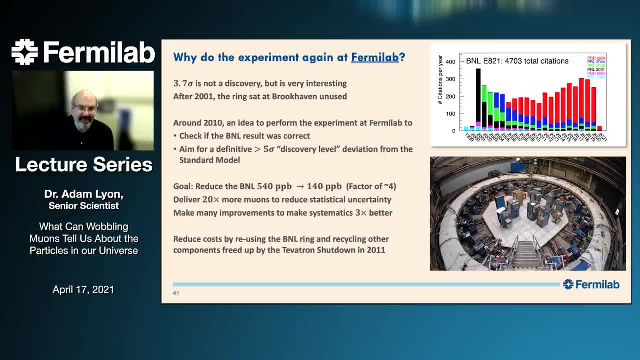 Robert Alverson- You know. so if we do see the same deviation that Robert Alverson- That brookhaven did, by the time we would be done, we would have an undeniable signal of new physics, if in fact that that that really happens. 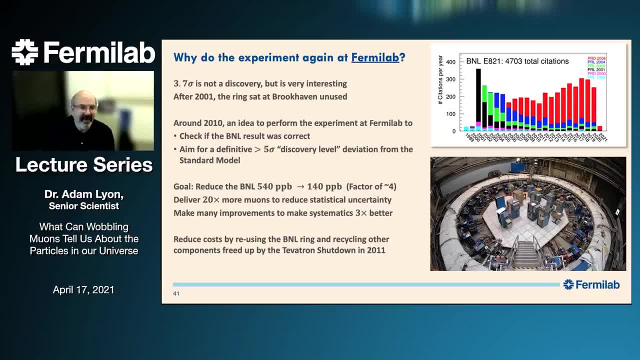 Robert Alverson- So the goal is to really do this experiment here again at Fermilab with a factor of four in Robert Alverson- Better precision- and that involves delivering 20 times the muons that brookhaven saw here at Fermilab. so we need 20 times more muons. we have a very powerful accelerator accelerator complex that can actually do that. 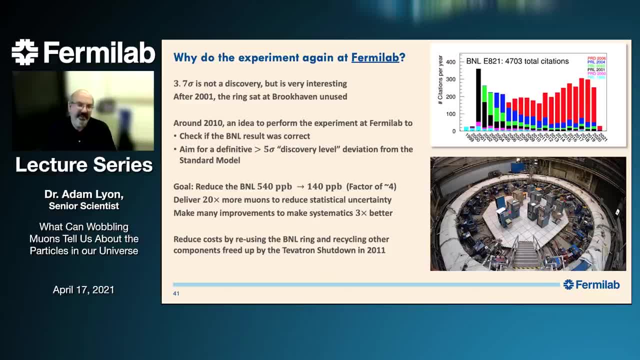 Robert Alverson- And also make many improvements to basically do the experiment three times better, in terms of what uncertainties, of how well we do things and and things that can that maybe, Robert Alverson- You know we have to be very careful about do those things three times better to really improve this error, this uncertainty, and also to try to reduce our costs by reusing, as 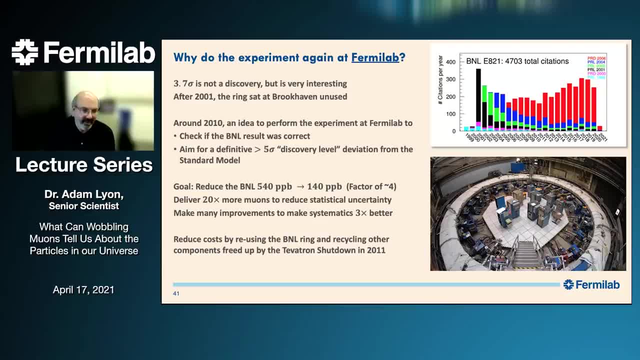 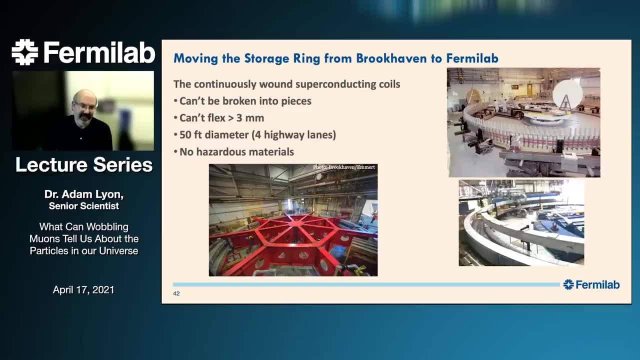 Robert Alverson- sort of the big parts and expensive parts of the experiment from brookhaven and also other components that were freed up when the tevatron slider shut down at Fermilab in 2011.. Robert Alverson- So we've actually recycle a lot of stuff from from the tevatron. 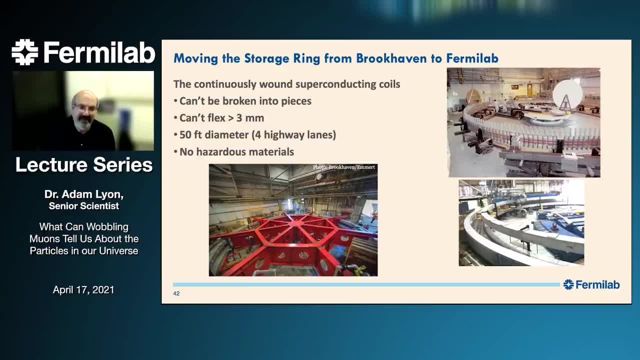 Robert Alverson- Okay, so moving the ring from brookhaven to Fermilab, that was an amazing thing. so first of all, the ring is made up of coil. so here's two coils, Robert Alverson- Top and bottom, and then as a coil on the back, those are continuously wound wires of niobium wire that they're superconducting, so that makes the magnetic field. 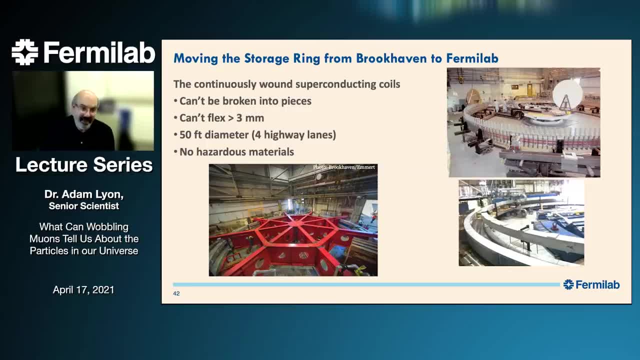 Robert Alverson- And they go all the way around and we can't break them. if we break out, we gotta make a new magnet and that's really expensive. we also can't, Robert Alverson- They have to be. they have to be very長 to unlock these things- more than about three millimeters. and these rings themselves are big. they're 50 feet in diameter. So if you stick it on a highway that takes about four lanes of a highway, so they're not easy to drive around. 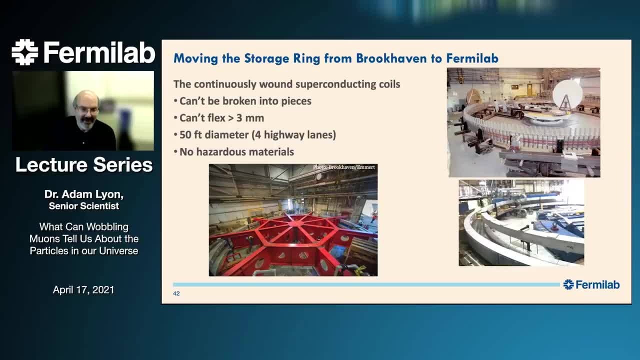 Robert Alverson- Fortunately they're not. there's nothing hazards about them. so. so that's since it's easy. but they're big and they're very fragile. so we contracted with a company called emmerich to move the reign from. from Robert Alverson- brookhaven. 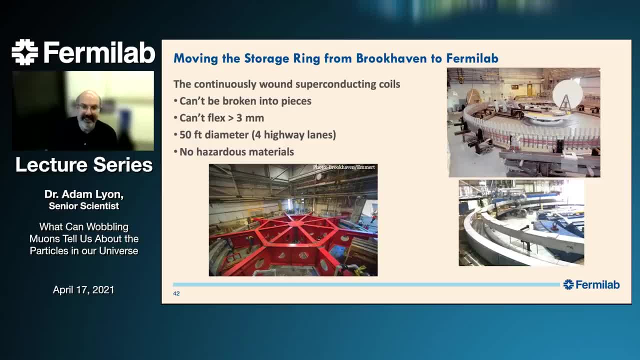 Robert Alverson- From lab. and so, Robert Alverson- They built this, Robert Alverson- gigantic frame. Robert Alverson- that the back coils sit in. you can kind of barely see them here. the next slide will be better. 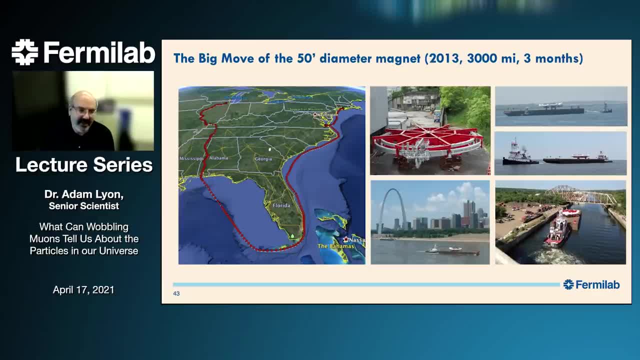 to really rigidly hold these coils so that they would be very, very, very protected. And then we put the ring on a barge, we slid it out of the building at Brookhaven, put it on a barge and basically drove it on the barge down the eastern seaboard, around Florida, up the Gulf of. 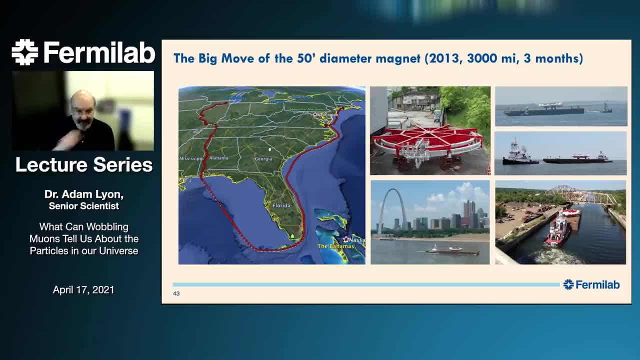 Mexico to Mobile, Alabama, where the Tennessee Tom Bigby waterway, where that entrance is, and then up there eventually hit the Mississippi and then on to Illinois. And so this was an amazing, you know- water journey for 3,000 miles. It took three months. We've got some really neat. 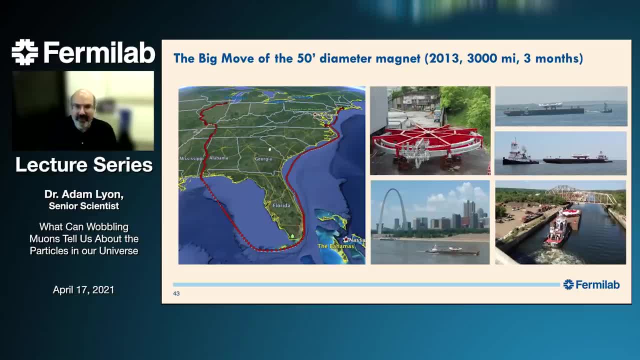 pictures: Here's where the ring is being handed off from the ocean tug to the river tug, And here it is going by the St Louis Arch. And then here it is, arriving in Lamont, which is the about 30 miles from Fermilab, which was the closest point on the Illinois River, where the 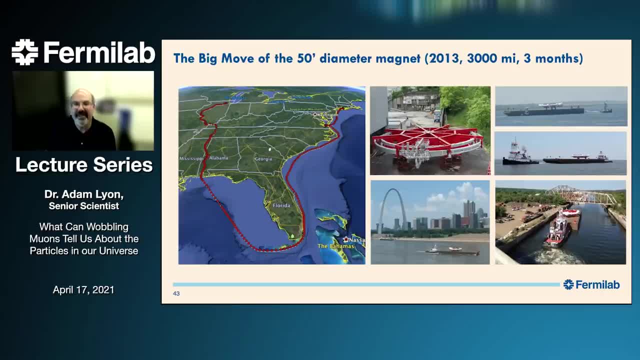 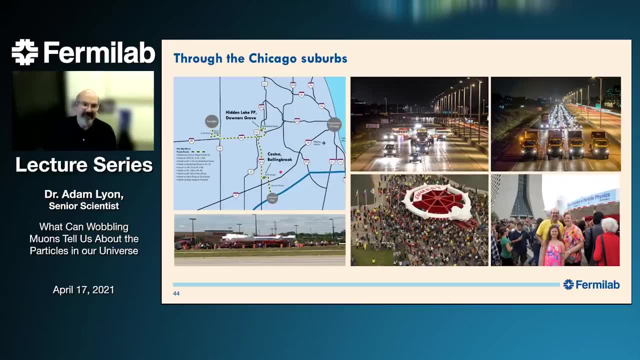 magnet could be offloaded from the barge. So then the magnet was still 30 miles away from the lab down here in Lamont, And so we had to drive it across the Chicago tollways, the highways in the suburbs, from Lamont to Fermilab. We did that over three nights. 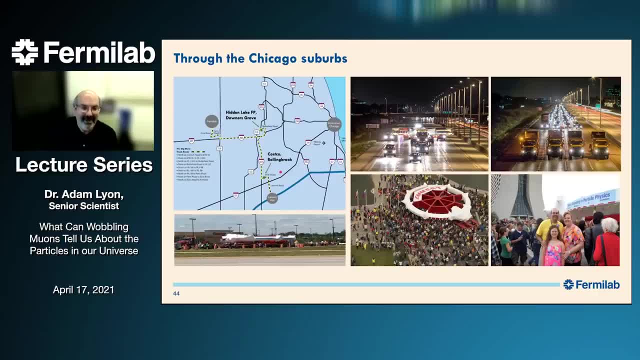 So here it is actually on Interstate 88 with all of its support traffic. I always like to go to the interstate 88. I like to go to the interstate 88. I like to go to the interstate 88. I was actually. I was very lucky I was in a car following the ring. It was really. 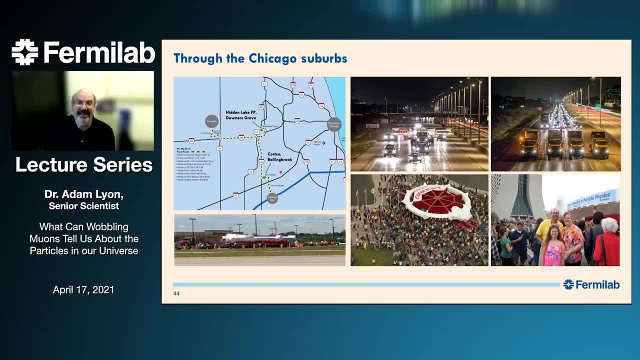 really cool. And then behind us the traffic was stopped. I'm sure they were not very happy, but you know all in the name of science And actually during the day in between these moves the magnet would sit, And so it actually sat across the street from a Costco and a bunch of us brought 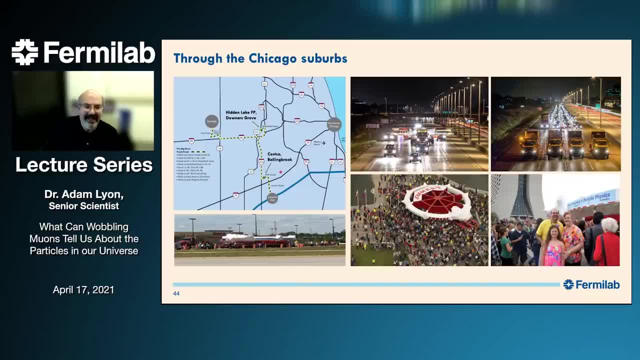 some brochures and talked to lots of people. It was really neat. And then it arrived at the lab and we had a big celebration. We opened the lab so that people could see it And actually we had no idea how many people we would get And it turns out thousands of people came. In fact so many. 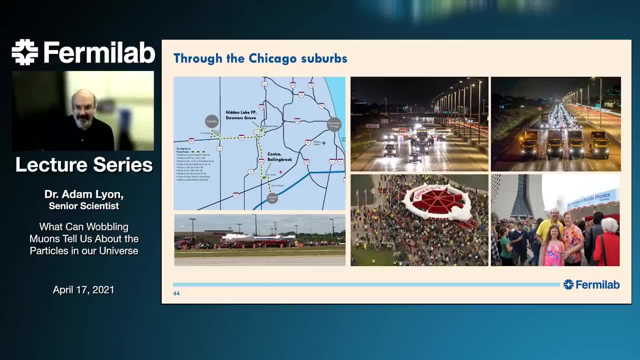 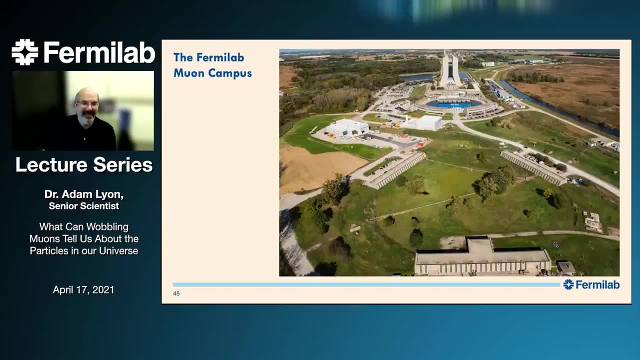 people came that we had to eventually start turning people away. We ran out of parking. So it was an amazing thing, And here's my family in a photo op in front of the ring. A lot of people did So. eventually we built our building that the ring goes into. 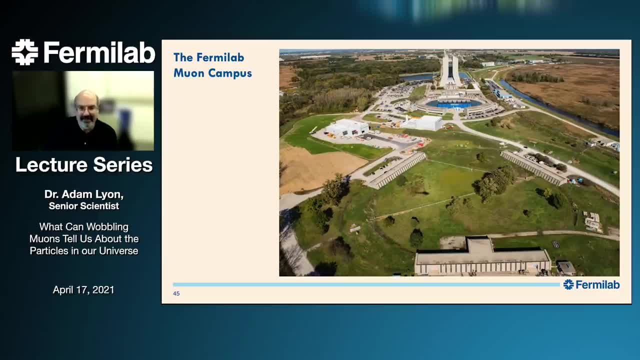 and we call this area the Muon Campus. So this is: this will support our experiment G-2, and another experiment that's under construction called Mu2E, And this part down here is where is part of the delivery ring where we deliver Muons to this. 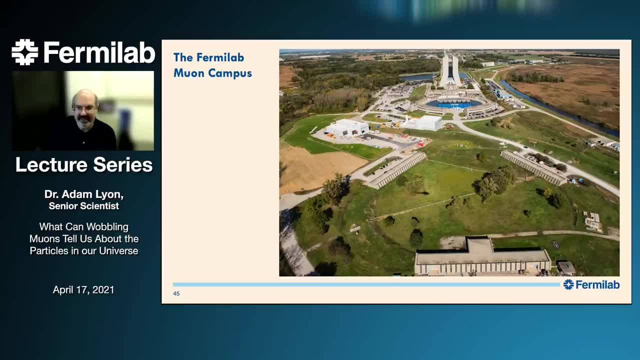 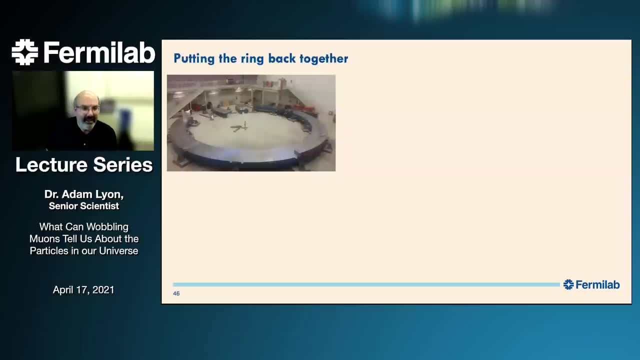 campus And that's actually recycled from the Temetron. This is the old Temetron anti-proton source, And here's our two buildings, And so here's just a couple of slides putting the ring back together. So we have this base of iron, This, actually this comes in pieces, And so we trucked. 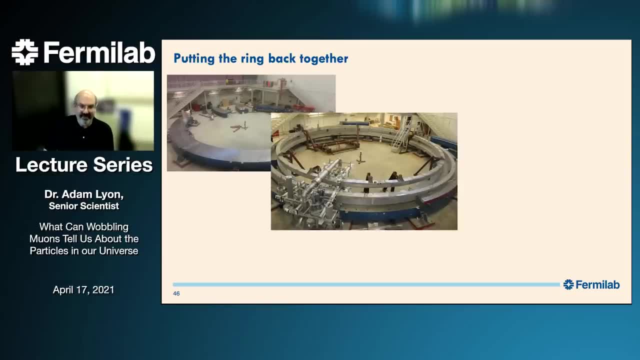 that from Brookhaven. Here's the ring itself now sitting on top of it. We can slide it into the building. The front of the building comes off, And then we can slide it into the building. The front of the building comes off, And then we can slide it into the building. The front of the building comes. 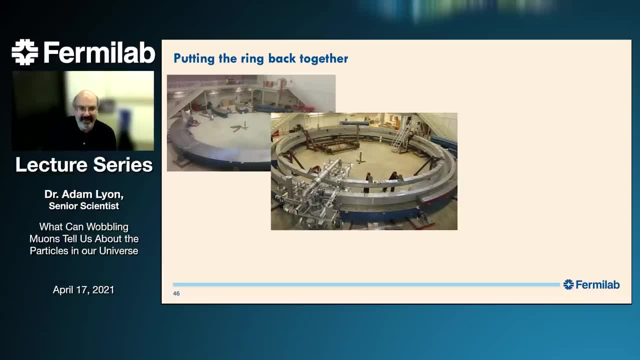 off And then we slide it in and then we lower it onto this platform And then we build up more iron that also got shipped by truck from Brookhaven And this actually forms the magnetic field. Here are the, here are the two inner coils, And then muons kind of go in this inset region. 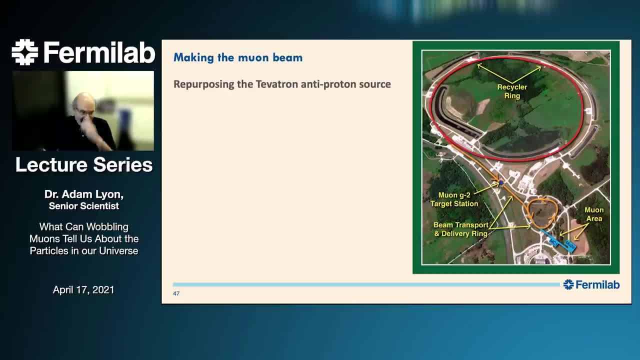 in between the two coils. So that's what that looks like. I talked briefly about how muons are created, So we do something sort of similar to what Brookhaven does does. uh, we have uh rings and accelerators that accelerate protons. they're very high energy. 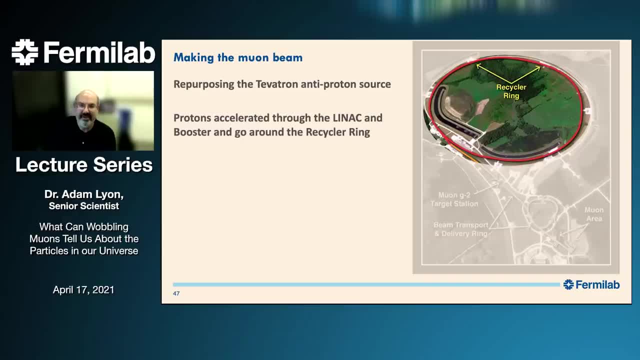 so protons from our accelerator complex eventually make it into this ring called the recycler ring. that kind of reorganizes the bunches of protons, uh, and sends them to a target station. uh, so that's our big block of metal. we have a cylinder of nickel, nickel alloy that the protons hit about. 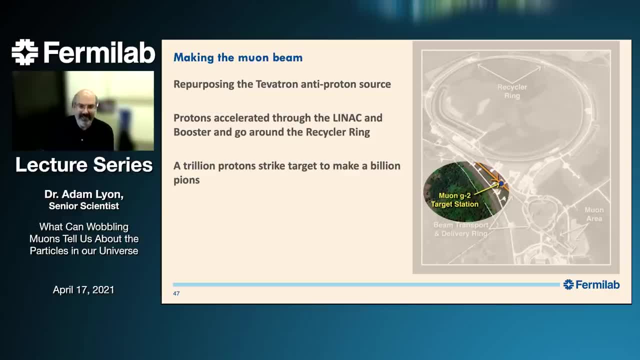 a trillion protons uh at a time hit this target and there are 16 bunches of protons in about 1.4 seconds, so each bunch has about a trillion protons. they hit this target. a whole lot of other stuff comes out the other side, as i mentioned before, including pions, uh. and these pions, remember they? 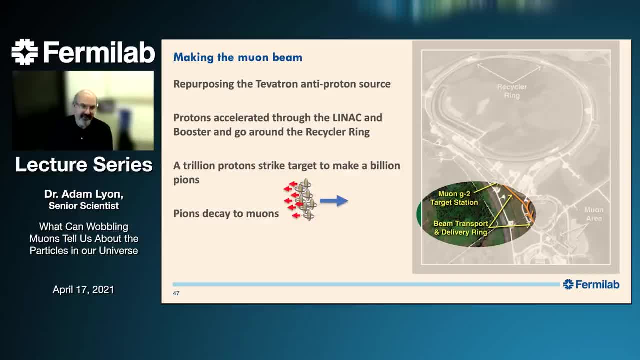 decay the muons. there's a beam line here where these pions will decay. remember, all these muon spins are pointing in the same direction. it's a polarized beam. uh, so that's. that's, that's what these muons go around, this delivery ring. that was sort of those three bunker buildings that i showed. 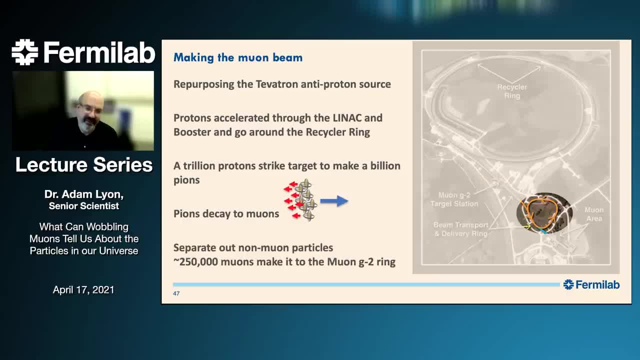 you before, and they go around this ring a couple times, four times typically, and that's because there are other particles that are coming along with muons and we don't want those particles, we don't want them hitting our ring because they'll, they'll make it, they'll make a mess, and so, actually, 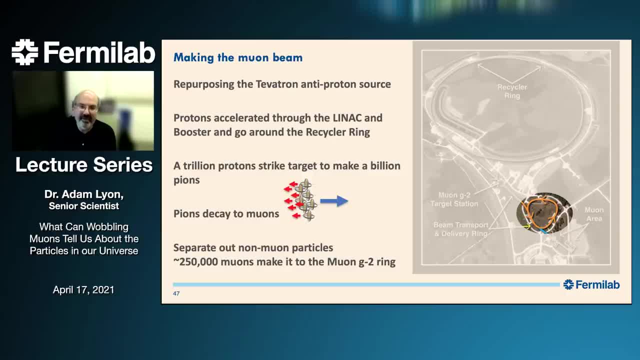 we use this delivery ring to separate out those particles from the muons and then we throw those particles away and let the muons continue on into our ring. so out of a trillion protons that strike the target, about 250 000 muons make it to this point down here right before they enter. 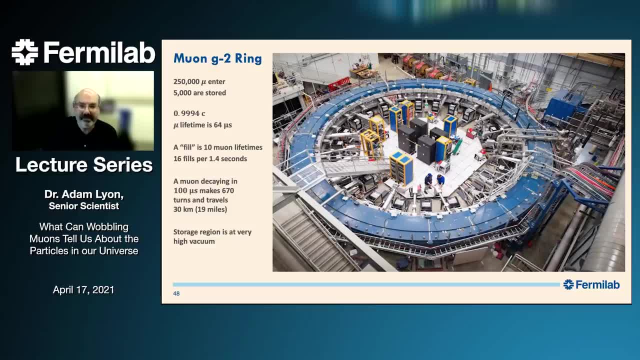 the building for the, for the g minus two ring. and so here here is the g minus two ring. uh, it's the same. brookhaven ring. uh, the magnet itself is the same, but everything else is new. uh, inside this magnet, although some things are recycled. uh, these beam line components here, these magnets, this is 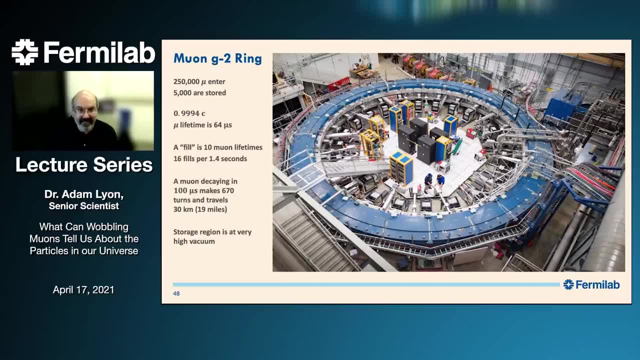 where the beam comes in. muons come in this way from from the building outside the building into here. they go into the g minus two ring. these, these uh magnets, are recycled from other parts of the lab. um, so about 250 000 muons enter the ring. they're sort of a torturous route they have to follow to get stored, to go to continue. 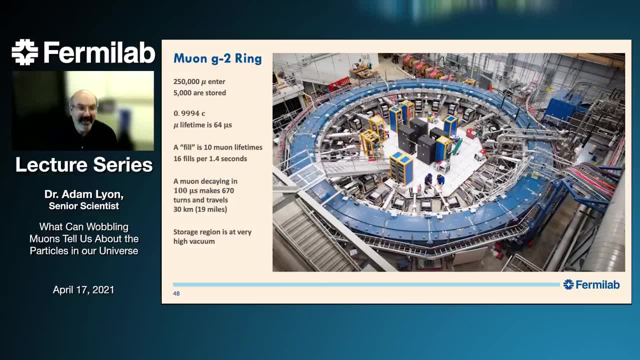 going around. only about two percent make it through that. so we actually only store about 5 000 muons at a time. these muons are going really, really fast. uh, you know 0.9994 the speed of uh times the speed of light, and so, if you remember special relativity, uh, when you have uh something, 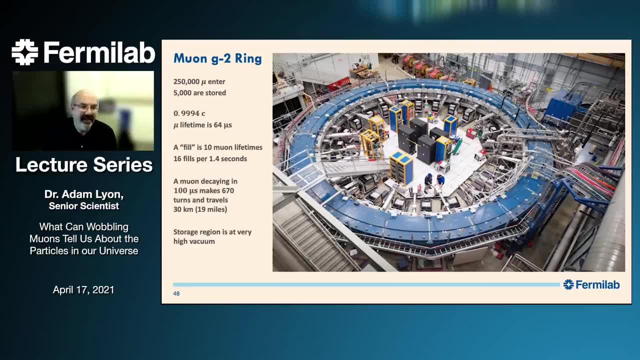 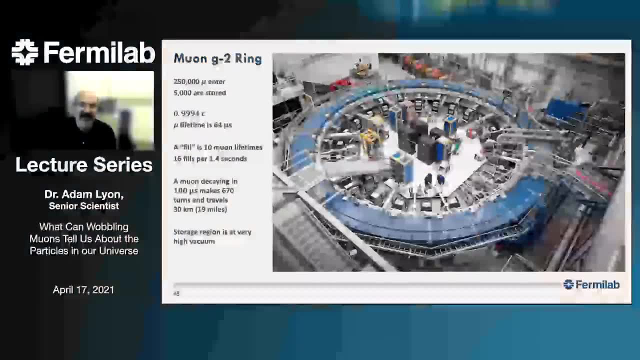 it's clocked to us looks like it's going slower. uh, and so a two point: a muon that would at rest live for 2.2 seconds on average, lives 64 microseconds. sorry, 2.2 microseconds. live 64 microseconds. uh, and this is great because the muons will live quite a long time. they'll go. 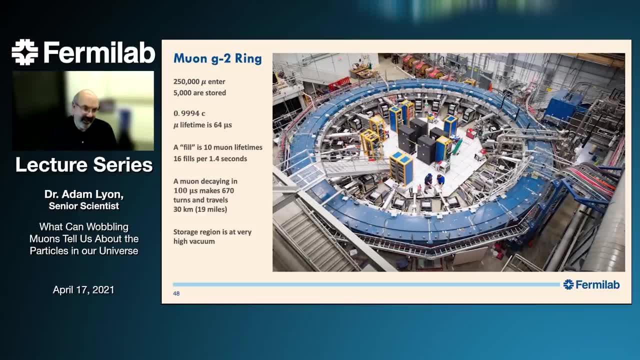 around lots of times. actually, this is on, this is the average. so some muons live shorter, some muons live a lot longer, and so we actually allow these muons, uh to, to go around for 10 muon lifetimes. so after about 700 microseconds they're all gone. they've all gone. they've all gone, they've. 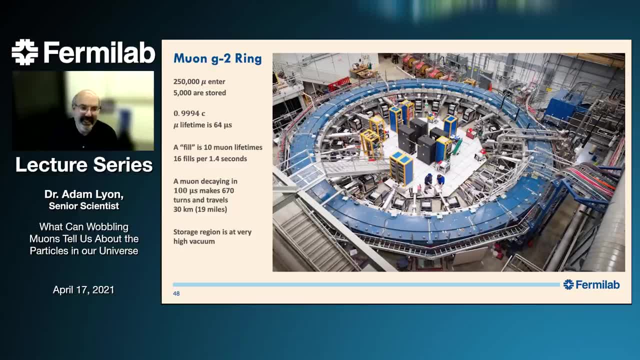 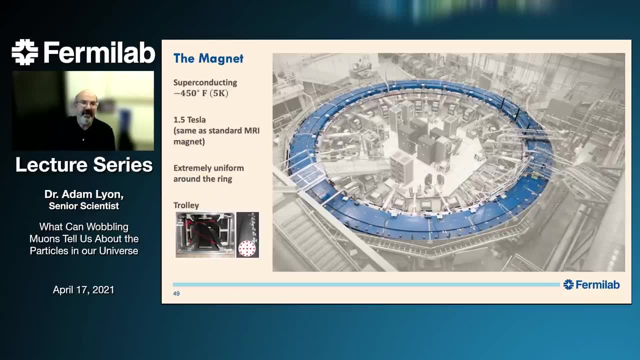 all decayed and we fill the ring uh 16 times every 1.4 seconds and the ring is at a very high vacuum, so the muons don't hit anything. the magnet itself is superconducting. as i mentioned, we have to put high current in this magnet uh to get the magnetic field we want, and so we have liquid helium going. 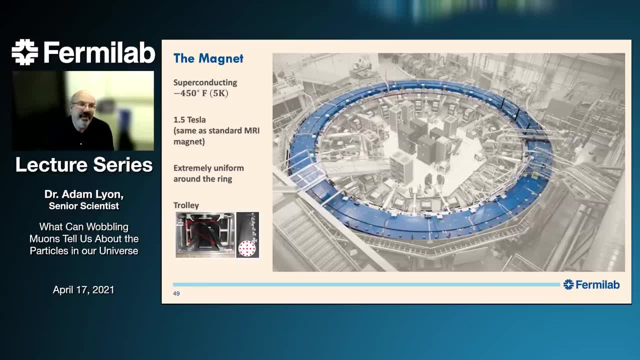 around those coils at five degrees kelvin or negative 450 degrees fahrenheit, uh. the magnet strength itself is about the same as a standard mri magnet uh in a medical office. so pretty strong but but strong, but, you know, quite strong uh, and we've done a lot of work. it took us a year of. 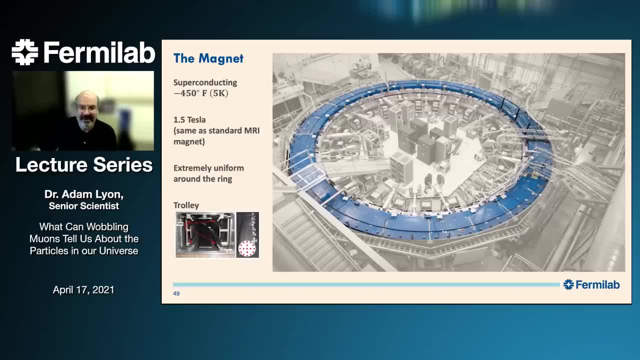 adding little bits and pieces, little bits of metal here and there and turning knobs to make this, the magnetic field itself, as uniform as we could all the way around the ring. that really helps us with the analysis. and then we had to measure the magnetic field. remember, we have there's the 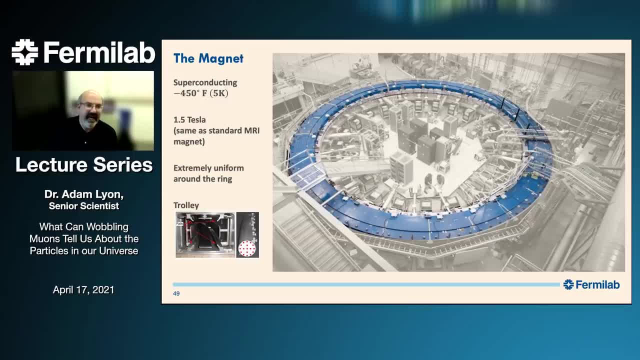 b part of our formula. we have to know what the magnetic field is, and so we have. we measure that we have, uh, embedded probes, hundreds of embedded probes, inside the ring itself, and then we actually measure the magnetic field with the trolley. it's a little railroad car that goes around the ring. 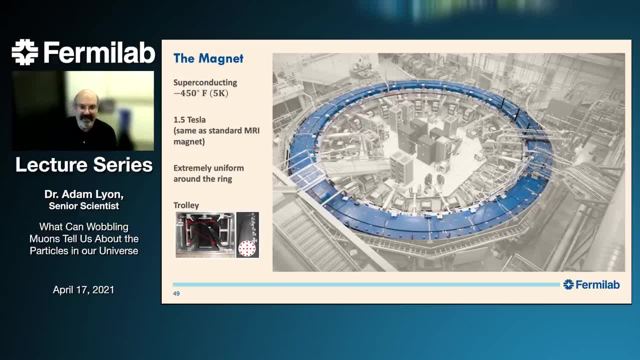 the little rails here and the trolley itself has 17 uh probes on it and it measures the magnetic field as it goes around in 9 000 stations as it goes around the ring. we can't run, we can't have muons at the ring while the trolley is going around. the trolley will block them all uh. but 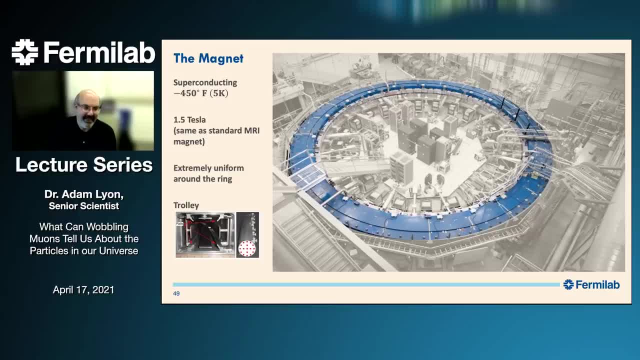 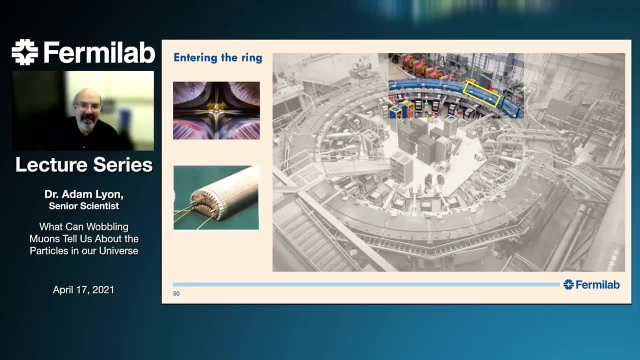 that's okay. so and we, we take a break every three days, uh, running muons, and we stop the muons and then we run the trolley and measure the magnetic field. well, that's really kind of neat. um, again back to the muons, and you want to enter from the back, they have to enter this magnet. so 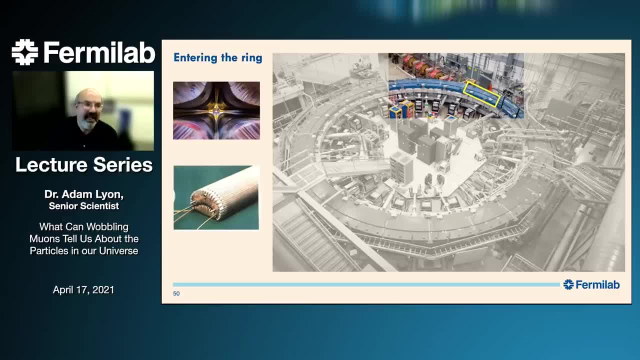 there's actually a hole in the coil where the muons can enter- uh, and this actually is a neat picture looking down these magnets here- but the muons go, go into the ring. there's actually a special magnet called the inflector that cancels out the magnetic field of the ring where the muons 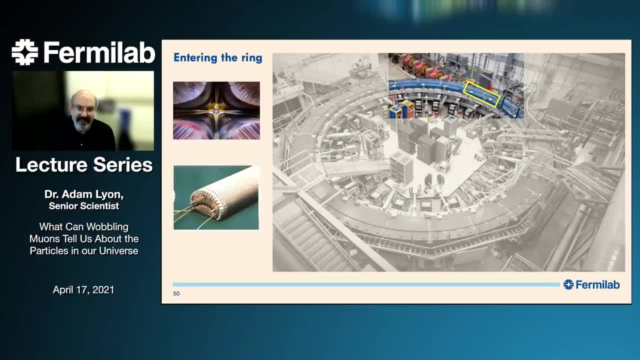 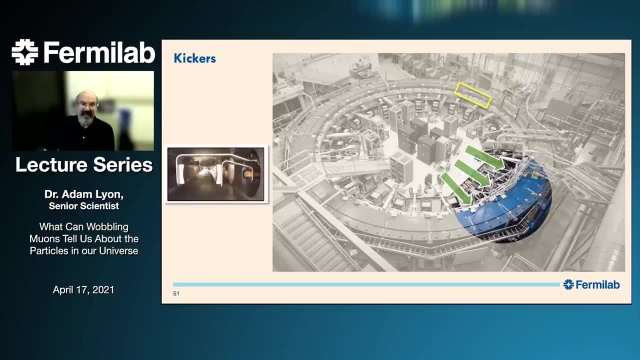 are entering, because the muons wouldn't like seeing a very big magnetic field all of a sudden. so we have to cancel the magnetic field with this strange looking magnet um, and when we do that, uh, there's a problem, and that the muons don't quite enter at the right orbit. so if we didn't do, 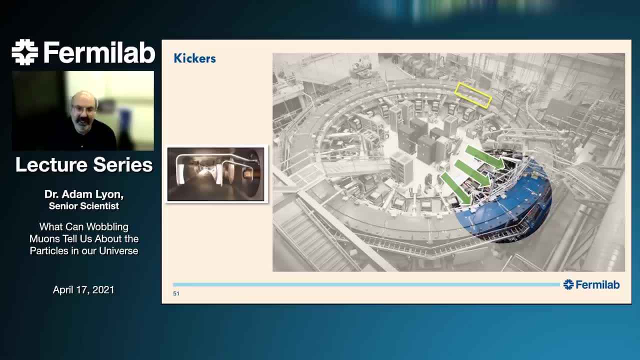 anything. if we just let them keep going, they would all kind of hit the wall here and we will lose them all. so we actually have to kick the muons onto the right orbit. and so, as the muons are going around their first time, their first time around the ring, when they hit about a quarter, 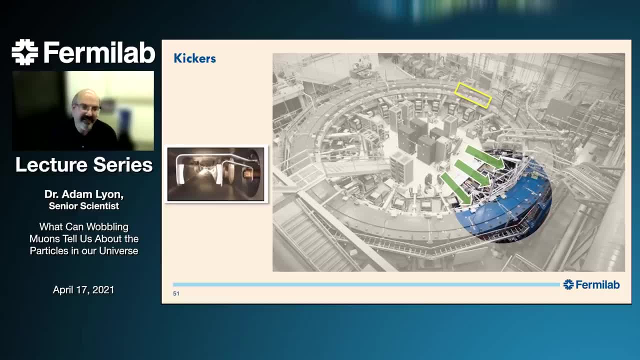 of the way around. there are these plates that we charge up to very, very high voltage and they fire within about 100 nanoseconds, so 100 billionths of a second, and as the muons are going, they are kicked about 10 miliradians. so not very much, but just enough, uh, so that they will will. 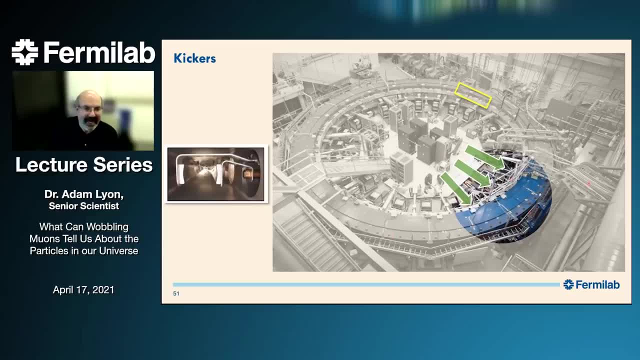 keep going around the ring, um, uh, and so we won't lose them. so, uh, so these kickers are very important, uh, and actually these kickers, you know they're, we need them, they're essential, but they also cause us a little bit of headaches, which, uh, maybe i'll get to and explain that, um. 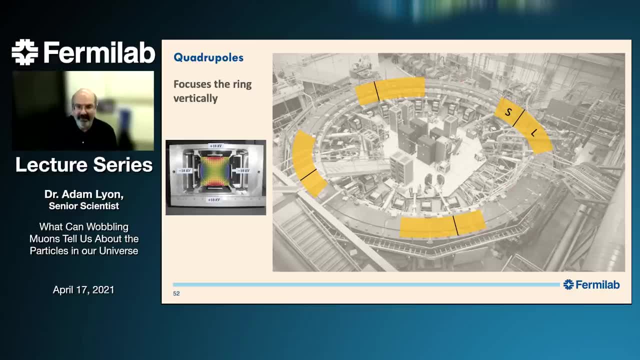 there's another complication, and that the magnetic field itself of the ring keeps the muons focused, but only in kind of the horizontal direction. so here's, here's kind of a cross section of what the, the beam, looks like, the, the vacuum region. so the muons are in this region. here they're going. 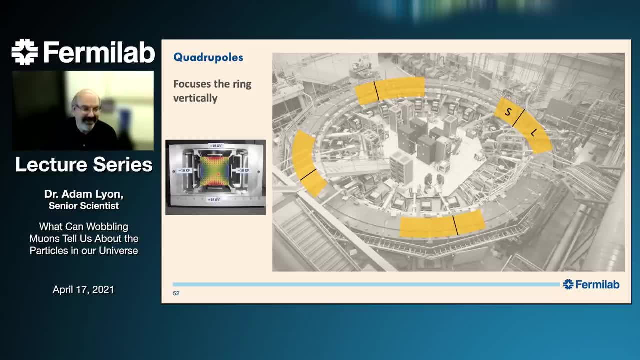 uh into uh the screen at some level. so imagine the muons going by into the screen, uh, and so they live in this, in this, in this circle here about. it's a nine centimeter diameter uh spot where the muons go, and so they are focused in a horizontal direction so they'll stay in the ring. but if we 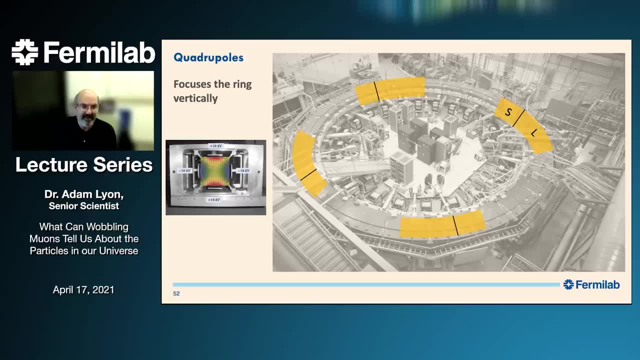 they would. they're unfocused in their vertical direction, so they would basically get more diffused, they get taller and off the beam would get more and more spread out vertically and eventually we would just lose them all after a couple of turns. uh, so we have electrostatic plates. 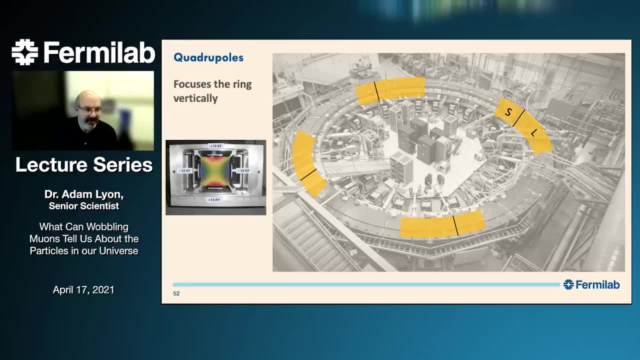 these quadruple plates that act as a lens. there's four room here, uh, one on each side, and we charge these up and these keep the the beam vertically focused. uh, so that's really important. if we didn't do that, we would lose the beam. so we need these things to keep the the muons in the ring. 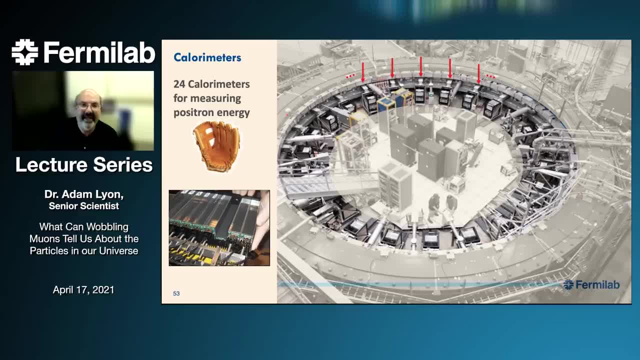 and then we have, uh, the detectors, the calorimeters, the catcher's mitts, right, so we have 24 of these things. i pointed out a few of them, um and uh, and so these, these are little boxes that are inset sort of into the ring, uh, where the positrons go. remember, the positrons curl inward. so we have 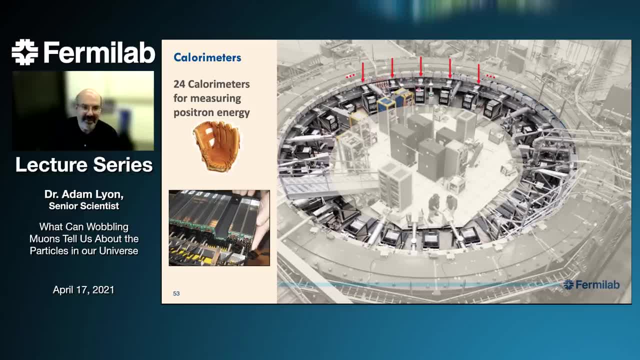 these boxes, that's to catch them, um, and they serve at the end of these carts to have all the services for for these calorimeters, and there's, like i said, 24 of them all the way around. and these are like a little bit of an example of what we call a crystal. uh, so when a positron enters a crystal, 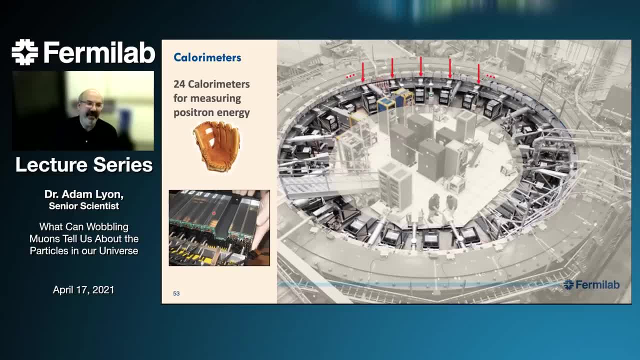 it kind of rattles around inside the crystal and makes lots of other particles and things and the crystal reacts by giving off a tiny, tiny bit of light. it gives us, gives off photons, and we can- we can- capture those photons and measure how many photons there are. uh. 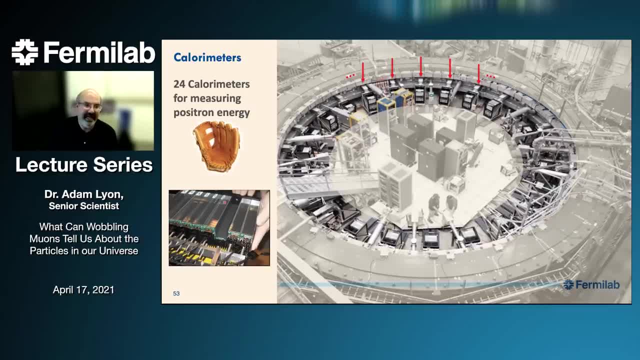 with a device at the end called a sipum, and basically the more light that gets produced, the more energy the positron has and the more signal we'll see on these systems. so that's how we do the energy measurement. That's how we measure that spectrum, the oscillating spectrum. That's what 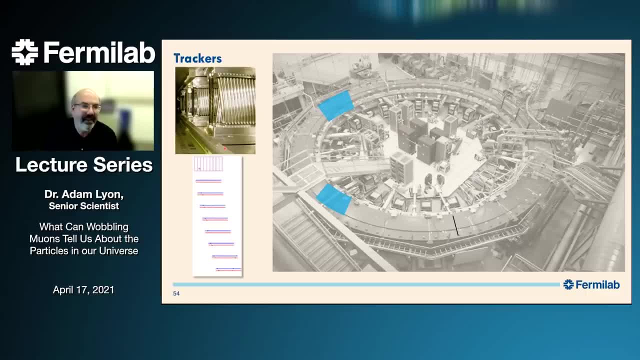 these colorimeters does what they do, these catcher's mitts, Okay. And then we also have devices called trackers, that, these weird straw looking things. So actually inside these straws, these are where the positrons go. So the positrons go through these straws. They're very thin. 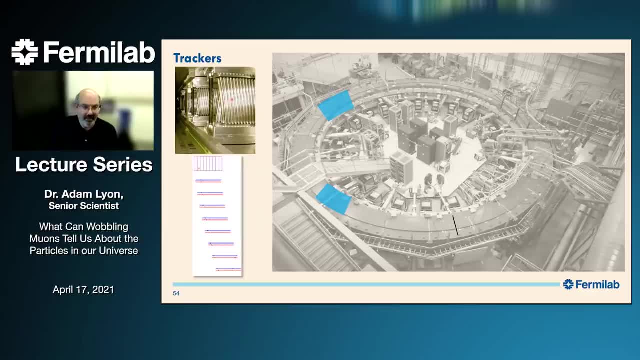 So they don't really block the positrons. Inside these straws there's a wire and there's a gas, And when the muon- I'm sorry, when the positron goes through the straw, it ionizes the gas and the wire senses that, And so it's a little hard to see here sort of where these trackers are. 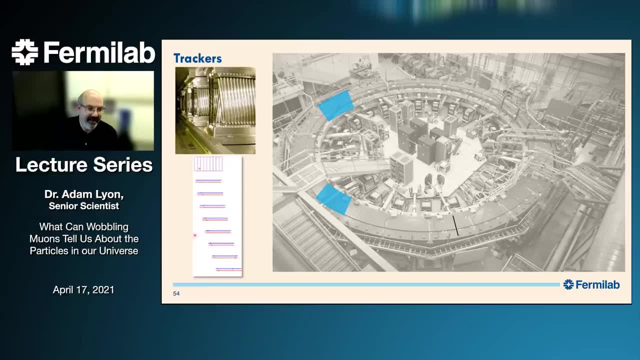 If you look carefully, there's little black dots where the positrons hit the wire, And so we can sort of connect the dots and extrapolate back somewhere around here and see where the muon was when it decayed. So we can get a picture of, we can deduce, where that muon was when it decayed. 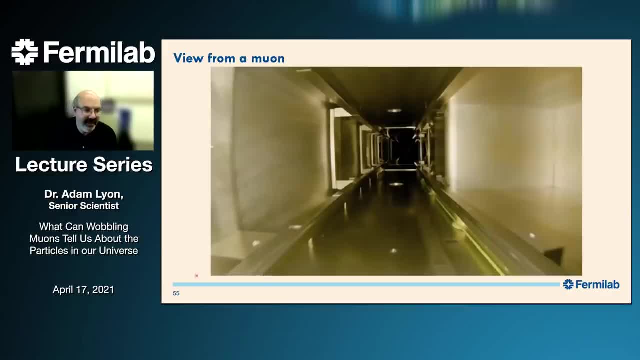 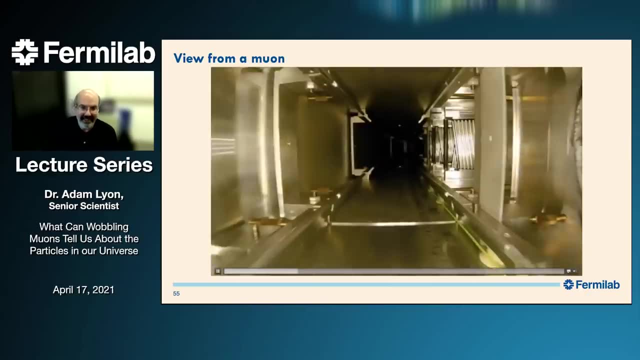 to the positron, And that's a really important thing we need to do Just very quickly. I'll show you a little movie. I got to turn off the laser pointer. If you were a muon, this is kind of what you would see. It's not stopping and starting. 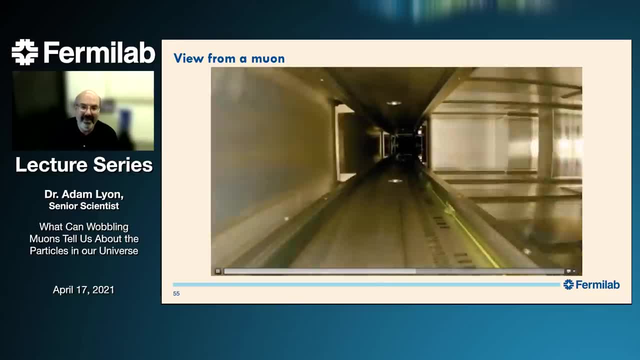 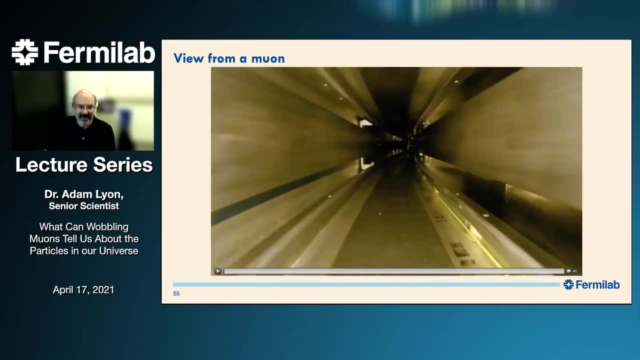 That's because it's on a trolley. Here's the trackers The trolley has to move along. There's the calorimeters behind here And here are the quadruple plates. So of course you're going around. It takes about 140 nanoseconds, 140 billionths of a second, for a muon. 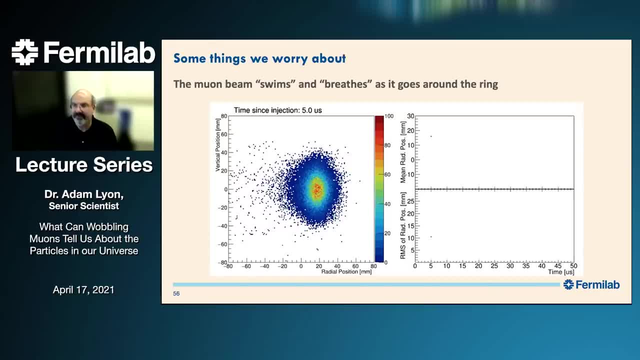 to go around the ring, So you'd be going around a lot faster. All right, I'm getting close to the end, So let me just go through this sort of briefly. So I mentioned the kicker causes some complications, And so the beam itself. if you imagine where the beam of 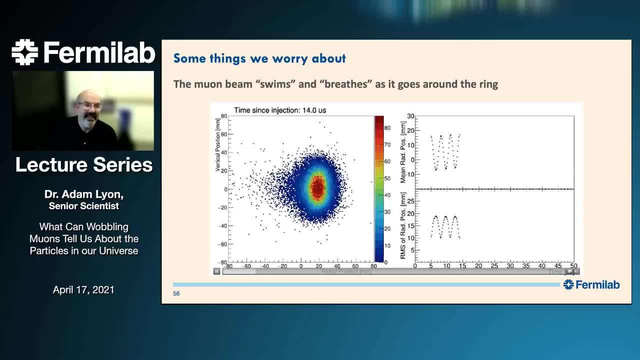 muons are in the ring. they kind of slosh around And so we say the muon beam swims back and forth. This is sort of what the muon beam looks like as it's going around the ring. So we kind of 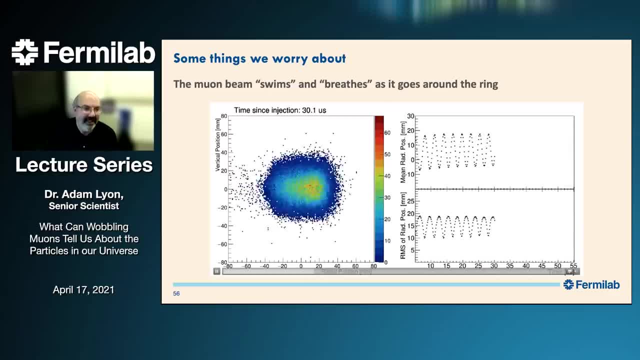 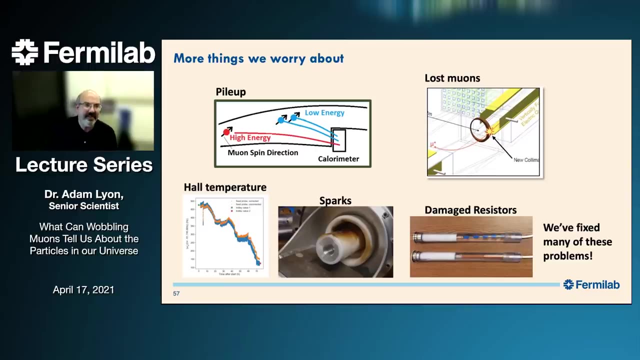 in this box, this nine centimeter diameter box or circle the ring, the muons kind of slosh around So it swims and the width of this gets bigger and smaller And so we say it swims and it breathes. So the muons are not always in the center, which causes some problems. But we have to figure that. 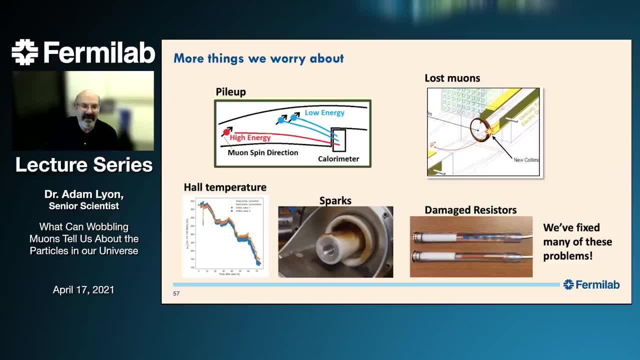 out and deal with that. We have other interesting things, like we have two low energy positrons from decays that enter the calorimeter at the same time, or a calorimeter at the same time. The calorimeter might not be able to travel apart if they're so close in time, So it'll actually add. 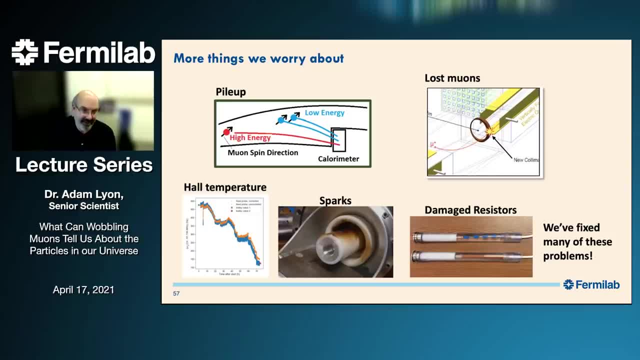 the two together and it'll look like a really high energy positron. And so we have two low energy positrons from a muon out here. So this is called pile up, And we have to actually figure this out and subtract that off, because that's actually a mistake. It's an unavoidable mistake, So we can. 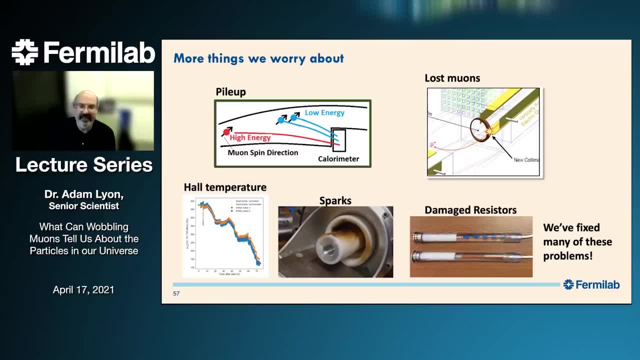 figure that out by different means: simulation and from data, And we can subtract that off. We can have muons on the edge of the beam that hits things and then curl inward and maybe hit a calorimeter. So muons doing that would confuse us a little bit. We can actually figure that out. 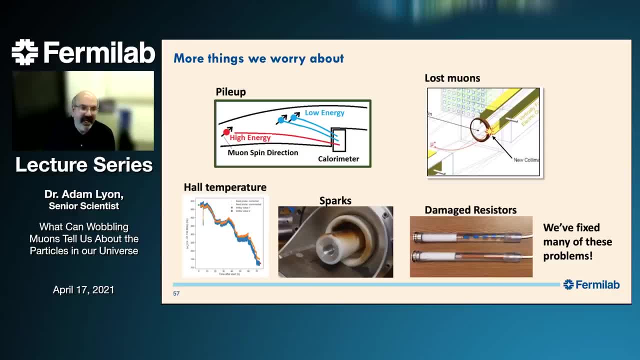 by looking at data We can figure out how often that happens. The temperature in the hall: this was our first run, So we were learning things. for the first time. The temperature in the hall was not well controlled And so that changed the magnetic field of the magnet a little bit, So we had to deal with that. These kicker. 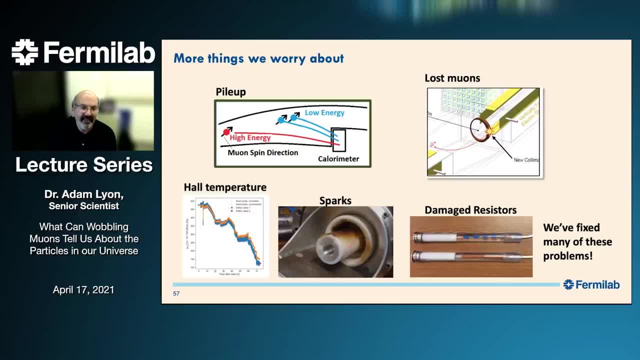 plates are very high voltage And so sometimes we would get sparks. So we had to actually run the lower voltage than we wanted. And we also- the quadruples- have high voltage resistors And the company that made them for us couldn't quite make enough of them, So we had to actually run them. 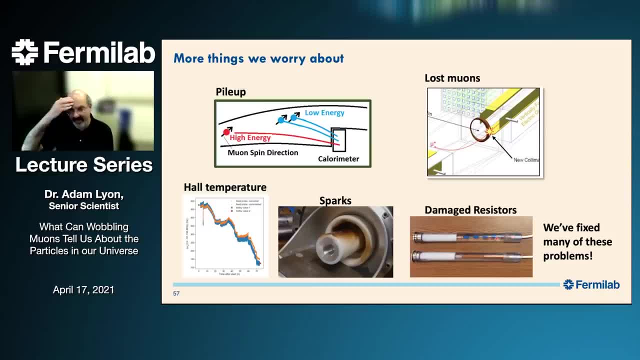 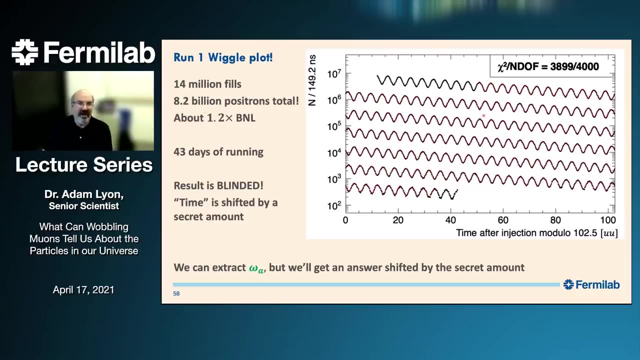 ourselves, And we didn't make very many. I think we made like four or five of them, But two of them didn't work so well And so that created some problems. But anyway, we have to figure all that out. That's part of what we do, And so here is our wiggle plot. So remember, I showed you the wiggle. 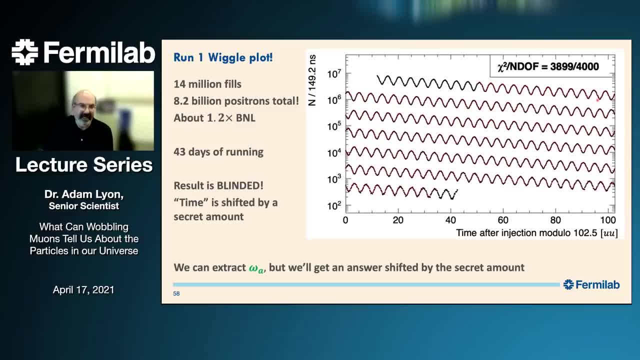 building up the wiggle plot, And so this is what ours looks like from our experiment. It looks sort of like what you saw there building it up, And so in this and one thing to note- this wiggle plot wraps around. So if I showed you the one long, thin wiggle plot, that'd be really hard to see. 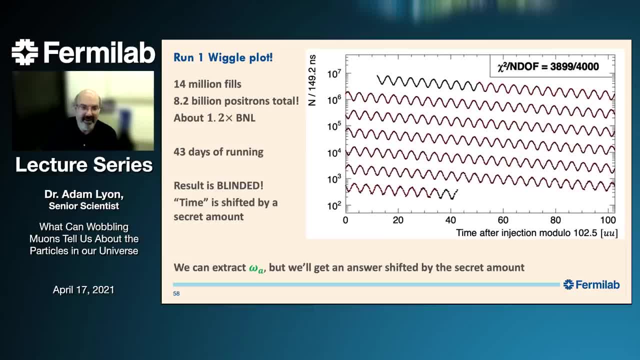 So this point here wraps around to this point here. So overall it's about 700 microseconds. It's actually, you can see, it's kind of sloped downward, And that's because we're actually measuring the number of positrons, And as muons decay over time, there's fewer and fewer. 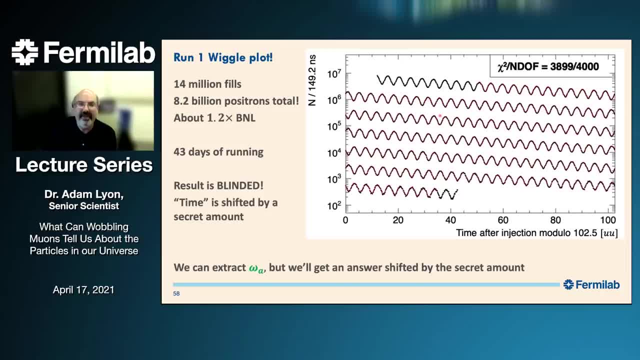 positrons, There's fewer and fewer muons for them to come from, And so this. so you're seeing the number of muons decrease over time, And this is the number of muons that we're measuring. And this is the number of muons that we're measuring over time, And this is the number of muons that we're. 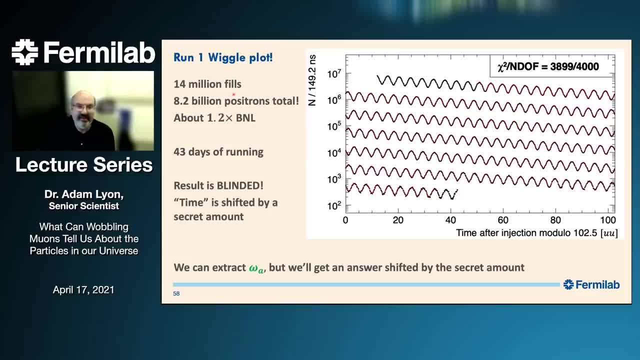 measuring, And this is the result of 18 million fills, 18 million fresh batches of muons and 8.2 billion positrons total, which is a little more than what Brookhaven saw, And this was a little more than a month of running. So what took Brookhaven about three years to do in terms of 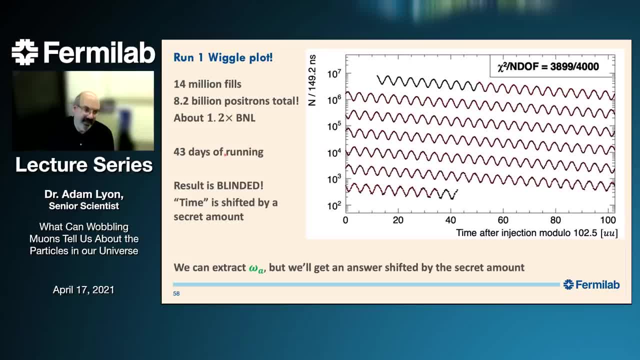 data. we can produce about the same amount of data in a little more than a month. right, And so this is, you know, shows the power of the Fermilab complex, that we can make a lot more muons. One thing to note is that I have weird units here. I. 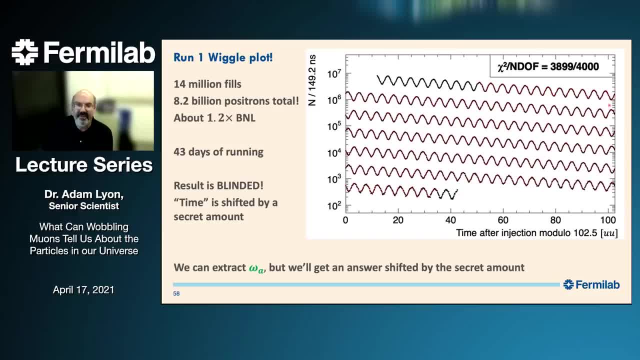 said this was 700 microseconds, So this point here should be about 102 and a half microseconds, but it's not. It's about that, but we don't actually know what this point is, And that's because we have blinded this experiment. We've actually shifted the time here by a secret amount. 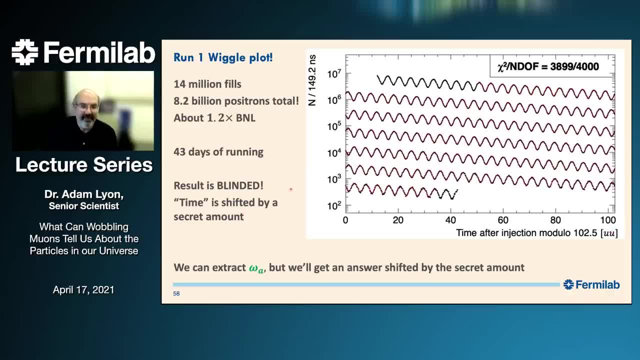 We don't know. on the experiment, we didn't know what this was, So we could extract the mega A. we could figure out what this frequency is, which would be a mega A, which would lead to the anomalous part of the G factor which is 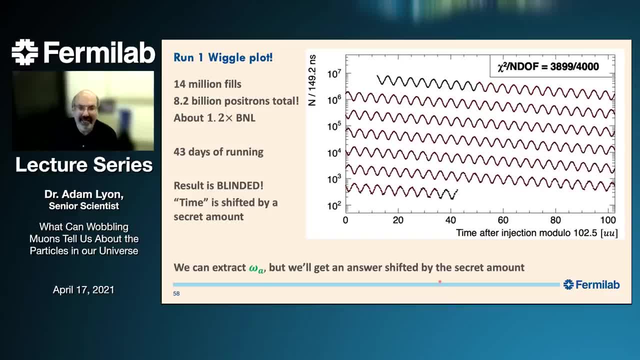 what we want, But we would actually get an answer shifted by a secret amount. So we couldn't actually figure out the answer. We could do everything else, but we couldn't actually know the answer. And that was something really important for us to do, because, you know, there's sort of an answer. 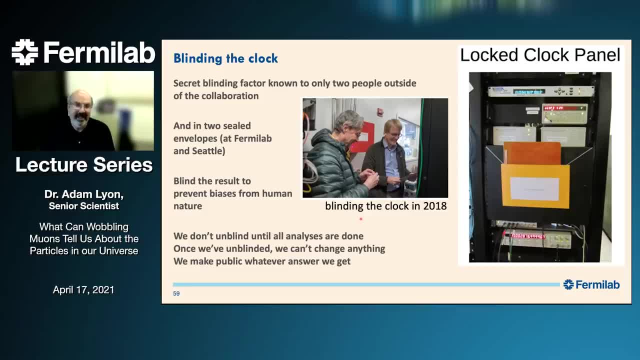 that everyone's hoping for right. You know we're all hoping that. maybe you know we'll confirm the Brookhaven experiment. And when you have something you're hoping for, you know and you sort of know how things are going, you can unconsciously 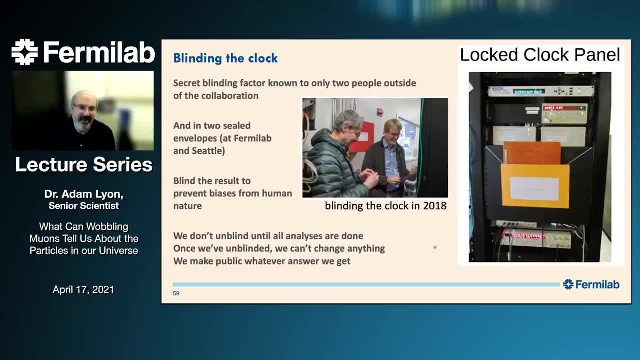 make decisions that kind of reinforce the result you want Right And we don't want to do that Right. We're we're scientists, You know we have to keep our cool, We, we don't want to be tempted into into sort of driving the result into something that we want. 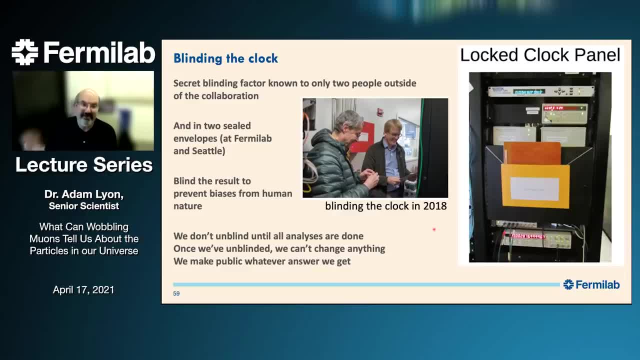 And so we actually make it. so we can't figure out the result until the very end. So we have no idea. are we matching this to our model or are we confirming Brookhaven? We have no idea until we're done. And so there's a secret, blinding factor: We actually detune one of the 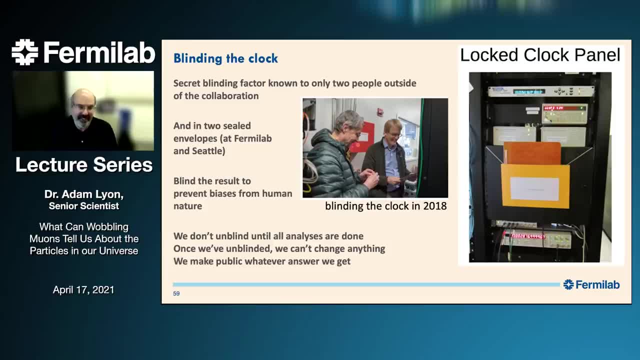 the clocks that feeds into the experiment which changes what omega-A we would get. That secret value is kept in two sealed envelopes, one at Fermilab and one at Seattle, where we have a lot of people who work on the experiment, and it's in two places for safekeeping. 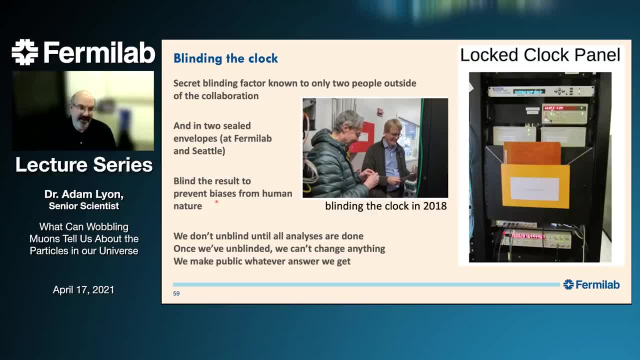 And, as I mentioned, we blind the results to prevent biases from human nature. And so we don't unblind until all the analyses are done, And we have a rule that once we do unblind, we're not allowed to change anything. What we get is what we get. 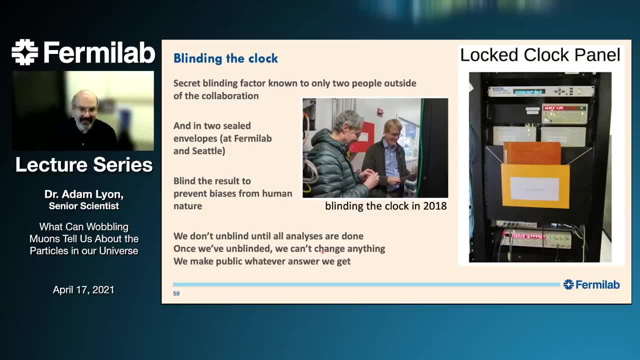 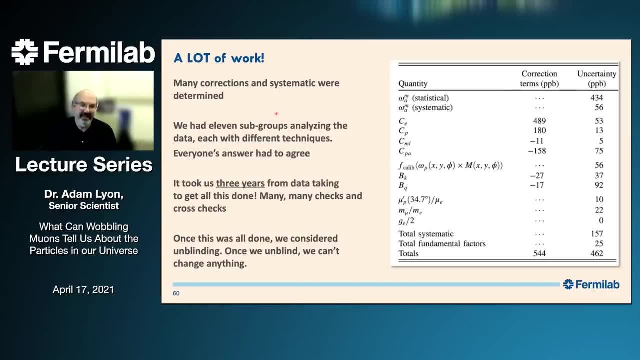 And so we make public whatever answer we get, And that is a rule that we have to follow. It's actually in our bylaws for our collaboration, And so I won't spend too much time on this. Don't worry about the numbers. 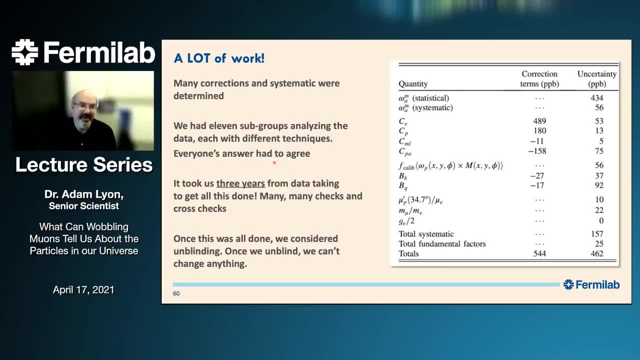 This just shows a lot of the uncertainties and corrections we figured out. This was an enormous amount of work. It took us three years after collecting the data to do all the analyses. We had 11 groups doing the analyses, each with a different technique. 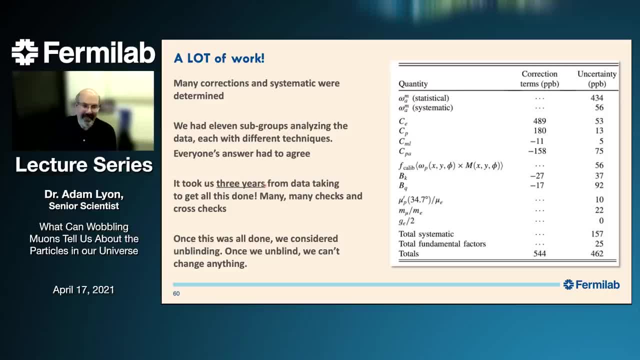 They all had to agree in the end And we had many, many checks and we solved many problems and estimated uncertainties for many problems. We had checks and cross-checks. So it took us three years to do all this And once all this was done and we all checked each other's work and saw presentations about how all this was done, 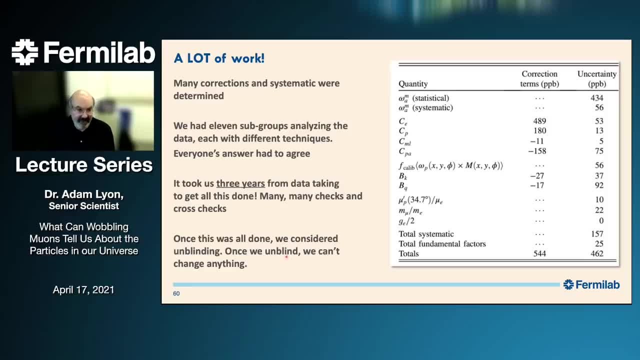 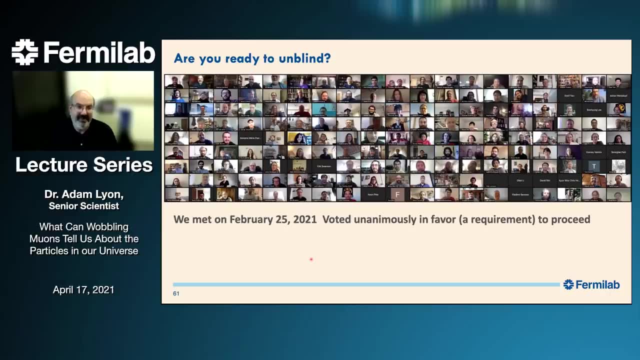 then we could consider unblinding. Remember, once we unblind, we're not allowed to change anything. So whatever it is, we is, But whatever it is it is. So whatever mistakes we made, we better figure those out before we unblind. 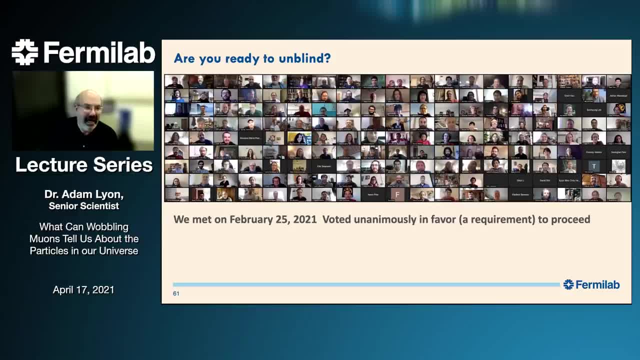 So about February 25th- a little more than a month ago- we all got together, So we had about 170 people. that was the authors of the Rubble One paper, which is a fraction of our data. We all got together and we all had to vote. 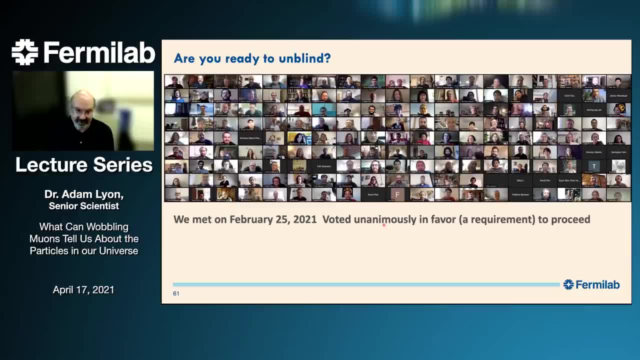 And the vote had to be unanimous in favor of unblinding to proceed- And if we didn't vote unanimously then we wouldn't unblind. We'd have to look harder and maybe understand what was the concern from that particular person. That wasn't the case. 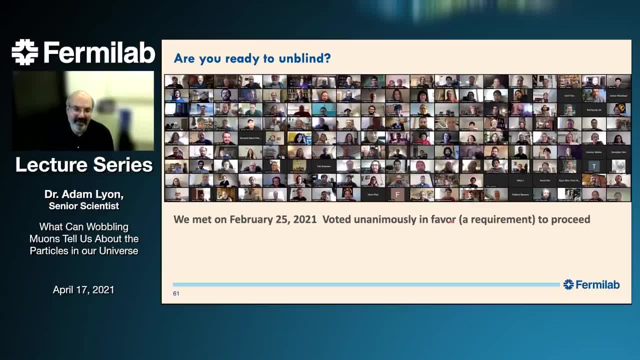 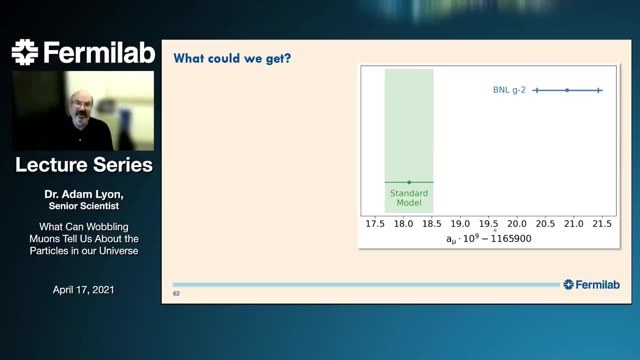 We were satisfied that we'd done everything we could, and so we voted unanimously to unblind. So before I show you the answer, you probably already know the answer, but let's look to see what we could have gotten So very quickly. so here's sort of the answer plot. 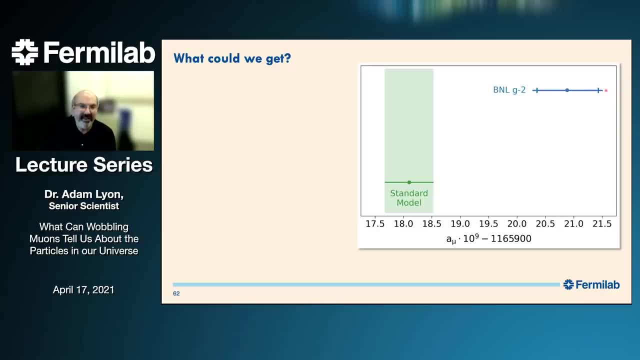 Here's what Brickhaven got with their uncertainty bars, and here's where the standard model is right. And here's this gap, this 3.7 sigma gap. So what could Fermilab get? Well, we could get a result that confirms Brickhaven. you know, if our result overlaps. 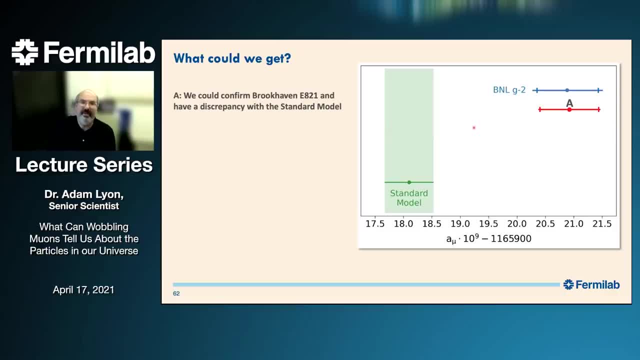 the Brickhaven result, then essentially we're confirming Brickhaven and we also would have a discrepancy with the standard model And, as we said, as I said, you know, this is sort of what we're kind of all hoping for, right. 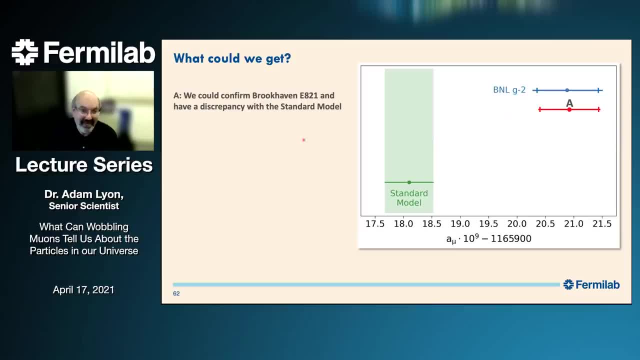 That would be the best thing, although you know we've got to keep our cool. you know that might not be what we get and of course we blinded, so we're not influenced by this. You know we don't make decisions based on that. 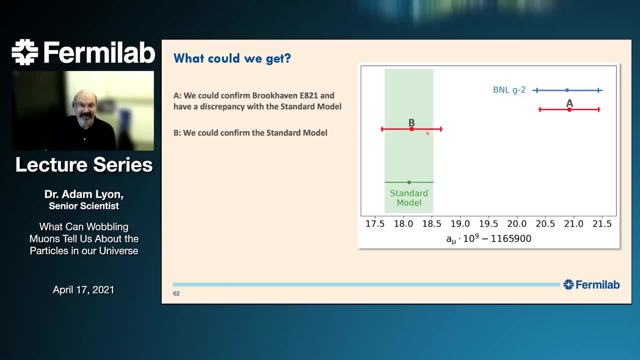 We could confirm the standard model right? That would be interesting. That would. so that would beg the question as to why the Brickhaven result, you know, would be interesting. The result is so different. Maybe they just got unlucky and saw what we call a statistical fluctuation. 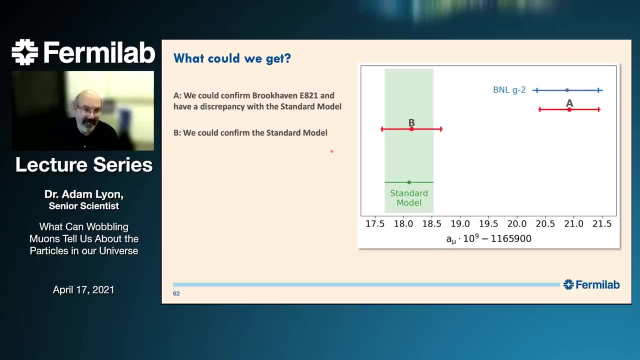 but that would have to be investigated. So this would have to be explained: why we got, why we got the standard model value and they didn't. that's a possibility. We could get something in between. So you know, that's. that's sort of the most unsatisfying answer. 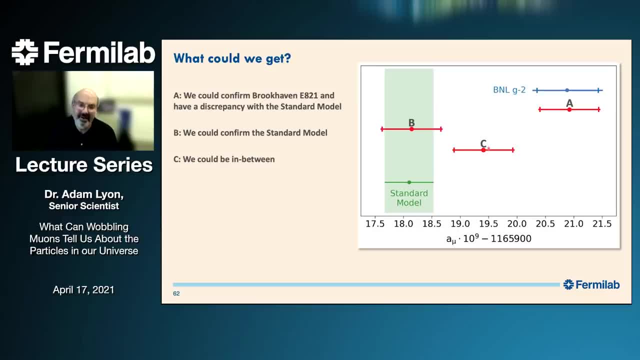 because we can't really say what's going on here. if we get something in between, We would have to analyze more data, which is what we're doing, and hope that this, this, will either move around, maybe we're seeing a fluctuation. 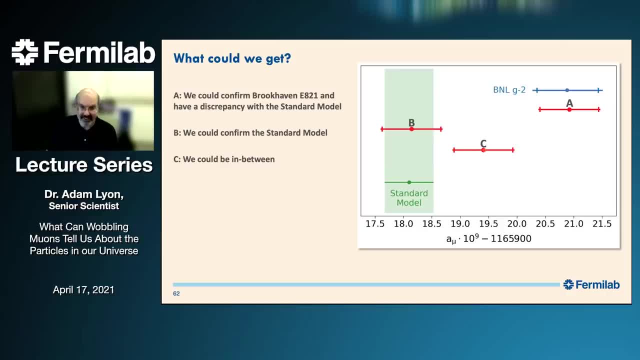 you know, we're going to get something in between, Or maybe this is the right answer, And then then our error bars would get smaller in the same position. So we would have to look at more data before we could really say anything. 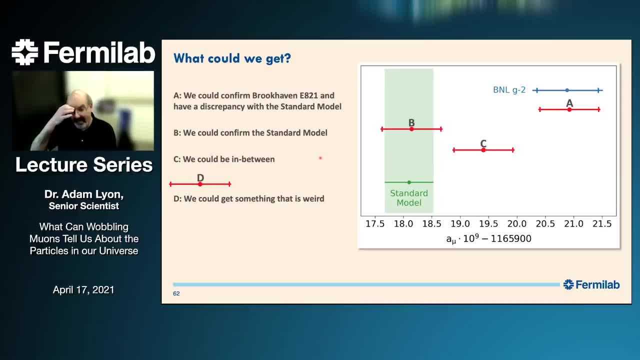 And then there's sort of the nightmare scenario where you know, we put in our calculations, we get the, we get the point on the plot and it doesn't show up on the plot, It goes somewhere else. right, Something weird's going on. 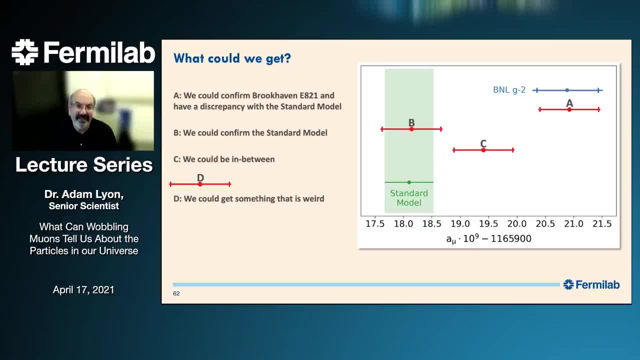 You know, we were pretty sure this wasn't going to happen. We had done so many checks and so many crosschecks and we were confident. you know, we would not have unblinded, We wouldn't have decided to unblinded, to unblind, if we thought there was something. 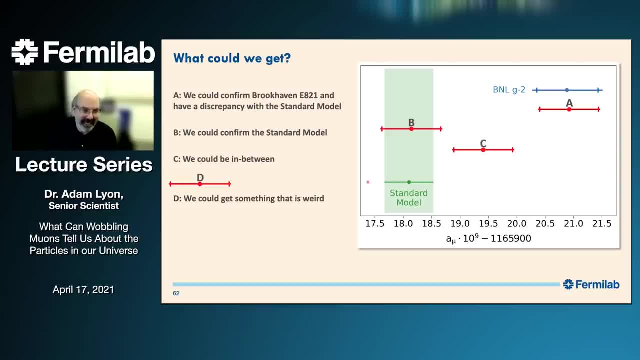 that we missed. So we really were confident that we wouldn't get, you know, some weird answer. But you know you don't know until you look right And and once we've unblinded whatever it is, you know that we have to make public right. 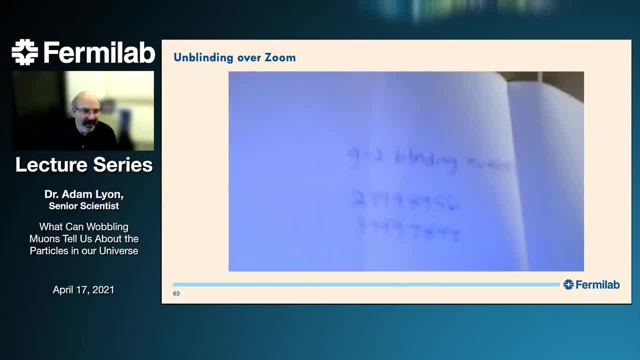 So I'll just go through this quickly Put it in the chat. We're getting a little late here, So we opened up the envelopes here. Steve Herzog from the University of Washington opening up his envelope with the, the, the secret factor. 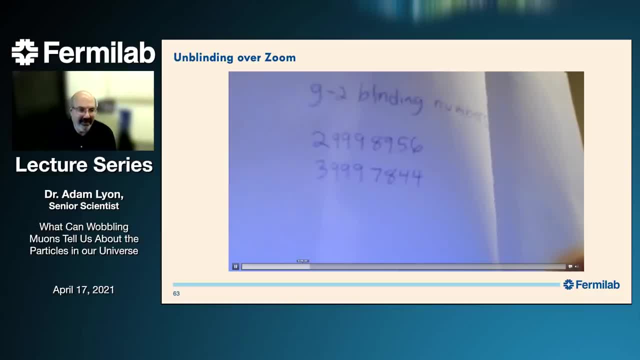 It's the bottom number directly. Two clocks up. We blinded for various reasons, So it's the bottom number that matters. Here's Chris Pauly, our spokesperson at Fremulab. He opens his envelope, gets the same answer, the same number. 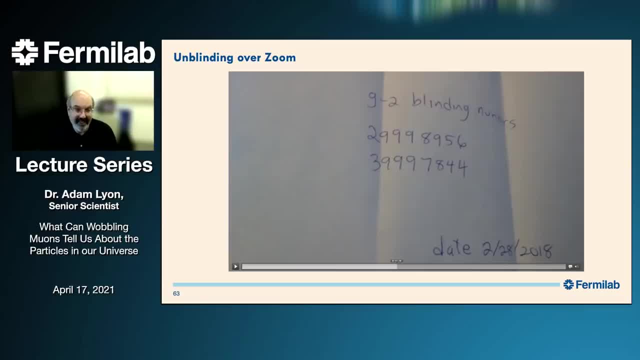 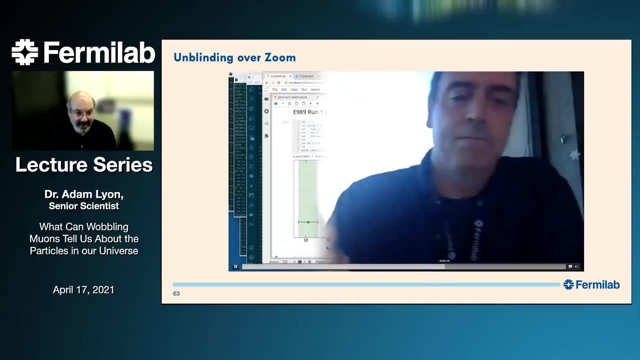 So that's good. So we have the same unblinding, secret unblinding number that we put into our, our notebook And we get the answer. So here I'll let this play so you can hear what our reaction was. This is pretty cool. 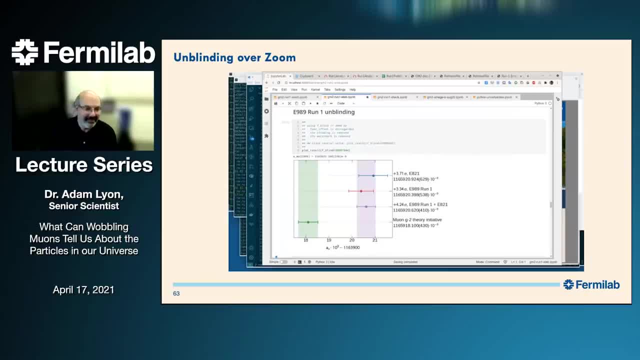 And this is what we get: Whoa, Wow, Wow. So we confirm the Brookhaven result. Here's our result here. So you have to realize, for us this is like landing on Mars, right? I mean, this is the Lars man, the Mars lander, successfully reaching the surface of Mars. 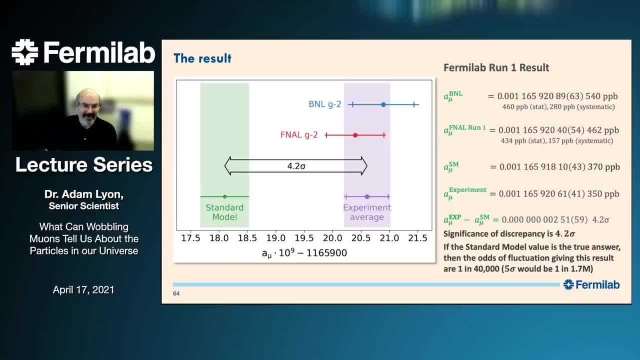 This is our Mars lander moment. Uh, and so we did in fact get a result very close to the Brookhaven result. Uh, here's the numbers. I won't go through the numbers, of course. uh, lots of numbers, but basically, on the graph, here is our Fremulab result. 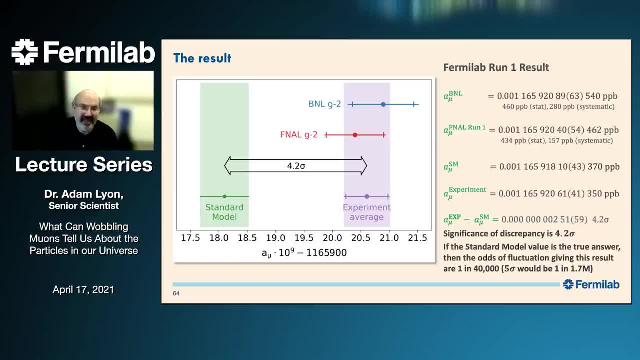 And, yes, we're a little bit to the left of Brookhaven, But we substantially overlapped, uh, and so we confirm their, uh, their results. And, again, this is why we unblinded right, Because, uh, because, if we didn't, if we did this, if we did this, you know, with, with, while knowing the answer, we would have to prove to people that we weren't influenced to get this. 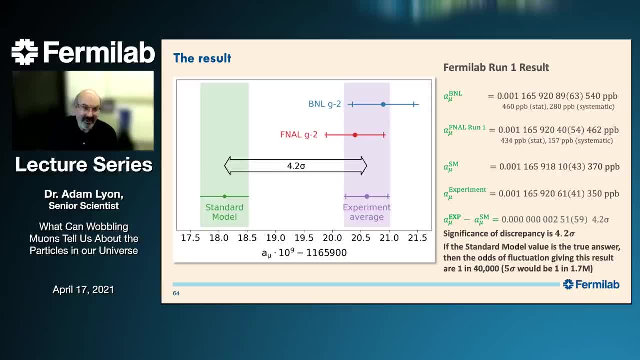 And? but because we blinded, we couldn't figure out what this was until the very end. Uh, and we have in our rules that once we unblind- this is you know- we have to publish whatever we get, and this is what we got. 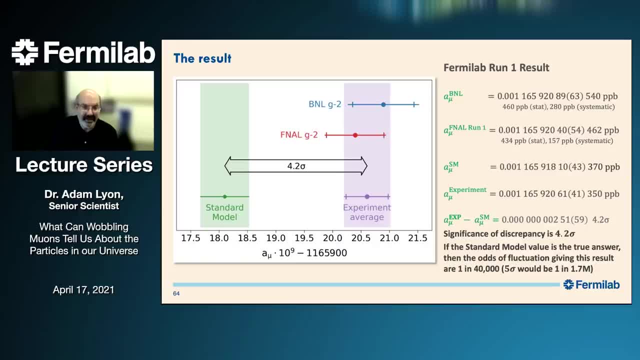 So, uh, we can actually aggregate, Uh, we can average these two together, uh, to combine our, the power of our two data sets, and actually we can get a, uh, a value, with a smaller uncertainty, by combining these two, uh, uh, independent experiments. 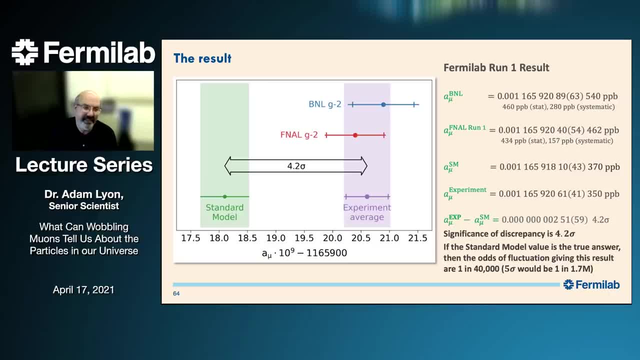 Uh, and because of the error bars get a little smaller. that increases the significance of the discrepancy with a fairer model. So instead of 3.7, seven Sigma, we're now at 4.2 Sigma. Uh, so we, we strengthen the discrepancy with this terror model. still not five Sigma. 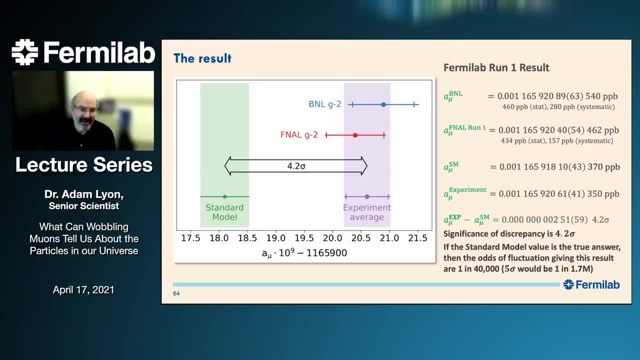 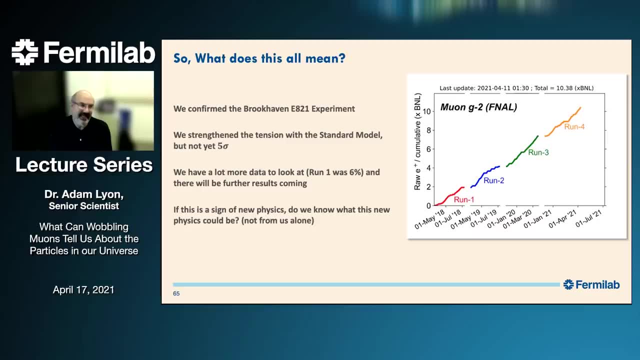 So we still can't claim a discovery. Maybe we're on the way, on the way to that. So that's so, that's very exciting. That's, this is why this is so exciting. Uh, so, in the end, uh, my second, the last slide, so we confirm, uh, the Brookhaven result. 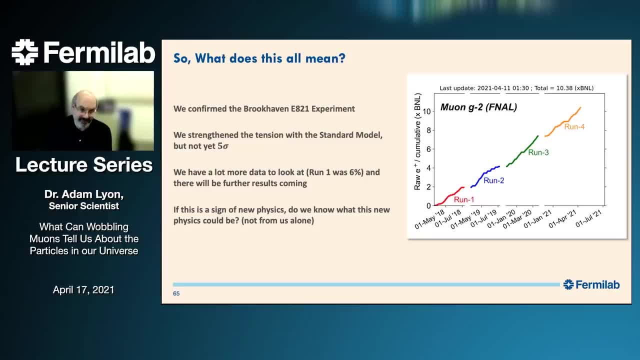 Uh and so so what Brookhaven did well was was confirmed by us, So so that means that's correct. We strengthened the tension with the standard model. It's a 4.2, two Sigma, not five Sigma yet. 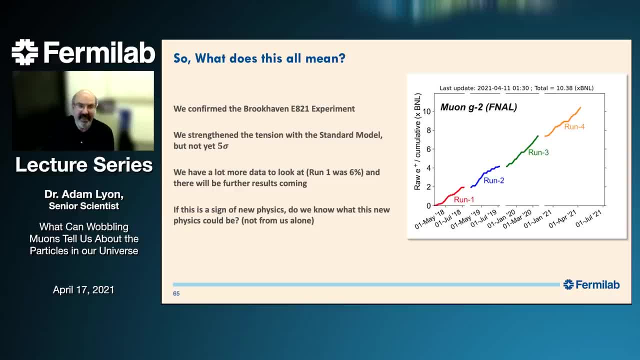 Uh, but maybe we're getting there, still can claim a discovery, but we have a lot more data To look at. uh, the run one. our first result was on 6% of of the total amount of data that we hope to collect. 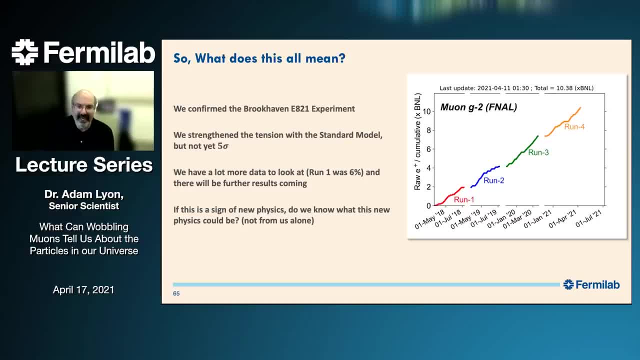 Uh, so we have actually two more years worth of data in the can: run two and run three. Uh, now we're actually in the process of taking run four and we'll have a run five and maybe we'll have a run six. Uh, so we're actually at 10 times Brookhaven now. uh, and, and we hope to get eventually. 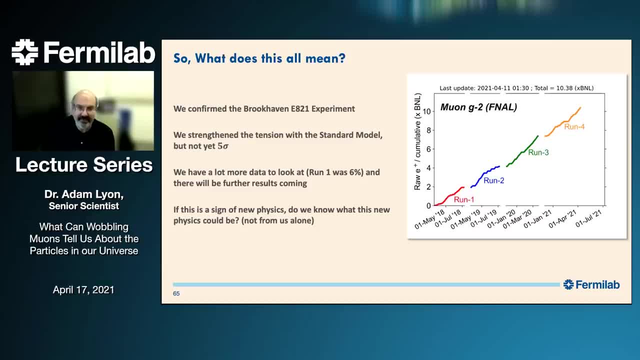 to 20 times per camera. right, That would be our, our full, full statistics. So in about a year, Okay, So in about a year, a little more than a year from now, we plan on uh releasing the results. 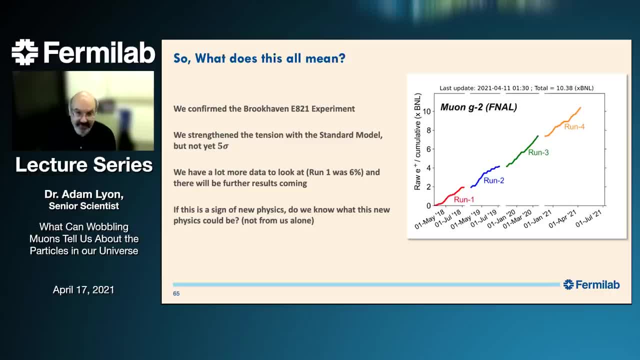 from run two and run three. So these are blinded still. we have different blinding, secret blinding factors, Uh, so these are still blinded. So we'll look at run two and run three. do those uh analysis and checks and cross checks. 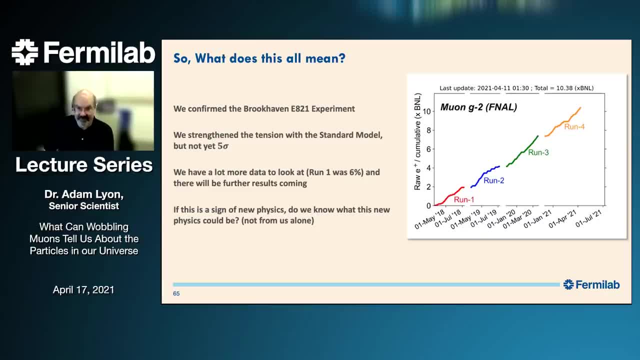 And then, you know, maybe in summer or 2022, we'll decide to unblind again and we'll see what we get. Uh, and then, as I mentioned, we'll take your run, for now, actually next week, I have to. 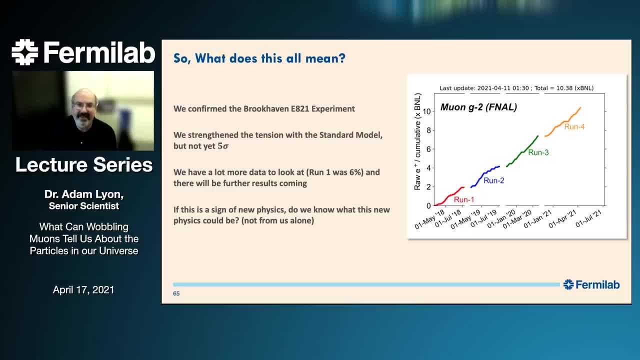 go on shift. We babysit, We all take turns babysitting the experiment, uh, 24 hours a day. So I'm on evening shift, uh, from four to midnight for four days next week. So I'm looking. it's actually a lot of fun. 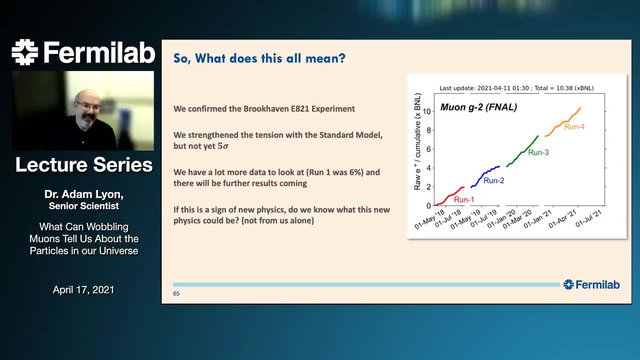 I'm looking forward to doing that. Um, and so we have a lot more data. So so what? what does this all mean? So you've heard there's been a lot of reports in the news. you know we've broken physics. 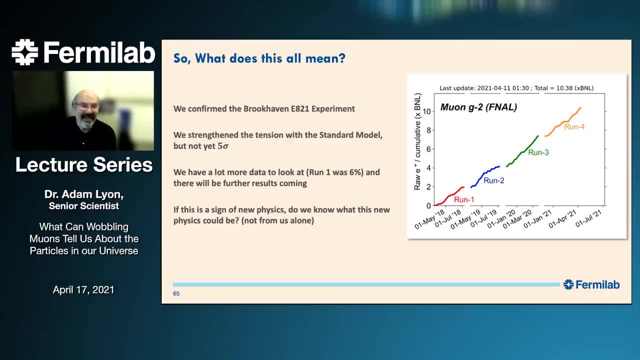 you know, you don't have to listen to your physics professors anymore. Uh, you know. so what does this mean, If this is this really were a sign of new physics- and again, not a discovery, but but? but we get, we have hints. uh, you know, what could this new physics be? 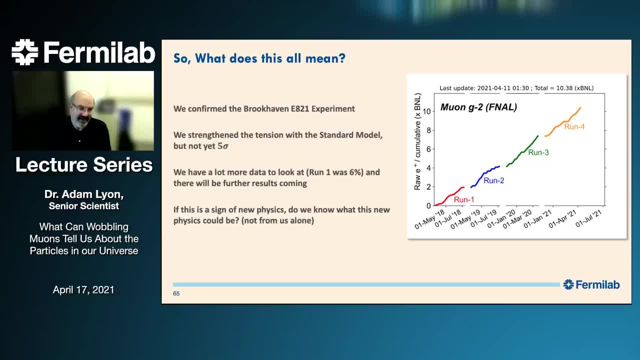 Uh, and the issue here is that this experiment by ourselves, we can't determine that alone. Uh, we have, there are, there are models, uh, that are compatible with our value for G minus two and are also compatible with not seeing anything at the LHC. yet 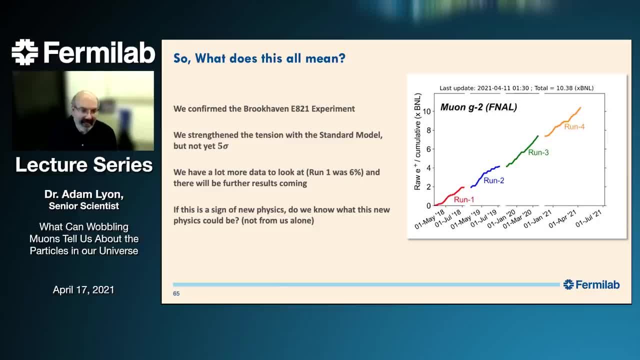 Uh, and we can't tell which of those models are right. Um, the LHC is doing a big upgrade and they will be. we'll be able to look at a lot more data, a lot faster than they could before. Uh, and so you know, there's hope that you know they can see rarer and rarer stuff because 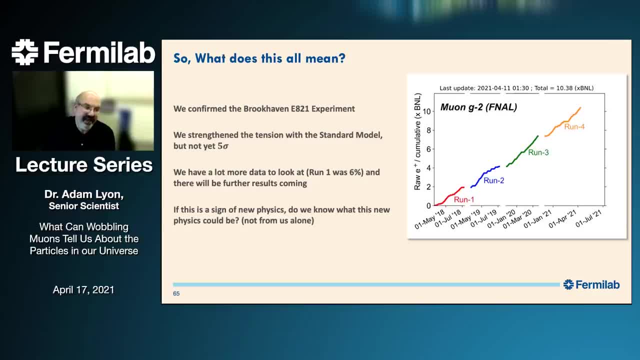 they're going to be making a lot more data, a lot more collisions, Uh, so maybe they'll have a hint of something as well, Uh. and so, to really pin this down, uh, we need another experiment to have to have a. 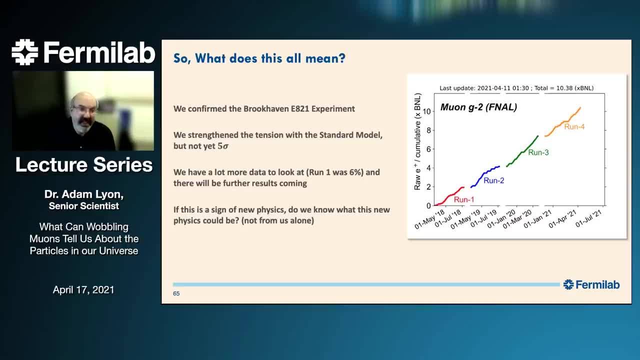 hint. There are some other hints out there, nothing above five Sigma Um, and so you know it's still a wait and see, uh, but you know it's still very exciting to see these hints, and especially the hint from us. 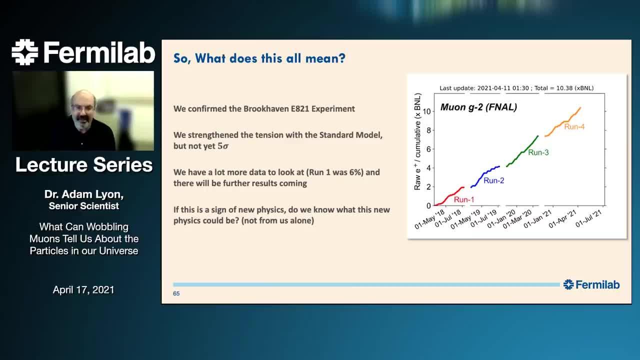 Yeah, Uh, come out, So, um, so, don't throw away your physics books. Uh, the standard model still works. you know where it works. it works well, Uh, and we'll have to see where, where these hints will go. 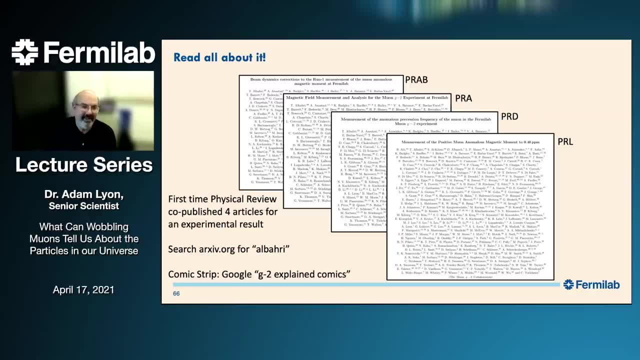 And and and it's very exciting. Um, if you want some, some reading material, if you can't sleep one night, uh, you can find our papers. Uh, there's a website called the archive. If you search for this person's name, you'll find our four papers. is, they're very technical. 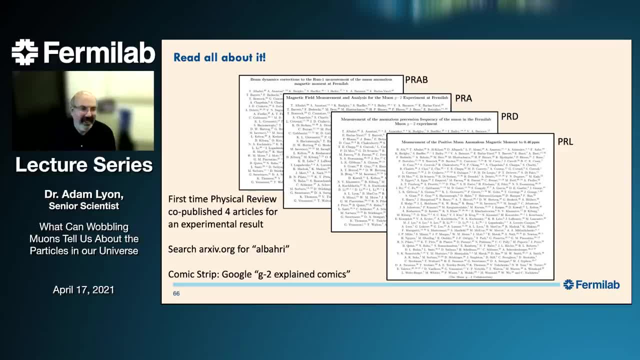 but they're, but they're neat. Uh, that describe the experiment. And if you actually actually want something more basic, um, actually we'll, we'll, we'll, sort of along the lines of what I've talked about. If you Google G minus two, explain comics. uh, the American physical society uh has. 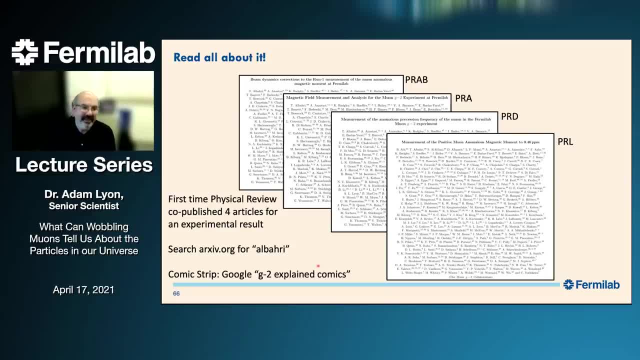 a comic that they've, um, they've asked, uh, uh, this person who makes the PhD comics. he's really good, Uh, and he has a comic strip about, uh, the G minus two. result: Okay, That is all that I have. 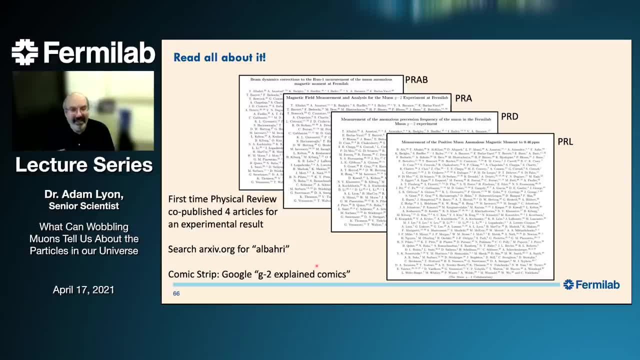 So, uh, hopefully I left you with a sense of how the experiment worked, uh kind of the history of it, where we where we've gone, What we've done and where we're going and uh some some idea of why this is so exciting. 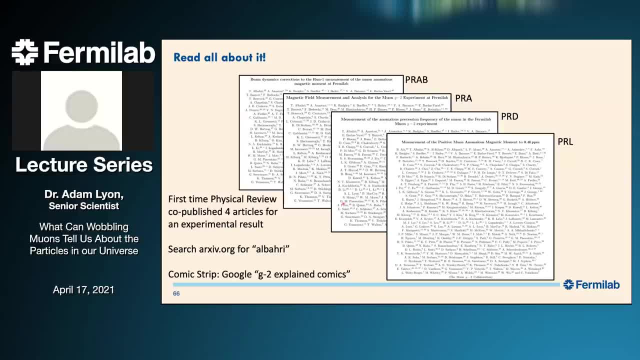 So, thank you very much. Thank you so much, Adam. This was an incredible talk. Um, we have, as you can imagine, quite a few questions from the audience, um, both here and YouTube live. Um, so I'm going to ask you, uh, uh, a bunch of questions from our audience. 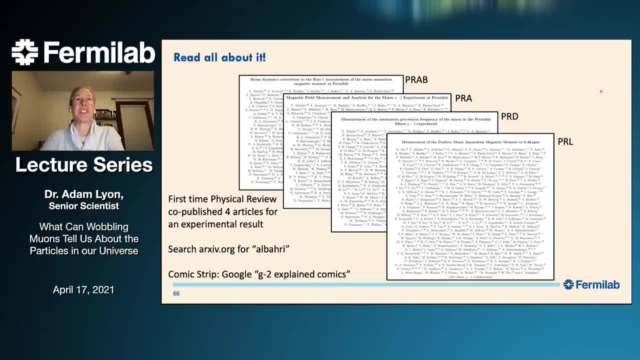 Um. so first question: could there be something systemic in the magnet Producing the results, as it's the same magnet in both experiments? um, would it have been better to build a new storage ring or um, is that a possibility? 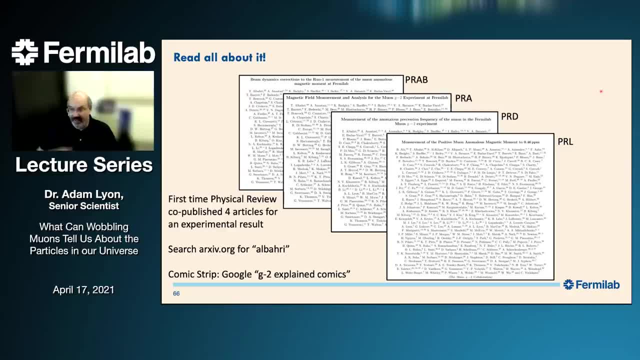 Right. So that that's a great question, And we've asked that question ourselves and and at basically at every seminar we give. someone asks this question. So it's what's a good question? Um, so yes, the, the magnet itself is the same, um, but everything else is new. 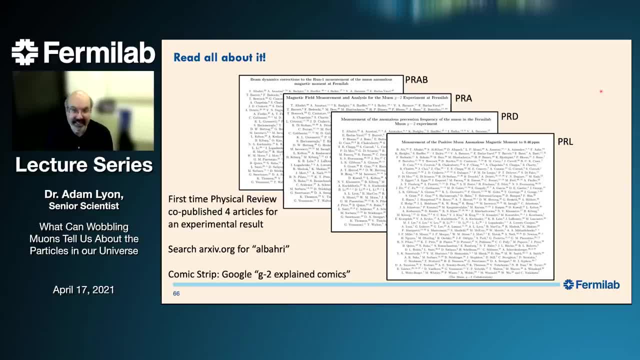 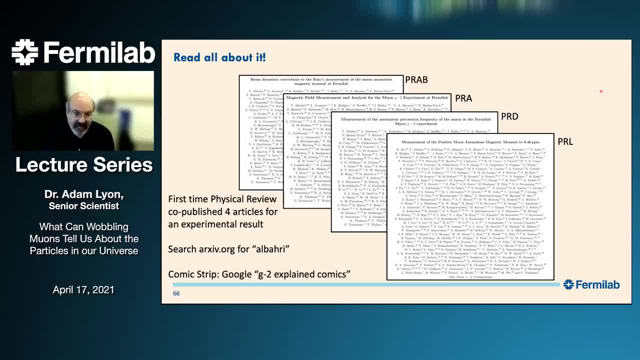 the inflector magnet, the kickers, the quadruples, those are all new, Um, and we actually we've improved upon the magnet, uh, from Brookhaven quite a bit. I I mentioned that we made the magnet very, very uniform. 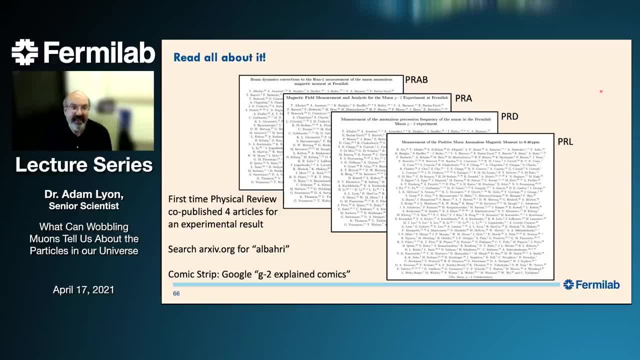 We actually did that better than Brookhaven did about three times better than Brookhaven. Um and so so we we really believe that there's there's there's really no correlation between our experiment and and the Brookhaven experiment. 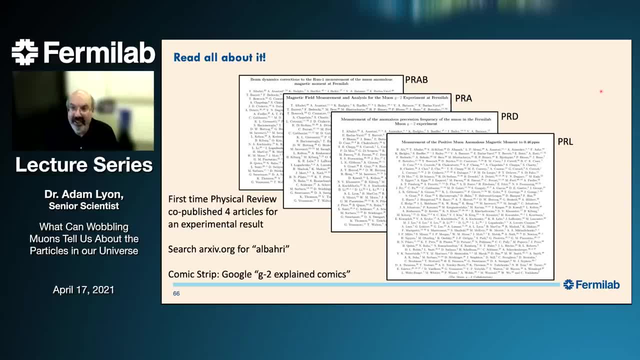 we use the same magnet. you know, the magnet itself really just supplies the magnetic field, uh, and it has, uh, the. so the strength of magnetic field of course is important, but that doesn't necessarily tie the two- you know, our experiment, their experiment- together, um, and and basically to 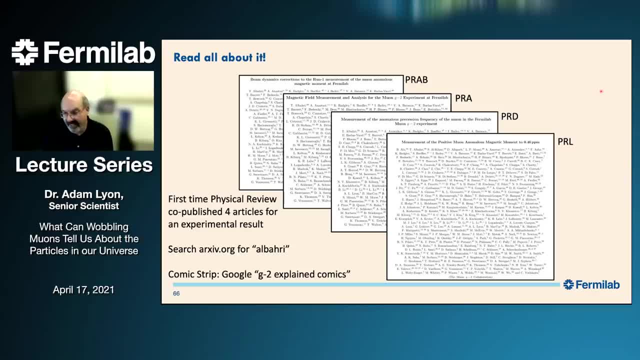 build a new storage storage ring would have been cost prohibited, we probably would not have done the experiment. you had had the the the ring fallen off the barge and sunk or something horrible like that. you know, we probably would not have done the experiment because it would have been too expensive. 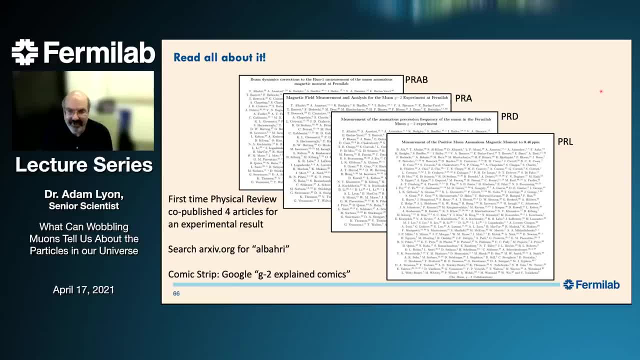 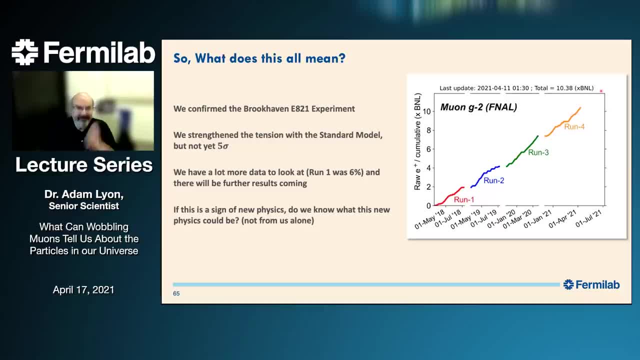 to be a lot of fun. um, i think it's going to be a lot of fun. um, i think it's going to be a lot of fun. up, what do you, what do you see? right, right. so actually i think- uh, i'm not, i'm not sure if so. 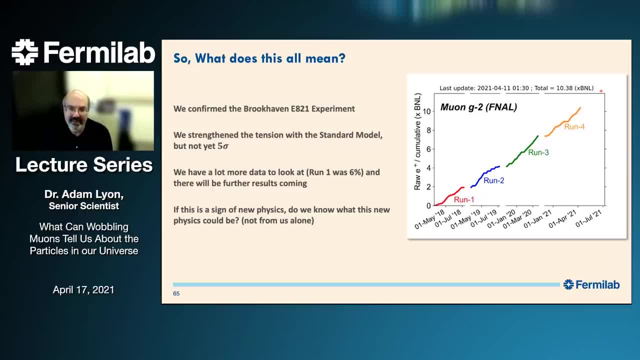 run two and run three. we think we'll get. so that should be a factor of two. better in uncertainty. um, you know, will that? you know we'll be a lot closer to five sigma. uh, will we actually reach five sigma? uh, maybe, maybe, maybe we'll be right on the edge of it. uh, certainly, you know, once we get. 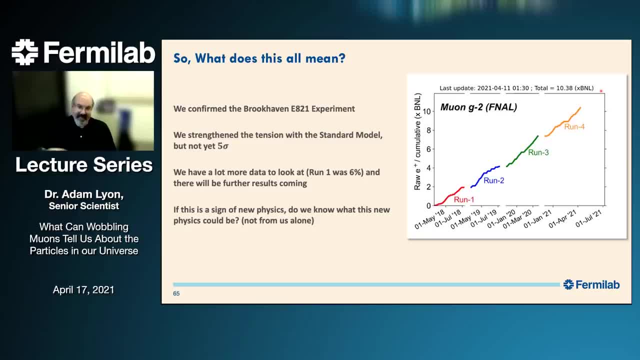 run four and run five, then then we should be. well, you know, if the result stays the same, of course, uh, uh, if we keep getting the, the answer where it is, then, yeah, i think certainly by the time we're done we'll be. you know, the plan was to be well over five. 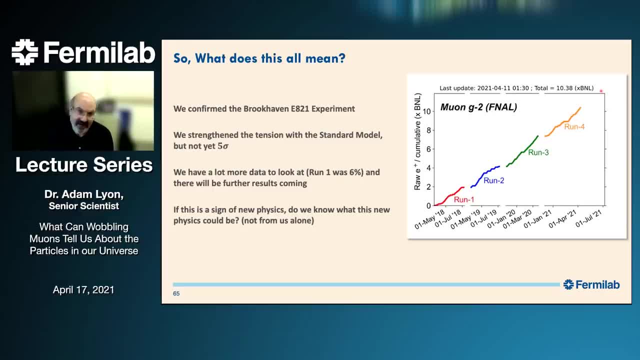 sigma, and so we should hit five sigma um somewhere along the way. i don't. i don't know if we'll get there, uh, when we analyze run two and run three, but hopefully shortly thereafter. awesome um. so from youtube live um. can this kind of experiment be done with the tau particle? excellent question. 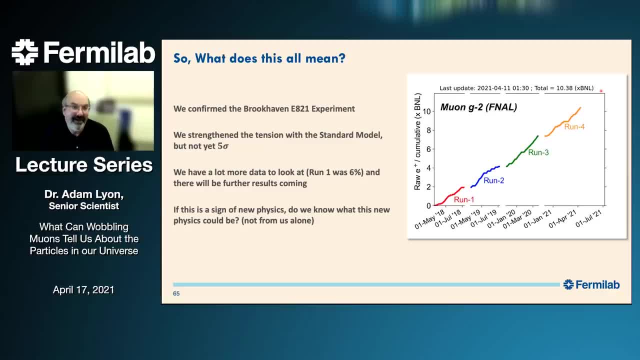 i'm so glad you answered. yes, i question so kinda in fact, um, if we could do it with the tau, it would be kind of a lot better because, um, i didn't really explain this very much- but the electron, you know. so this experiment has been done with the electron, actually to exquisite precision. uh, to part first, to solve part per. 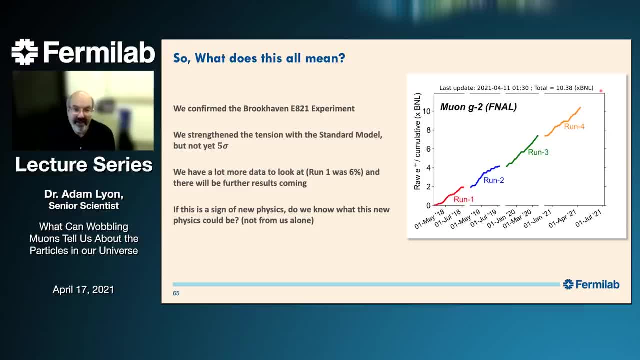 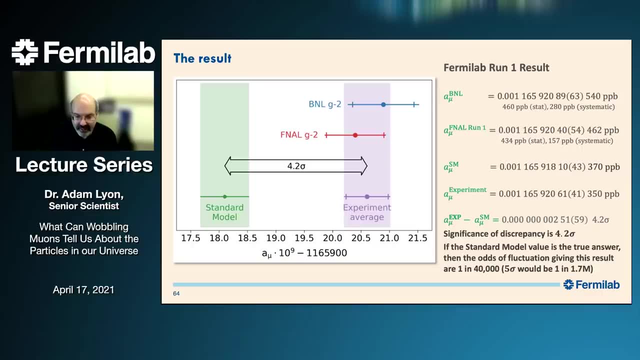 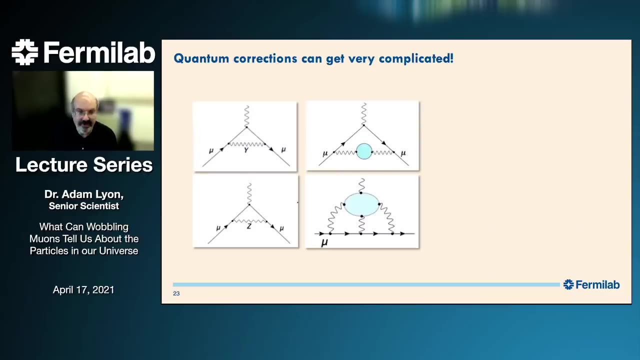 trillion precision. but the problem is that because the electron is so light, let me see if i can get back to that, to that slide. that's not working, i don't want to do that. hold on a second. uh, where was it? well, okay, there, it is okay, let me do that. okay, so, because the electron is so light, 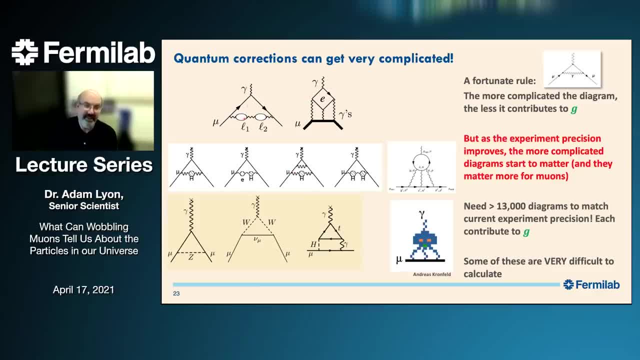 it is only really sensitive to certain types of these diagrams. uh, because the muon is heavier, it's actually more sensitive. so it's sensitive to the diagrams with quarks and the diagrams with the z and w goes on. the electron is much less sensitive to those. a tau will be even more sensitive to stuff. 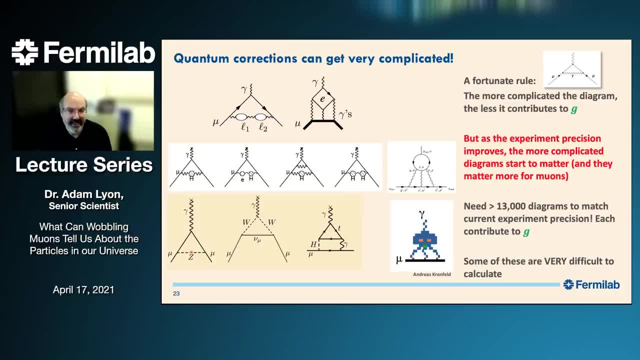 is that they're very hard to make. Well, actually that's not true. We can make towels. They're not made as copiously as muons, So they are hard to make and they live for an incredibly short period of time. 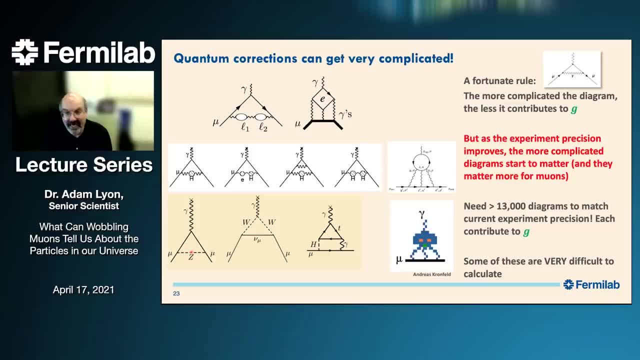 They live for something like 10 to the minus 13 seconds, And so when you have a particle that lives for microseconds or hundreds of microseconds, that's easy for electronics to deal with. Electronics can deal with things at the microsecond scale very, very easily. 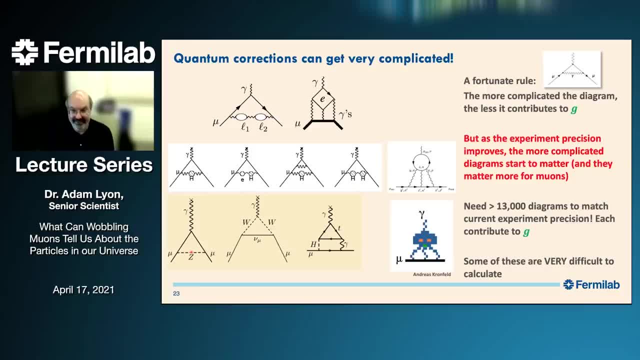 But when you're talking about sub-femtosecond, which is 10 to the minus 12 is a femtosecond- we're talking faster than that- then that's very, very difficult to do. So, no, so no one really knows how to do this with towels. 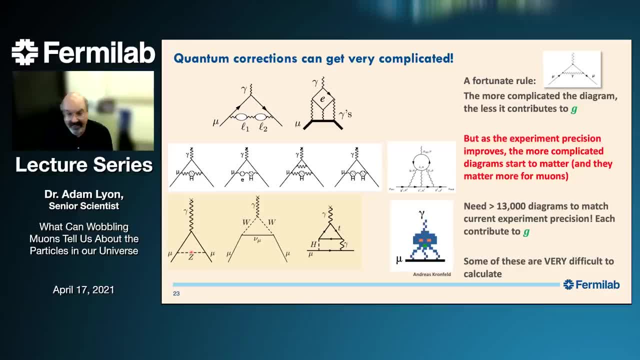 in a way that would work. If we could, that would be great, but that would be an incredibly difficult experiment to do. So we had one question about the data. How is this experiment's data stored? How much data is gathered for? 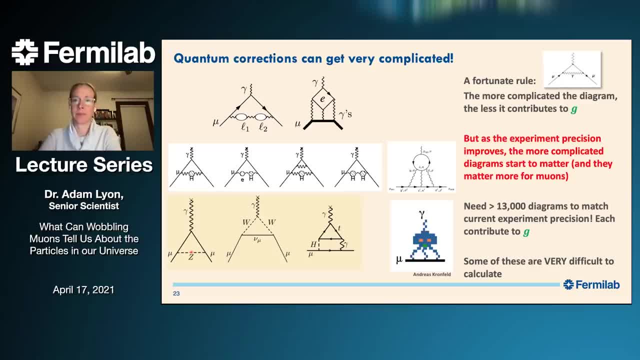 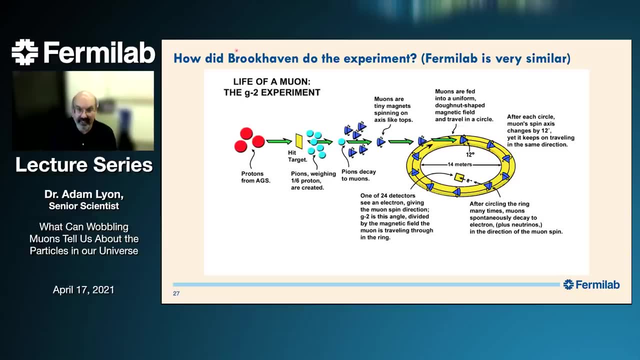 and how much data is gathered for each of the runs. Okay, so I'm trying to remember. So I said it was about 8.2 billion positrons for run one and run two and run three. have a little more than that. 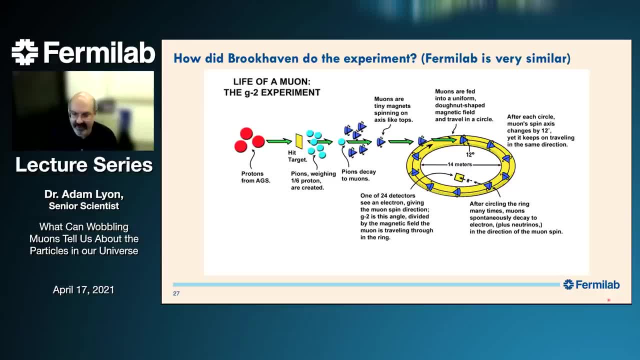 So it's probably- I don't know. I don't know what the actual number is. I'll guess it's around 10 billion each, maybe a little more for each of those runs. Let me get to that plot again. That's what I'm trying to do here. 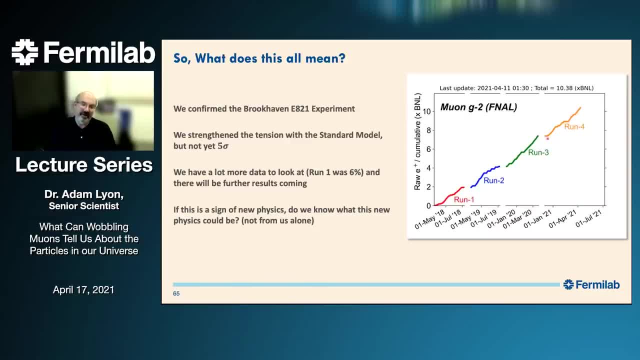 Oh, I just missed it. There it is. Yeah, so run two and run three are quite a bit longer and have a lot more data, So they'll probably have. I don't know the answer, I'll stop my head, but they'll have. 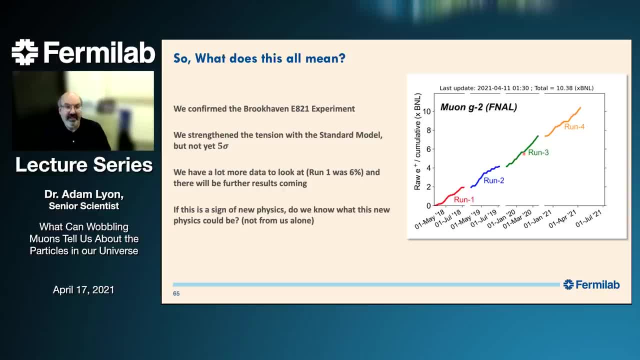 you know, hopefully 30 or so billion positrons, So runs one, two and three. if you want to know about how much data this takes about, I'm trying to think four or five petabytes of data, maybe more, maybe. 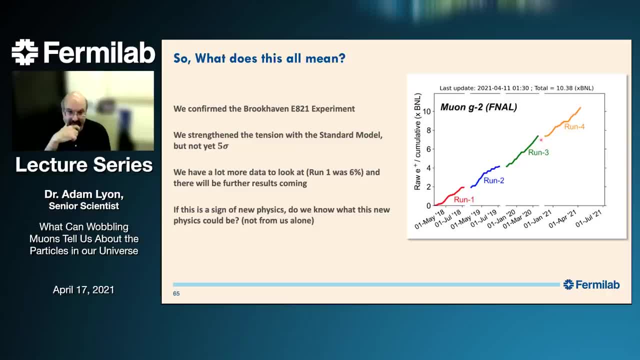 They actually now have about eight petabytes of data. So that's a lot of data that we store. So that's a lot of data on tape at Fermilab for this experiment. Hopefully that answers the question. Yes, So another question: what is your current favorite? 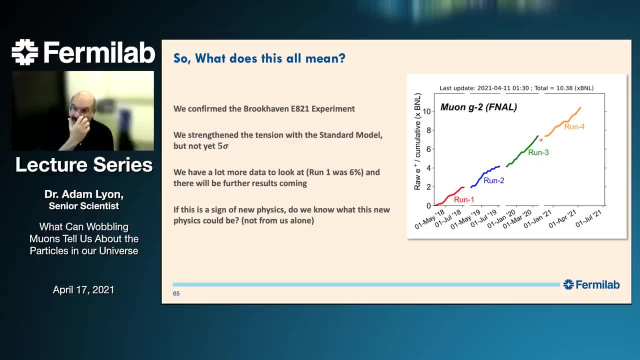 explanation of the difference between theory and measurement. All right, so I'm not going to give you a fun answer As an experimentalist. we see, actually it's very interesting, The theorists themselves are trying to figure out which bottles could be compatible. 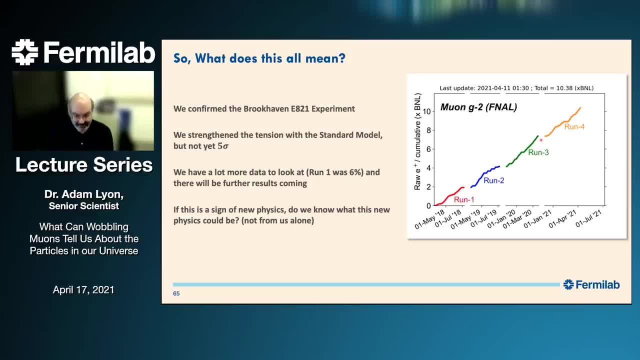 and there are many. I don't have a personal favorite. I mean supersymmetry would be fun because I was involved in a supersymmetry search when I was a grad student And there's just a lot of experiments that have been looking for supersymmetry. 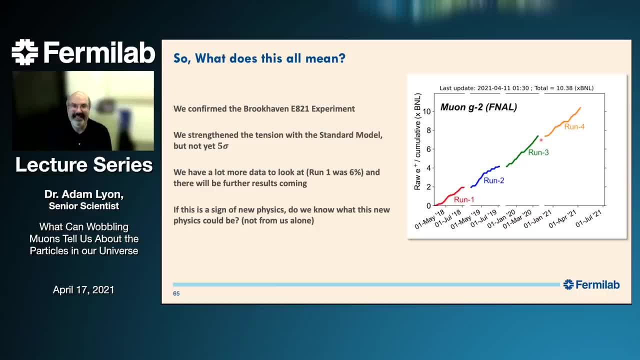 And so far it's eluded the LHC, if it does exist, And so that's sort of been a puzzle. So it would be great if it were supersymmetry, but it would be great if it would be anything else. 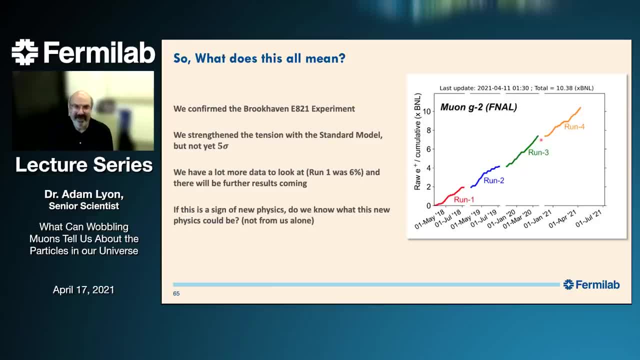 So I think it's not that I would prefer one or another. It would be great to know right. That's really what we're hoping for, And once we do know, once we get to the point where maybe the LHC has seen something, 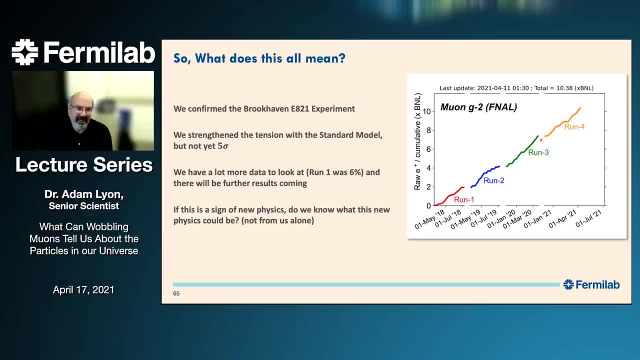 or we have a much bigger discrepancy and other experiments are starting to see hints and we get a better picture of what the theory is. that's beyond the Stearn model. You know that doesn't necessarily mean the Stearn model is wrong. 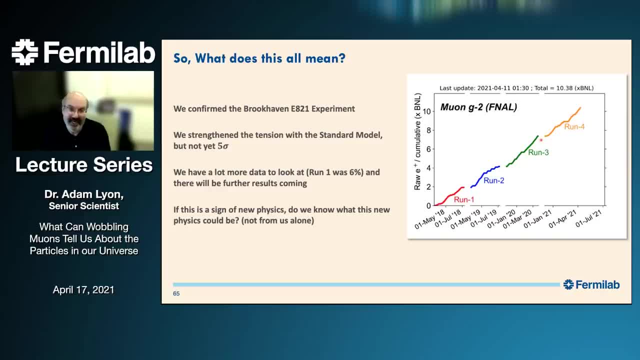 It just means that it's a piece of a bigger picture and we will have learned more, right? So that's what we want to do. We want to learn more. We know the Stearn model is an incredible theory. It predicts so many things. 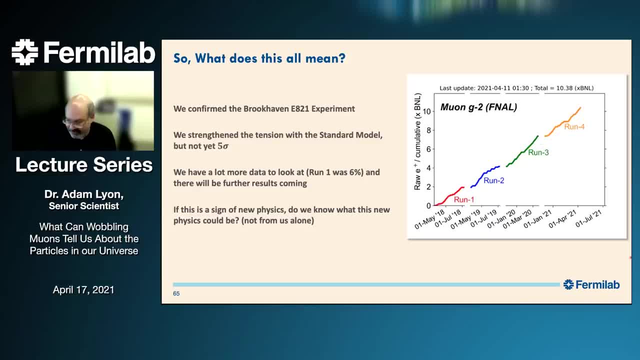 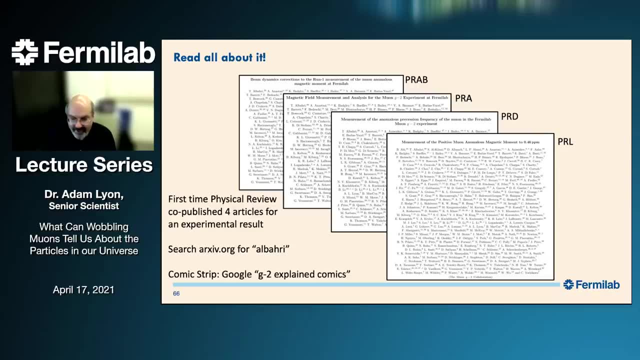 I don't have actually here, I will, since you asked the question, I can. So in making this talk- and actually my talk came out to be twice as long as I wanted- long as I wanted- So I had to get rid of a lot of slides, So I can actually show you one now. 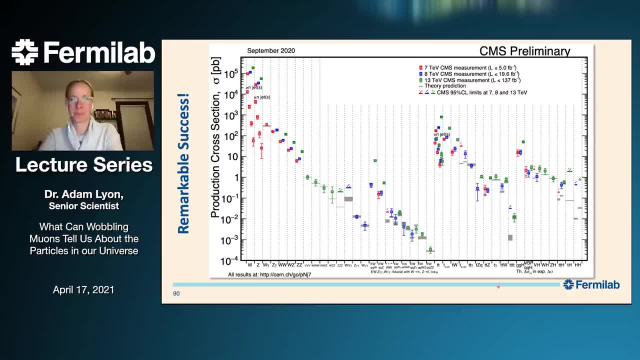 Okay, I think you can see this one. So this is a plot from the CMS experiment. There are many formula people who work on CMS. This is at the LHC at CERN in Europe, And so this is, you know, many, many, many, many analyses looking for standard model particles. So that's kind of the 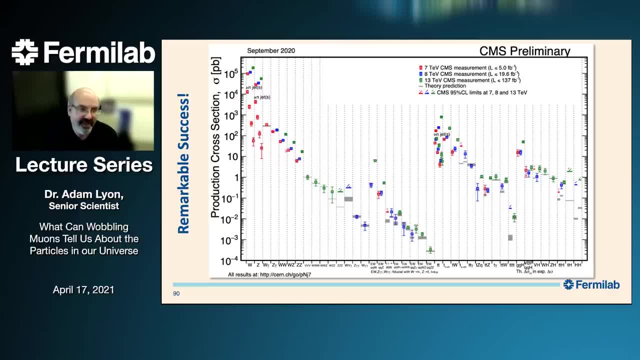 dots are the rate that these particles are produced in the LHC or in the experiment. The CERN model can predict this, And so the gray bars are the prediction and the dots are what this experiment measures. And a lot of times you can't even see the gray bars because the dots are right. 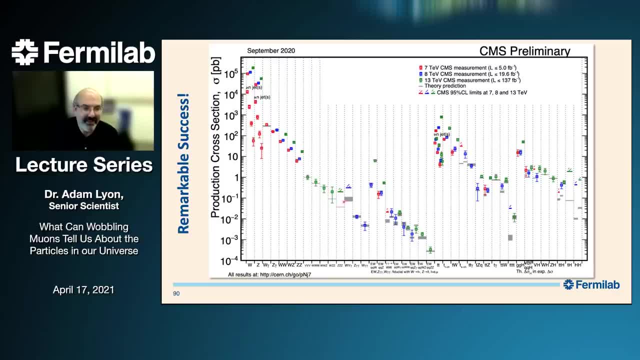 on top. Sometimes the dots are within the error bars, Sometimes the gray bar is below this weird thing here, And this is actually a limit. This is a so triple Z, So looking for three bosons, that's. that's something the LHC hasn't seen. 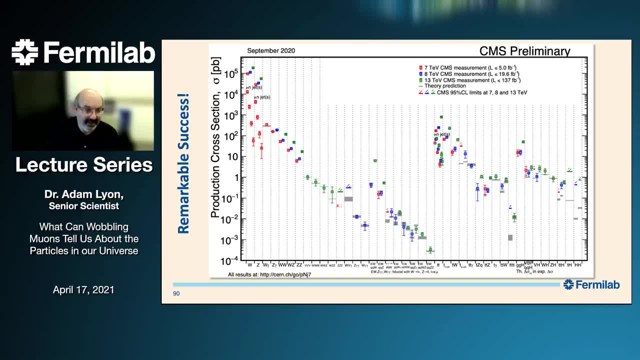 Or that, or CMS hasn't seen yet, because the the value of the rate that that it's predicted is too too low, too rare for what the LHC can produce right now. Right, So they set a limit. But this, this, this whole plot here is nine orders of magnitude here. This is an incredible. 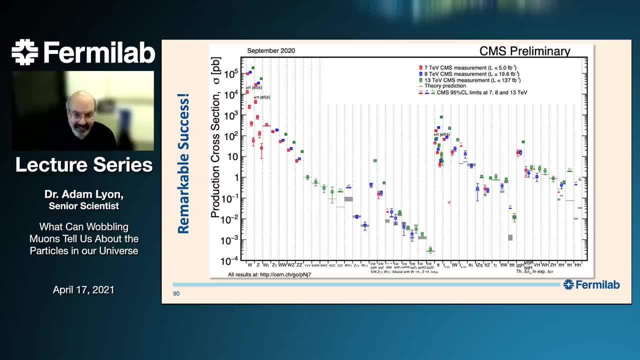 plot, because basically, it shows how strong the standard model is, that all of these predictions are basically correct. So this is an amazing thing And this is why it's so hard to look beyond the standard model, because the standard model works Well, even though we have these ideas, we have these, these things. we wish the standard model. 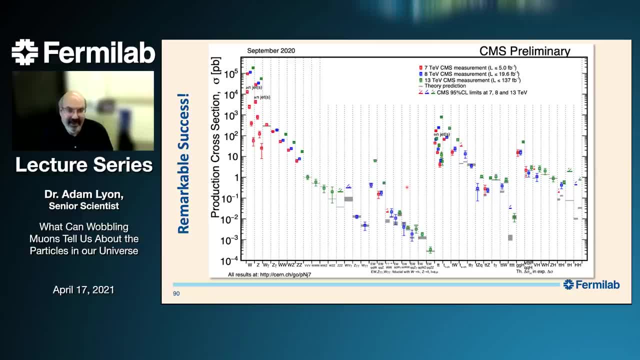 would do that. it doesn't. you know what it does do. it does incredibly well, And there are very, very small number of experiments like ours, like G minus two, that has a hint of something weird going on Right, And no, no one has a hint above five Sigma. So so, yeah, So so, thank you. 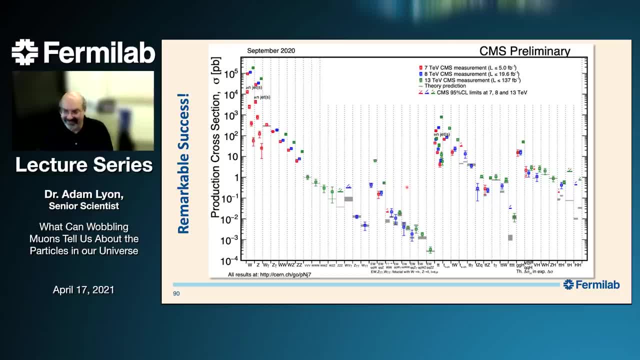 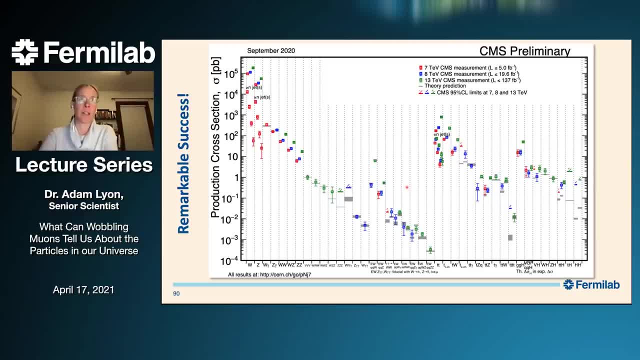 the anomalous frequency indicates something beyond the standard model and not just a need for some fine tuning to the thousands of diagrams from the standard model contributions. Ah, that is a great question, Right? So could there be a mistake in or something else going? 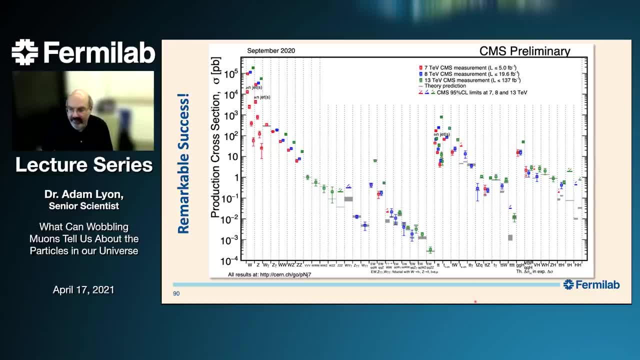 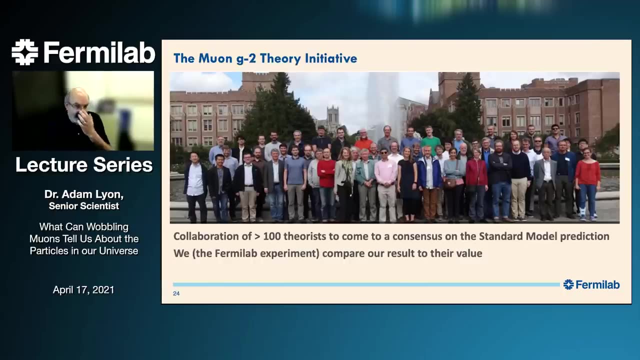 on in the standard model prediction. I don't have it in this talk, unfortunately. So this, this, this, this muon G minus two theory initiative. let me find their picture again Here. they are Right. So there's, there's, there's over a hundred theorists here. 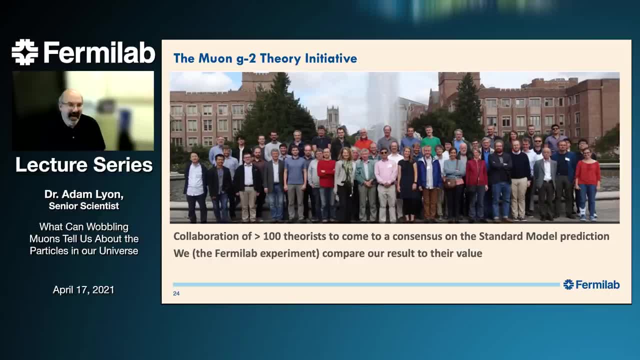 Some of them work alone, Some of them work in small groups, And they they've all produced pieces of the standard model prediction. So so, calculating what these diagrams contribute to, G minus two, as I mentioned, some of them are very difficult to to calculate, And so they. 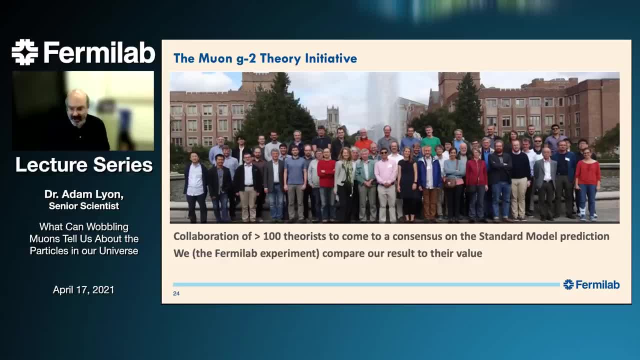 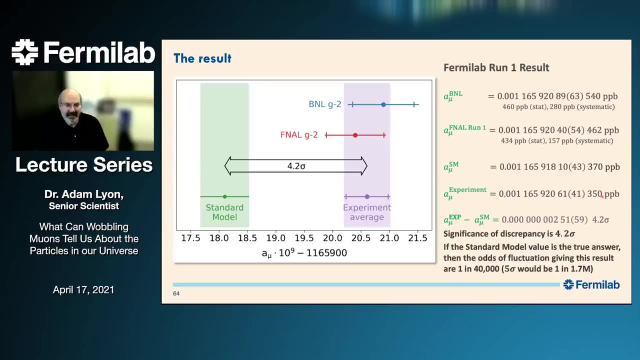 sometimes they calculate them different ways And they they put all that together, But if you look carefully you notice that the theory value had an uncertainty as well. So they evaluate all these different ways of coming up with these calculations and they look to see. you know how they're slightly different. if they're agree, if they don't. 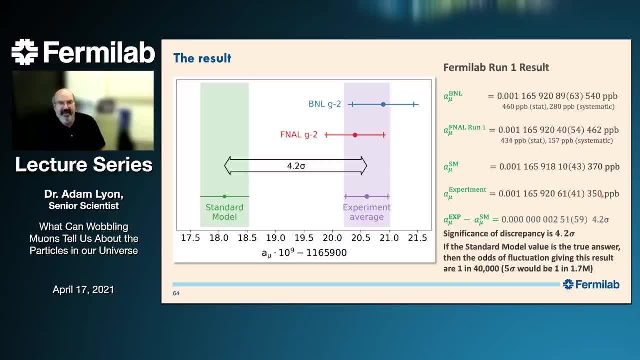 agree, you know- and they assign uncertainties- we'll call it systematic uncertainty- based on the level of agreement, And they come up with a very small uncertainty. So so this is the error bar That they put on on this value And that takes into account sort of all the different ways of 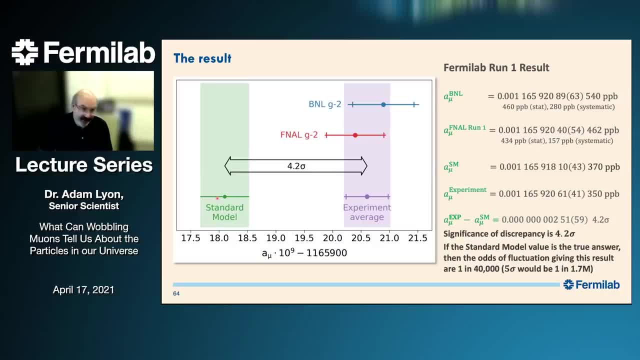 doing this, these calculations. Now, to be fair, there are some new, very new calculations that are being done with a technique called lattice QCD. So some of these diagrams can be calculated in a new way with this, with this technique. the technique itself is not that new at all. 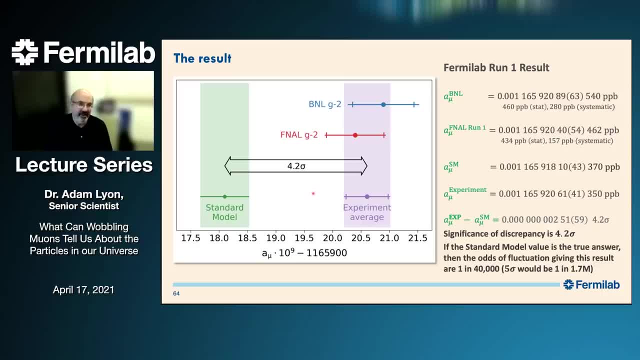 but it's being applied to G minus two In a way. that kind of pushes this technique to its limit, And so they they're producing- I don't have the plot here, but they're producing- results that are more pushed out to the right. 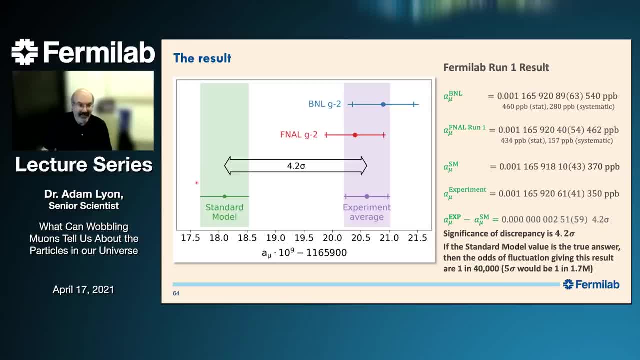 but a lot of them have very large error bars that could you know. basically they overlap. you know everything, So you can't really say what they're saying. They're not included in this, in this average, because they're they're very new and they need to be evaluated. 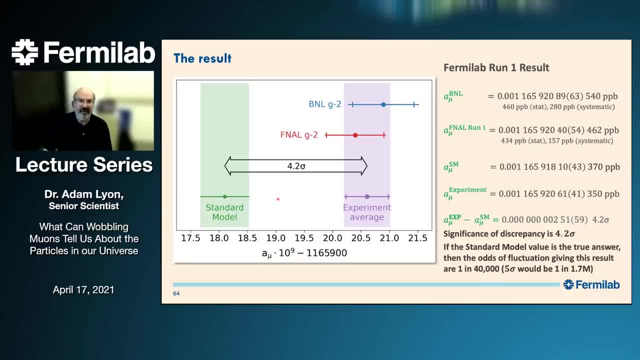 There is a new result from lattice QCD, from one from one group which is more over here story the experimental value, And that's very interesting. They are claiming that they understand how their calculation works to a very high level of accuracy. but that has to be scrutinized and it's very, it's very new. 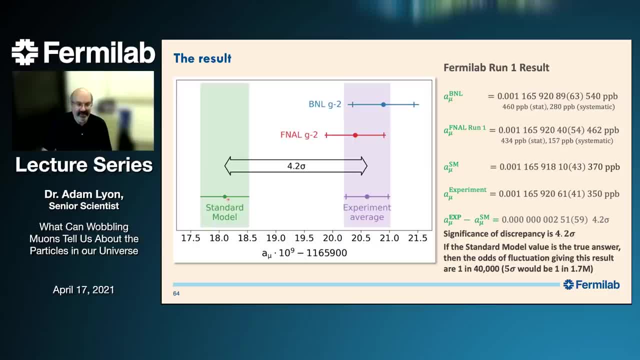 And so actually it was so new that the that it came out after this value was determined- And this was a few. this was determined a few months ago, So this, this thing, is so new that it hasn't been. Is this the result of skip analysis that we're saying yesterday? 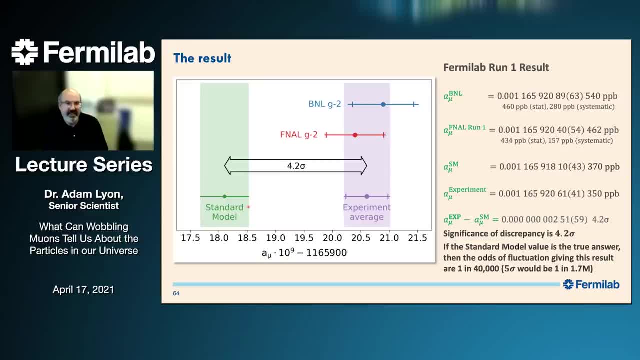 That hasn't been the result. And then look, you can see we're not seeingede civilians in it Like this doesn't look very good, but I think we've gone down a battle here, looked at very closely yet by the muon g minus two initiative, so i think they're going to be. 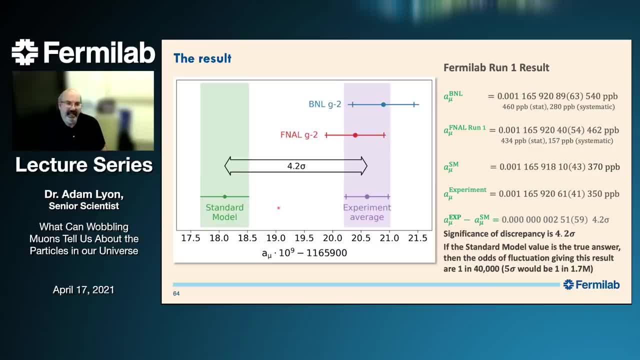 very busy over the next year. uh, lattice qcd does involve a lot of assumptions and there are some places, there's some regimes where it works really well and there's some regimes where it doesn't work very well, and so you know if groups are claiming it works very well in lots of regions. 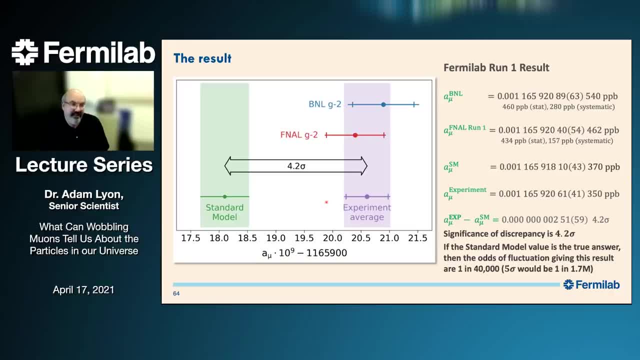 you know, that's something that has to be looked at and this is how you know, this is how science works, right? uh, you know, someone pushes, pushes things to the edge and gets a result, uh, and then it has to be scrutinized by the community and, uh, and over time, you know, the community will either. 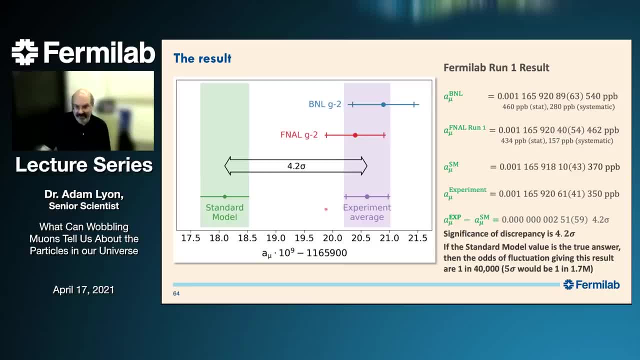 believe it and, and maybe you know that'll push the standard model value over to the right, or maybe they'll find uh, something that's that uh, that was overlooked for a reason to doubt the new reason, the new, these new uh calculations, and it'll stay down here. so we'll just have to see. uh, i think you. 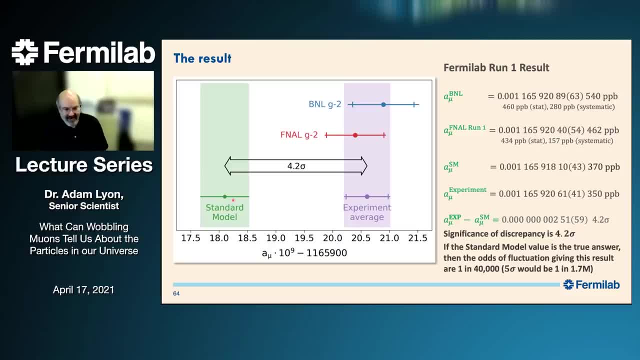 know, as we're, as we're busy doing, you know, analyzing run two and run three and taking run four, uh, the the stamp, the me on gmi2 initiative will be very busy evaluating uh these, these new latest qct results, because they are in conflict with techniques that have they've been doing for 20 years. uh, and so, even if it turns, 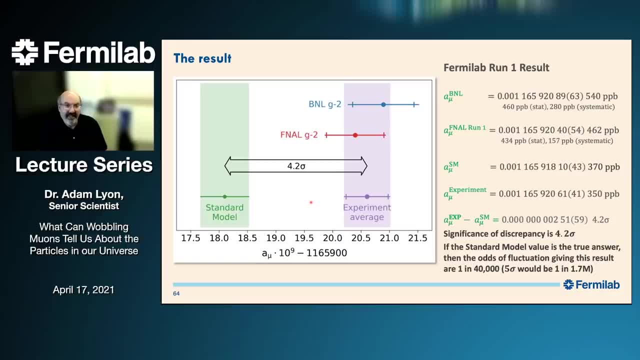 out that these last qc results are more correct, then then they have to explain why these long established results are wrong. what's wrong with them? because now there's a tension within the standard model. that has to be, that has to be, uh, understood. so so, no matter what happens, we'll. 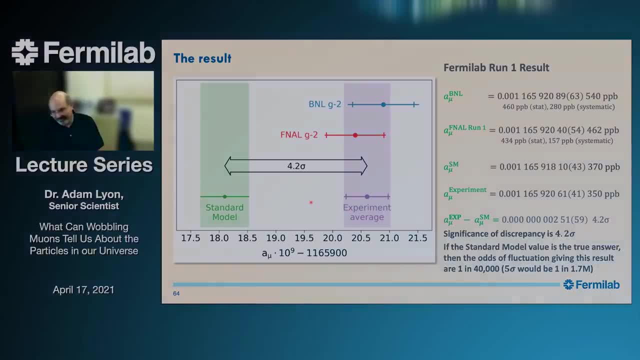 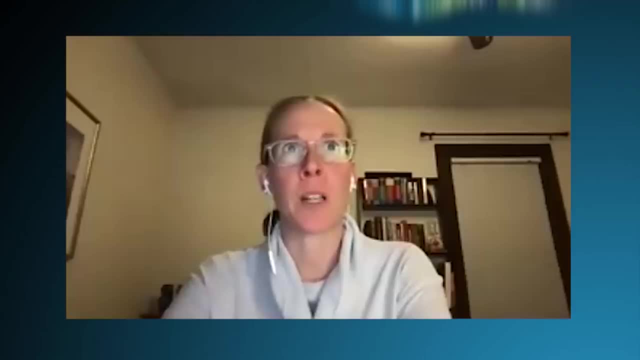 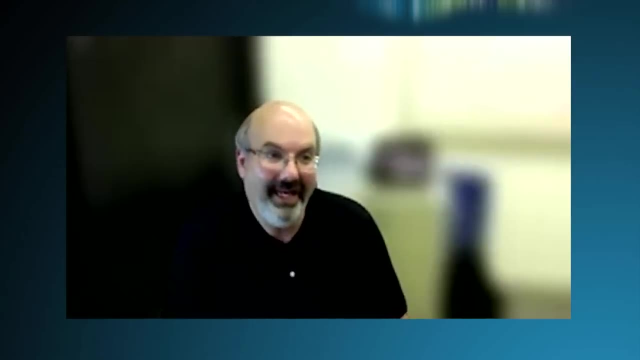 learn something new. so that's that's what i want to say in the end. so what are your thoughts about the possible relationship to dark matter, as the news has talked about this? um, is it just wild speculation or is it justified? um, so i i think, i think there's something in between justified and. 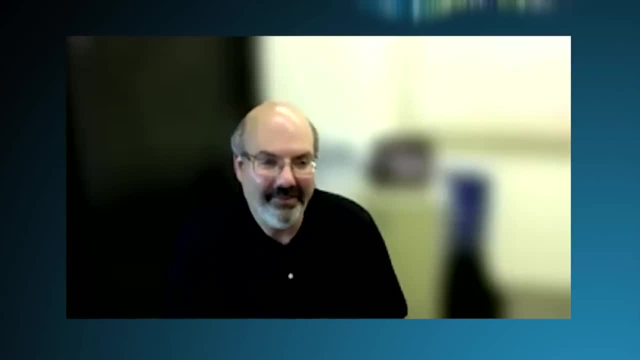 wild speculation, right so. so, as i said, um, there are lots of models that are compatible with uh, with muon g minus, with our value for muon g minus two endless discrepancy: uh, dark matter models. some of them are compatible, so it could be dark matter. uh, it could be other particles called leptoparks. it could be super. 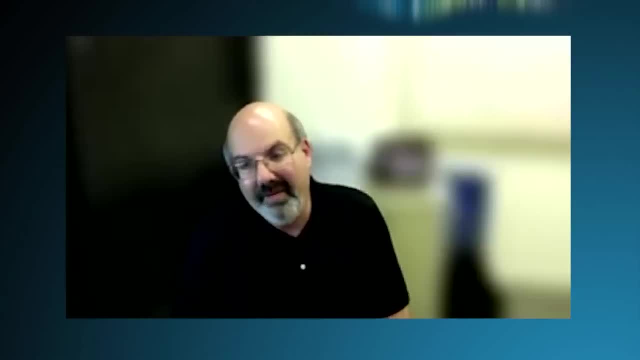 symmetric particles and we just don't know. you know, like i said, we we really won't, we can't determine that from our experiment alone. uh, we need hints from hopefully, you know, hopefully the lhc will start seeing some hints, uh, uh, or other experiments will start. 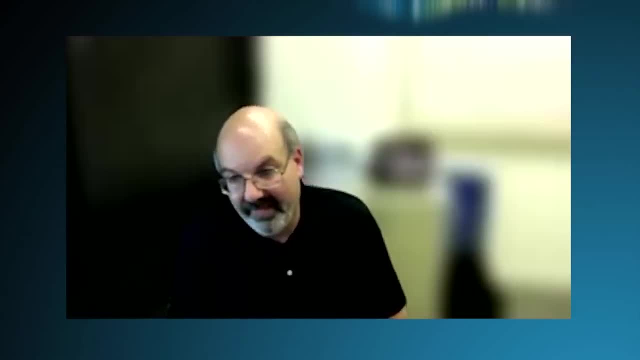 showing some hints, or we'll need to to to have new experiments that are even more sensitive, uh, and and maybe that'll point us along the way. so so, so, guiding to an answer like that is difficult at this time, uh, but you know, we're starting to sort of shine light on things and right now the 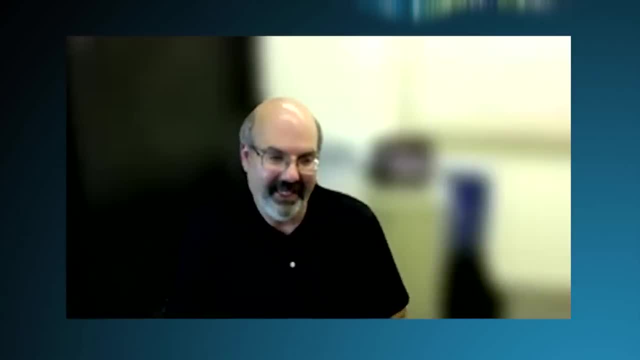 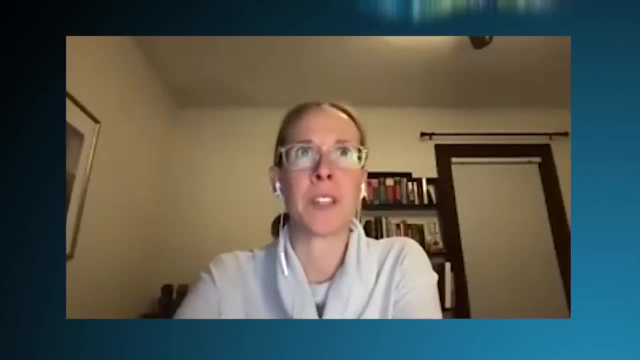 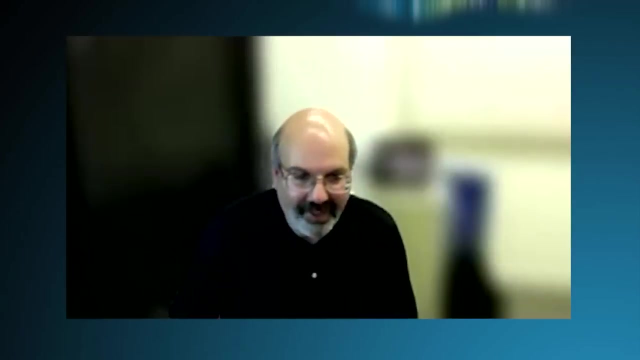 spotlight is very broad, uh, but maybe with other experiments it can be narrowed in the future. um, so we have a few practical questions. um, as the magnetic field is measured every three days, how much variation is seen over time? that's a great question. uh, i can show you this. uh, where to go. 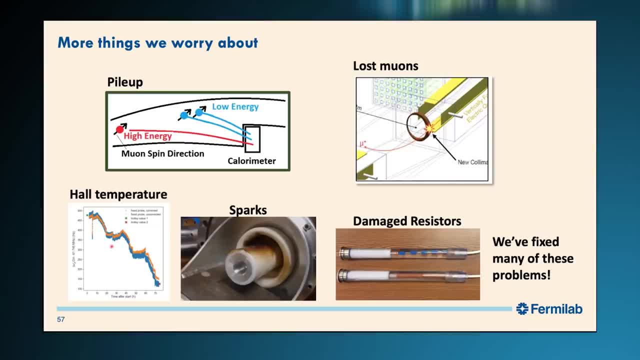 here it is. so that's a great question. so so we actually care about the magnetic field where the muons are, and to do that, uh, we have to run this trolley around the ring and actually we have a little camera we can see the trolley go by. it's really cool, um. 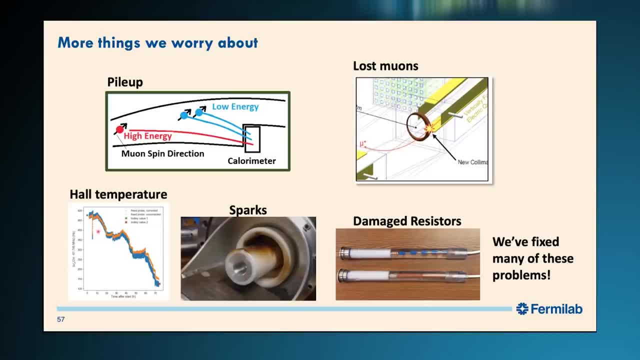 but but yeah, so the magnetic field between those three days does change and that's mostly because for run one, uh, we had a hard time controlling the temperature of the hall. so this sort of shows them the changing magnetic field over those three days that we can measure with these embedded probes in. 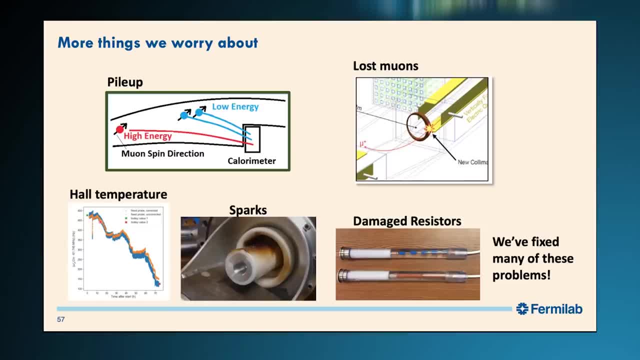 the ring and that's really what they're for. uh, so we have, i think, 300 and some probes around the ring. they're fixed in the ring, uh, and they're measuring how the magnetic field changes in the trolley run. so the trolley runs are kind of the very precise measurement, uh, and that's every. 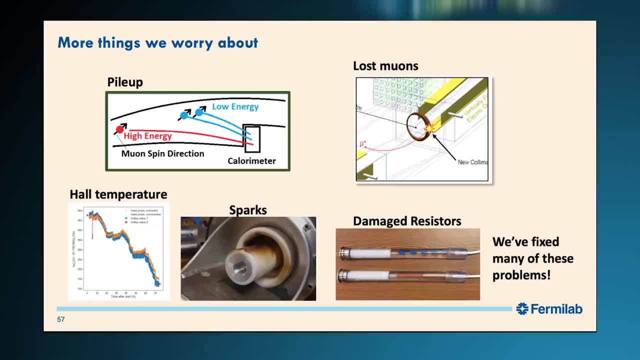 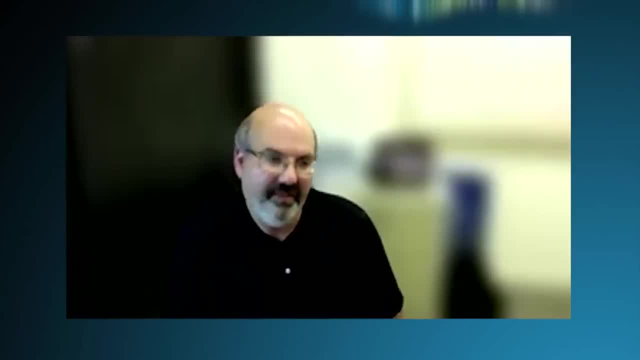 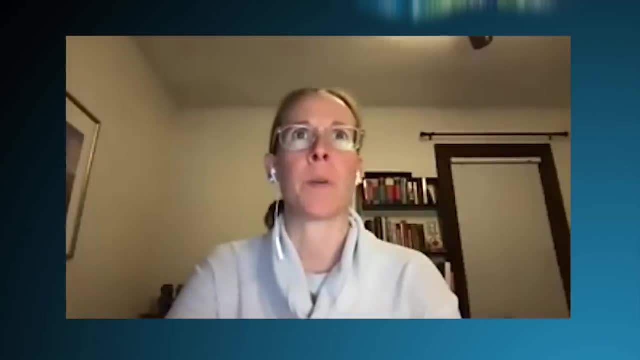 three days and then we use these fixed probes to get from one three-day measurement to the next three-day measurement so we can determine what what the ring was doing in that intervening time. so these fixed probes really make it so that we can do that awesome. um, so when you kick the muons so they won't crash into the ring wall, does this affect? 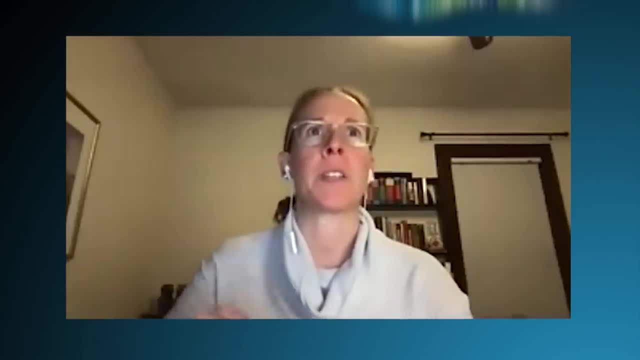 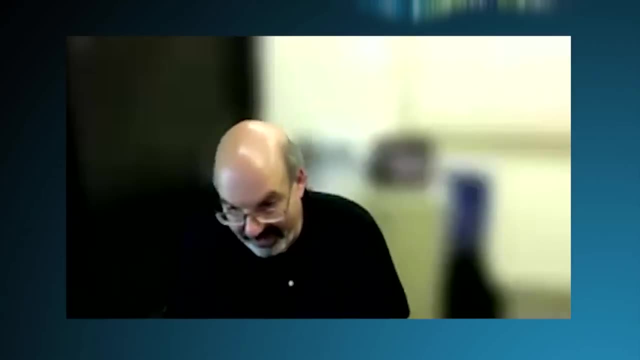 their spin. um and uh, how do we know things in place to focus, um and kick the muons and ones into a focused beam are not affecting the results. that's a great. that's another great question. uh, the the kick is incredibly short, so if it does change the spin, it doesn't change it. 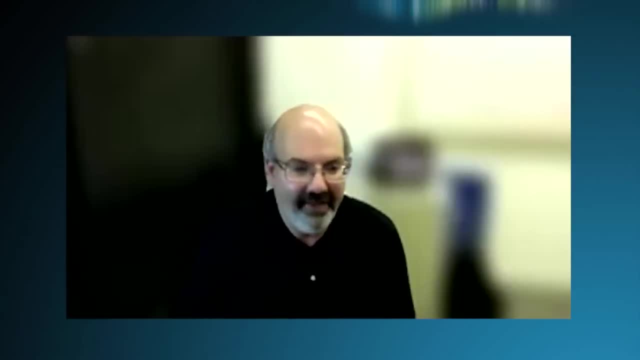 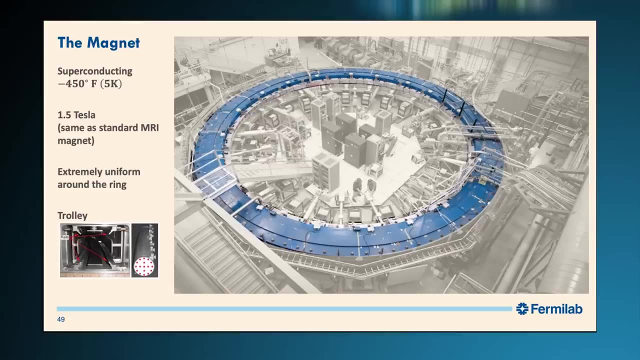 very much um, the uh. i don't have it in this talk, but there is actually something neat that happens. so, yes, the uh, the quadruples do change the spin, um, but we can actually minimize that effect by choosing a very particular momentum or energy for our muons. so it turns out there's something called the magic momentum, and if you 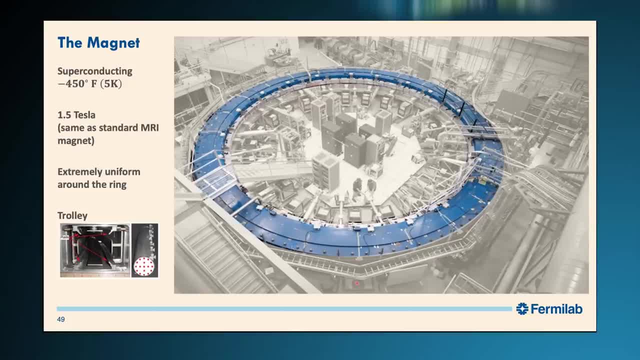 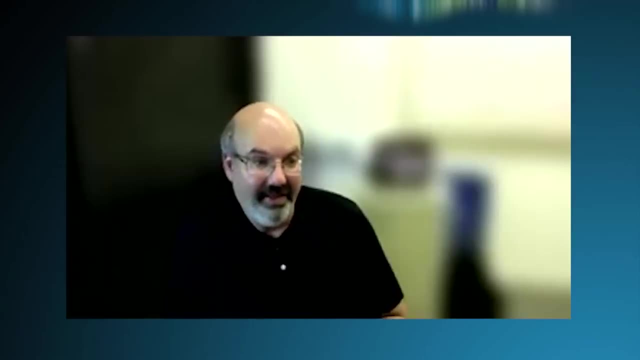 if the muons are going around the ring at 3.09 gev, that's the magic momentum. then that minimizes the effect of the of the field from the quadruples. it doesn't, so it actually, it actually. if you choose this exactly right momentum, then the muons really don't feel the um, uh, the the they're not. 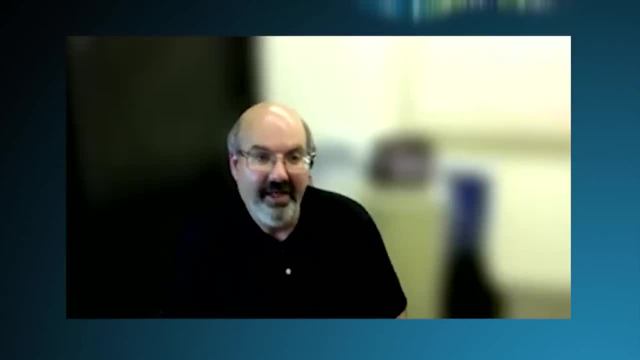 affected by the quadruples. so it's not affected by the quadruples, so it's not affected by the quadruples. now the problem we have is that, you know, most of the muons are going. a lot of the muons are going around 3.09, but a lot of them are not exactly 3.09, some of them are a little off. 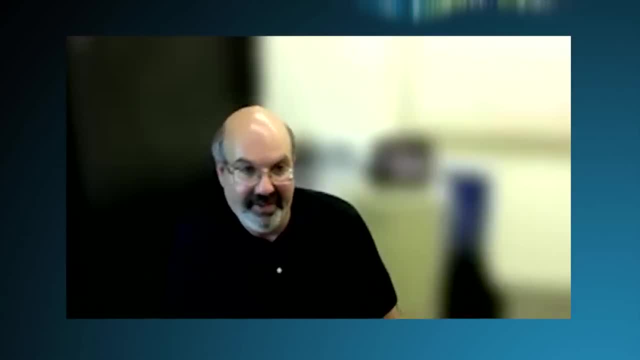 uh, so there's always a range of momentum. they're very close, they're within, i think, 0.15 percent of 3.09, but that's enough that we have to worry about it. so we actually have a correction, we can calculate, we can look at where the muons are in the ring and that gives us, that tells us. 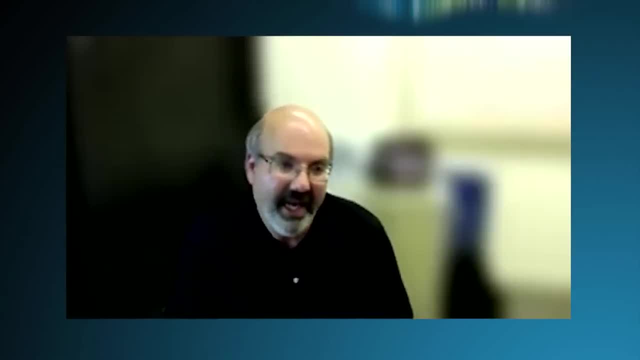 what the momentum distribution is of the muons, and from that we can calculate a correction for this effect. um, there's actually another correction, uh, because the quad, the quadruples, you'll focus vertically. that does set up a little vertical oscillation of the beam, and so the muons might not, uh, decay depositrons in the horizontal plane. they might. 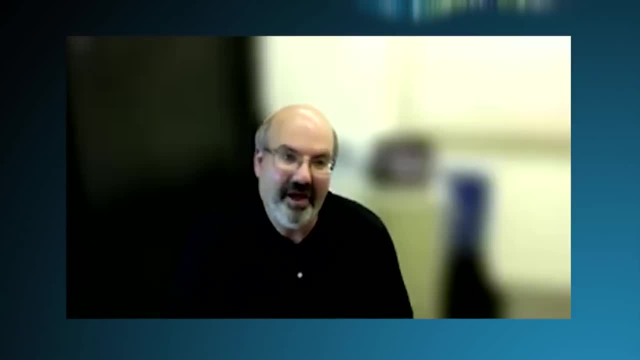 be tilted up a little bit or tilt it down a little bit, uh, and that's called the pitch, and there actually is a pitch correction that we make. we can figure that out, uh, and we can correct for that and uh, and assign uncertainties to that as well. so those are actually long-standing corrections. 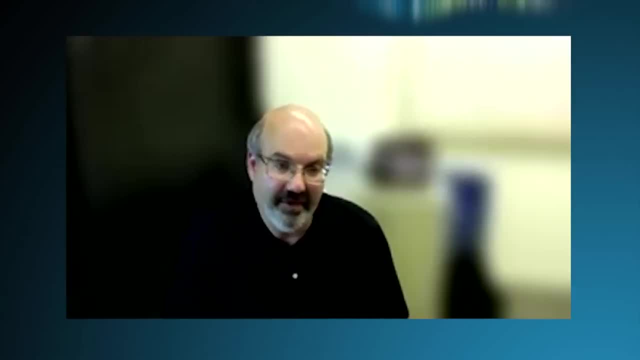 brookhaven did them too, uh, and so they're, they're, they're, so we know how to do them and we know how to estimate their uncertainties and so, and so we do all that. so, yeah, so that's a good question, and we know how to deal. we know how to deal with the effects of parts of the ring that that could. 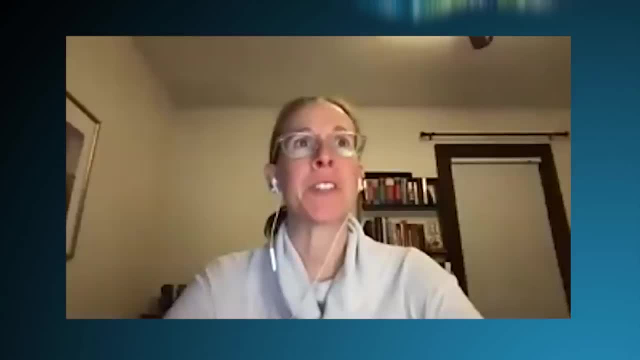 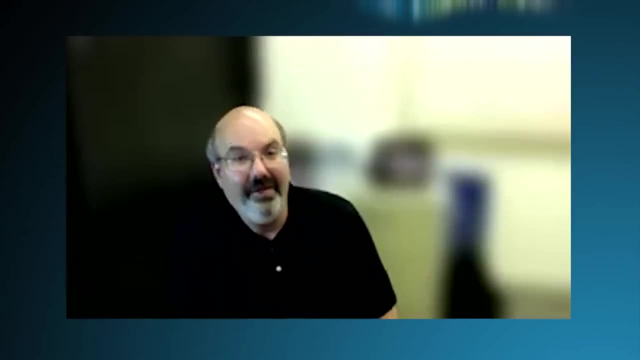 potentially change the spin. um, so does the ring make much sound when it's working? huh is a good, so not really so. so you, you can't be inside the hall when the ring, when the ring has muons. uh, because there is there is already, there is potential for radiation, and so we have a we. 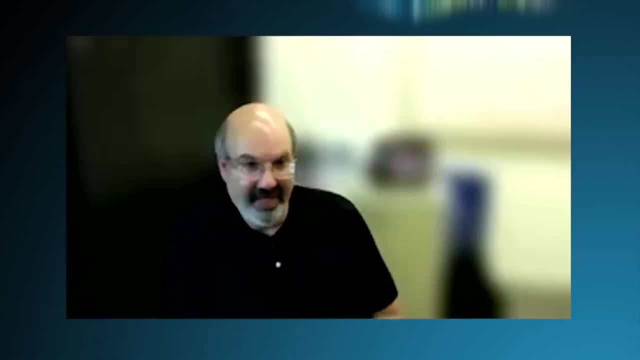 have a kind of a uh elaborate safety system, an interlocking system, so no one can be inside the hall, so you can't be in this picture, when, when we actually have beam, uh in the ring, um, we do. it's kind of funny, uh, like i mentioned, sparks uh, so sometimes some of the kicker plate. 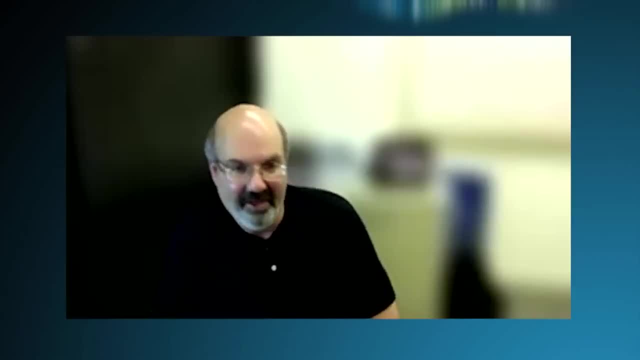 and some of the quad plates can spark. uh, that's actually not so good. we don't want that to happen. uh. and for the kicker, we actually uh, sometimes those can be heard, and so we actually have a baby monitor, uh, next to the kickers. uh, that's tied into computers in the control room, uh, and so we 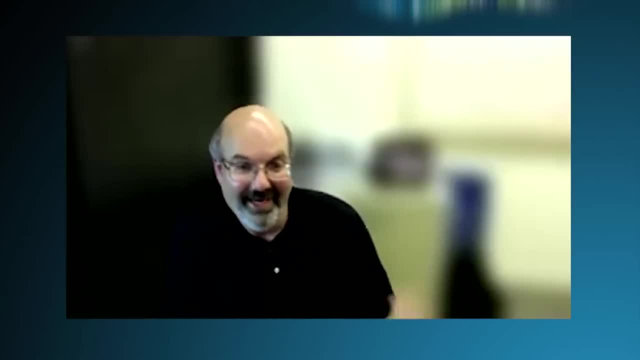 can actually, if the kickers spark- which fortunately is very rare- we can actually hear them spark on these baby monitors. it's really kind of funny, uh, but we have other ways of detecting the sparks as well. it's sort of a backup last year, you know, especially because i'm personally working on the 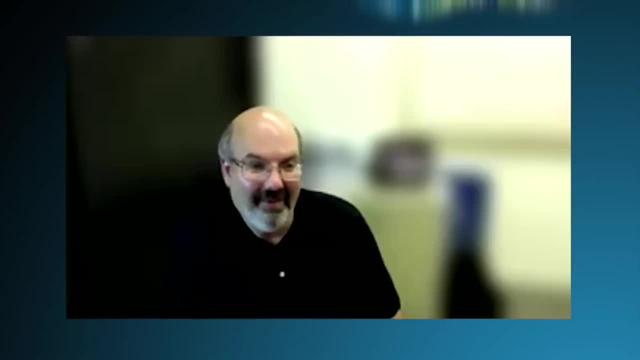 resort way of detecting these sparks, But really on the whole. I mean there's fans running for all these electronics, there's fans in the hall, So you just kind of hear a hum of stuff. You don't really hear things whooshing around in the ring, But the baby monitor is kind of fun. 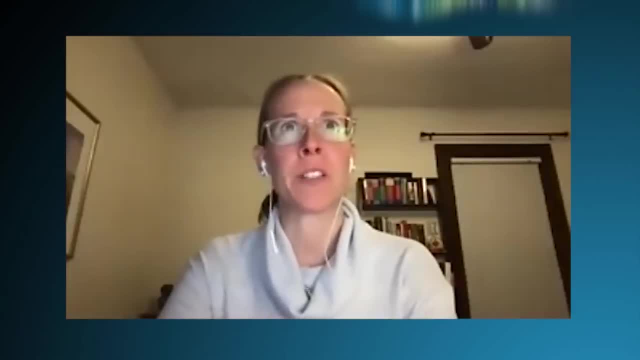 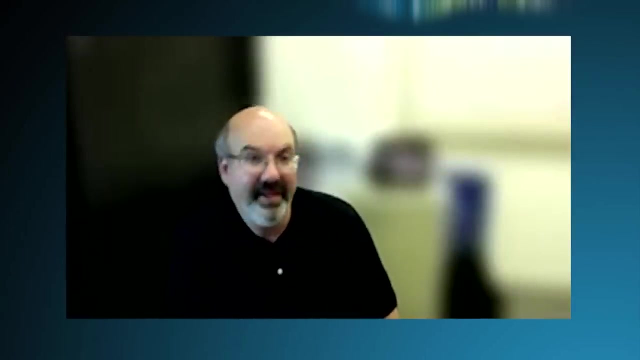 So is it possible that the five sigma requirement is too high a threshold given the intrinsic uncertainty of what you're trying to measure, as suggested by the standard model? That's a good question, Interesting question. So no, So five sigma is really the. 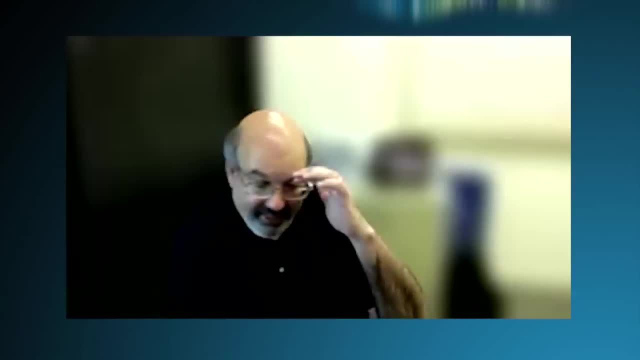 standard for experimental particle physics. I think it's also for other areas of physics as well. It's a long established standard And really you strive for that result. So you try to take enough data and maybe it takes years to get there, But you do. And let me, I have a slide. 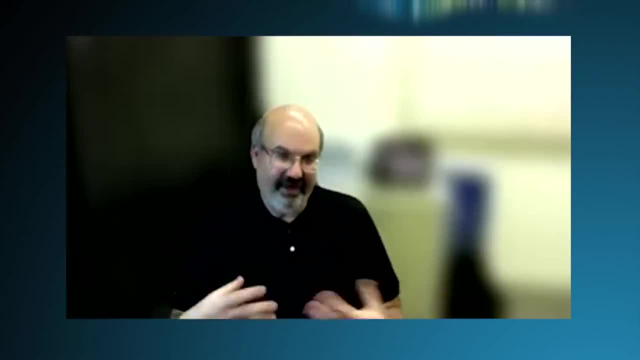 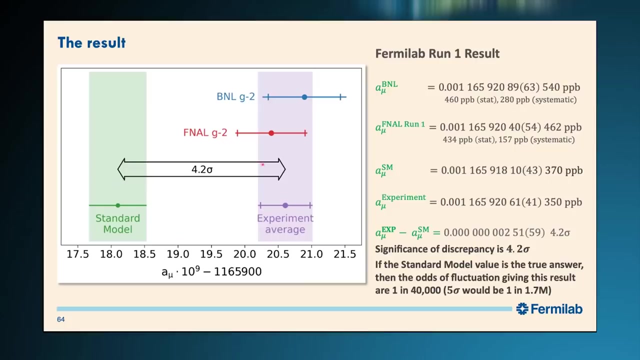 that actually. Well, maybe I won't show that slide, But to try to explain what that means. So, basically, what you're worried about is: could the actual value- Let me get there- Could the true value really be the standard model value? And what you're seeing is an unlucky statistical fluctuation. 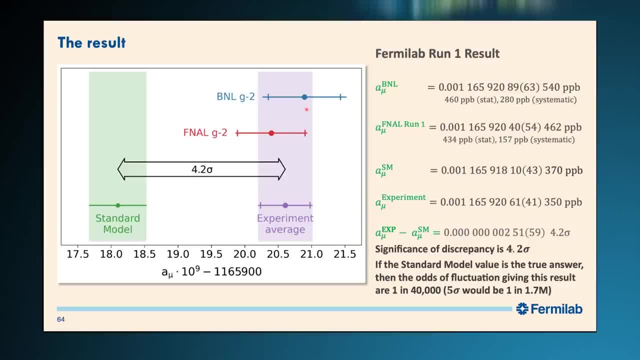 So it's like, if you're, I don't know if you're playing backgammon. if those of you who play backgammon, you know each player. when they turn they roll two dice right, And if you roll, two dice, you're going to get a lot of value, And if you roll two dice, you're going to get a lot of value. And if you roll two dice, you're going to get a lot of value. And if you roll two dice, you're. 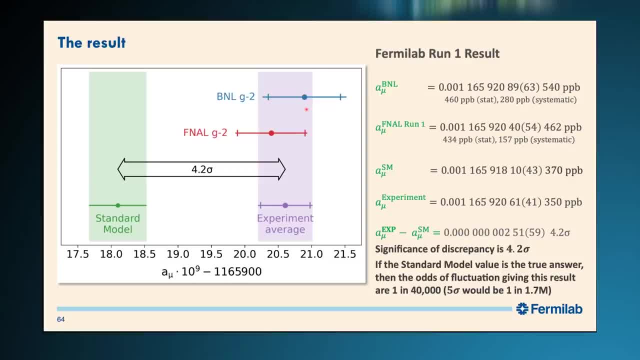 really happy because that's like the best move you can get. And sometimes when you're playing backgammon and you're playing against someone and they're doing really well and they get, like you know, two double sixes in a row, and you're like, oh, this is terrible, you're going to lose. 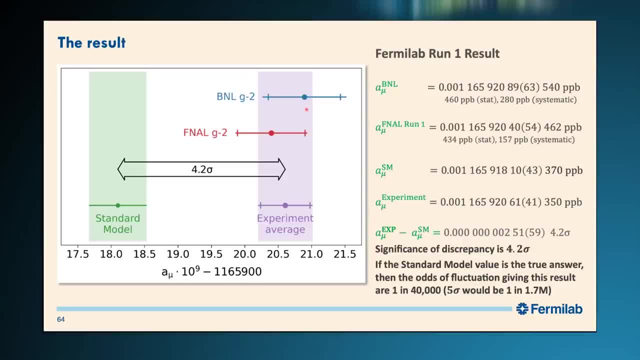 You know, and that's really unlikely. It's very unlikely to get something like two double sixes in a row, but it can happen. You know unlikely things can happen, And so you know the but the less likely it is for that to happen, then the more robust your answer is right. 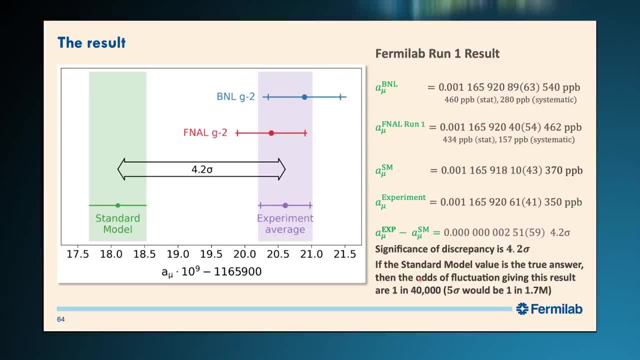 So basically a 3.7, so actually here 5.2, 4.2 sigma means that if in fact the true answer is a sterile model, then the odds are 1 in 40,000 that a statistical fluctuation could make your 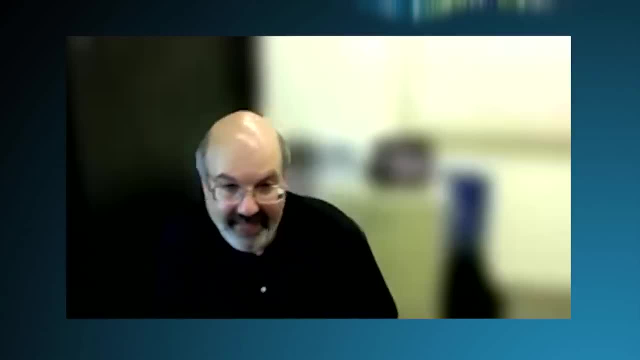 result be pushed out all the way to here. So that's becoming. you know that's quite unlikely and the odds of two double sixes are like 1 in I think 1,200 or something. Yeah, I think 1,200. 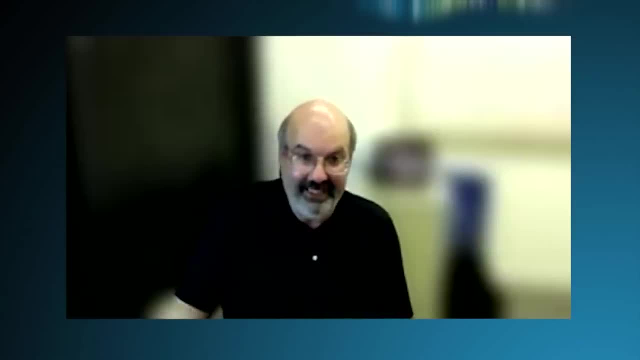 or 1,300 or something like that, So a lot less likely than the odds of getting two double sixes in backgammon. But if this were 5 sigma then the odds would be 1 in 1.7 million. And at that point we say: you know that really. 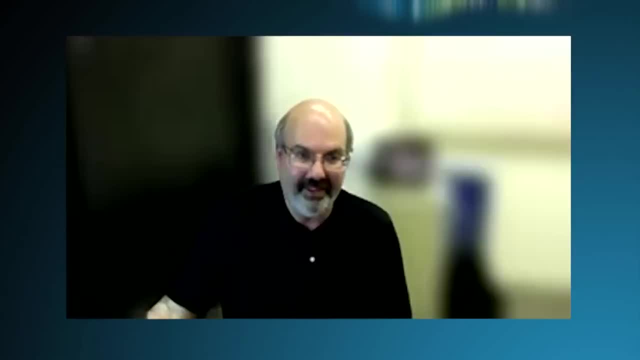 that's so unlikely, that then this result is very, very robust. So the closer you get to 5 sigma, the more robust you get. So we're getting. you know we're better than 3.7, so we're getting. 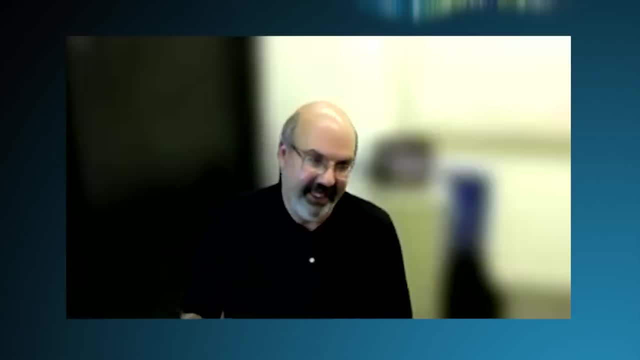 more robust, But that 5 sigma really is that gold standard that we want to meet, And that's when everyone takes this seriously as a discovery. And so the Higgs had to be above 5 sigma. the top quadrant that was discovered. that had to be above 5 sigma, And we're keeping. 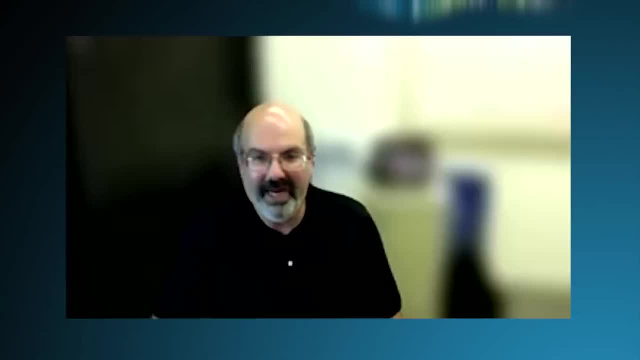 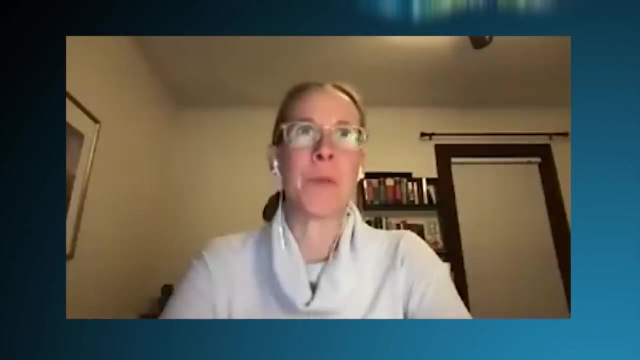 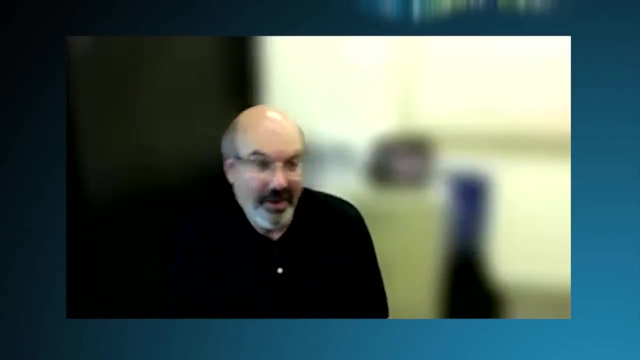 with that tradition, because that works, Because 1 out of 1.7 million, that's really rare, Very, very unlikely that that would happen. So sorry, Thanks. So time for one last question. Thanks, So thinking decades ahead. um, where could this new discovery lead decades ahead? okay, um so so hopefully, uh. 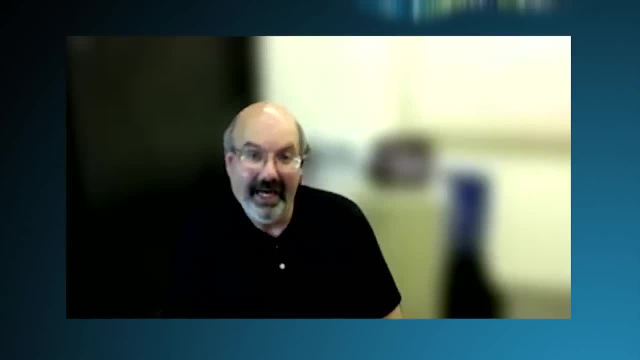 in the next three or four years, uh g minus, or you know. our experiment will be done, um, and we will you know if things go the way they're going. this is a prediction, right. we don't know this is going to happen, but you know we will probably get a result which is much greater than five sigma. 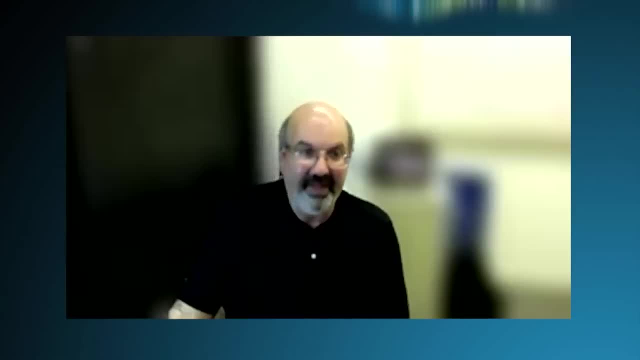 you know, assuming this error model stays where it is, maybe moves around a little bit, because this lattice, these lattice results. we'll have to see what that happens, but uh, but maybe we get a, a result that that's greater than than five sigma, and that would be great and, as i said, you know, 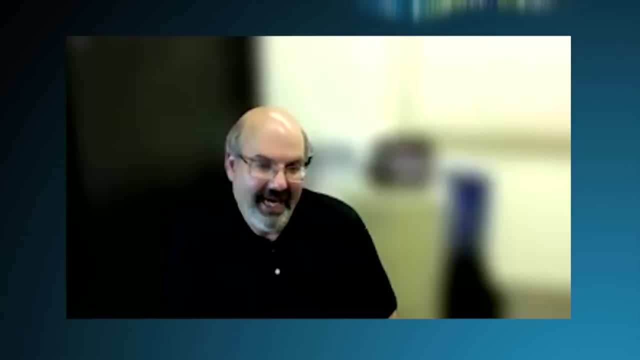 even with that, uh, you know, we alone can't really say what the new physics is. but hopefully, decades from now, um, you know the lhc will have run. you know we, you know they're, they will be in the position to hopefully see something new. uh, if, if it's it was, if it's within their reach. right there, there are things within their maybe. 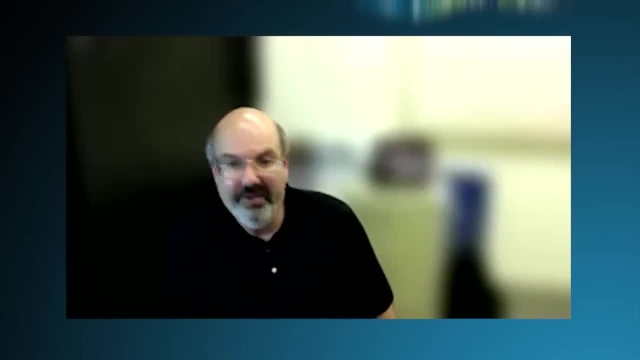 within their reach, or maybe not, and so we have to see what they see. uh, we're doing another experiment here called muti, which will be turning on probably in a few years. uh, and they're going to look for a very, very, very, very rare decay of the muon, something like at a rate of of 10 to the 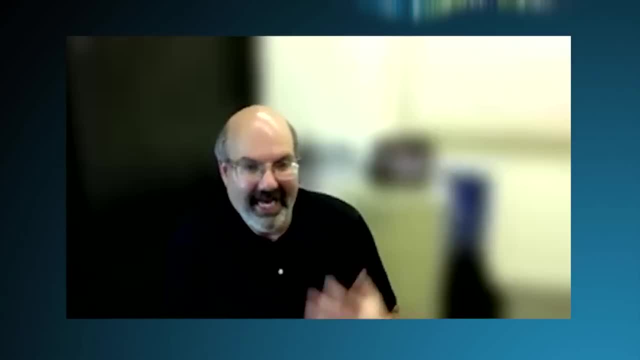 minus 50, uh, and so if they see something that's a big discrepancy with the standard model, uh, if they measure something above that, and so that again would wouldn't, that would narrow down the spotlight right as as to what, uh, what we see, uh, what part, what models there could be, and you know, 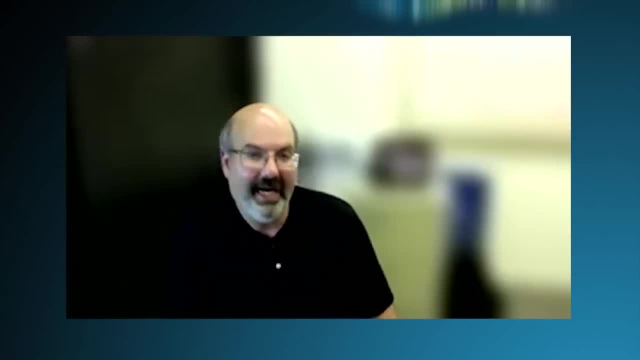 we have these big neutrino experiments, uh, that are going on, uh, and they're you know, they're looking for things like what's called cp violation and understanding, uh, how neutrinos work, to even greater detail, uh. and so you know, this is all you know. this all gets put together right, so so you. 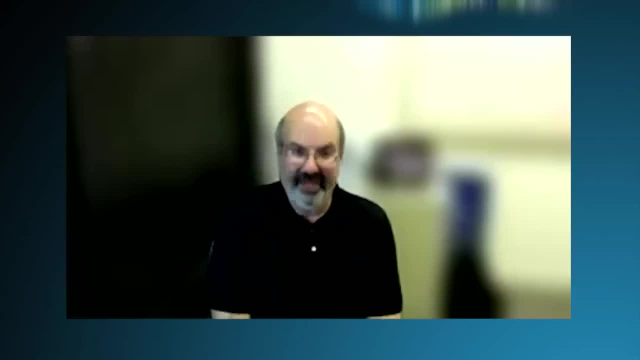 know, we we try to create with all these experiments? uh, try to create a picture, a hopefully consistent picture, and it might not be for a while. this is how science goes right. it takes a while to uh, for things to sort of merge into into an answer. uh, you know, and it might take decades to do that. but 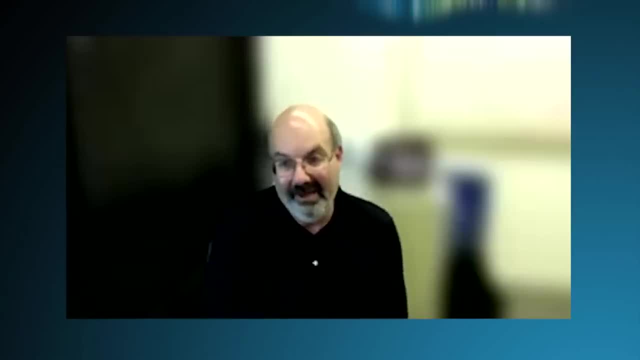 we're putting together. we have pieces that we're putting together and hopefully we can do more powerful experiments in the future. you know, based on what previous experiments see or don't see, uh, that will guide us, you know, along this journey to understanding you know more about, about nature and the universe. 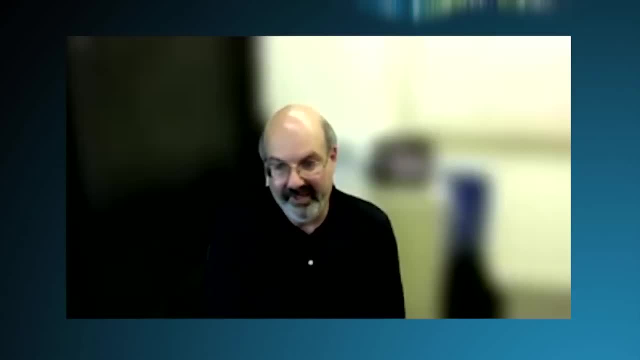 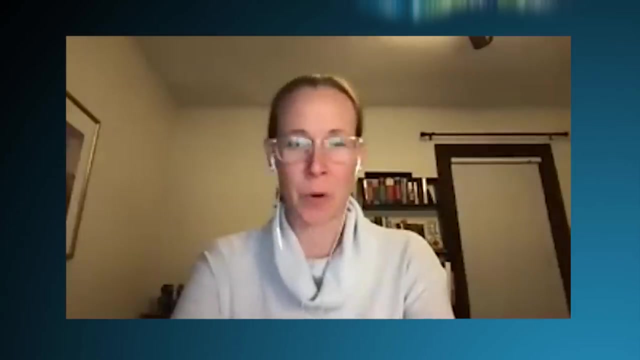 that that's really ultimately what we want to do, uh, and maybe along the direction of what this bigger theory is, that the steering model we think lives inside. there you go, awesome. thank you so so much. um, and for those of you that did not have your questions answered, or those that are interested,